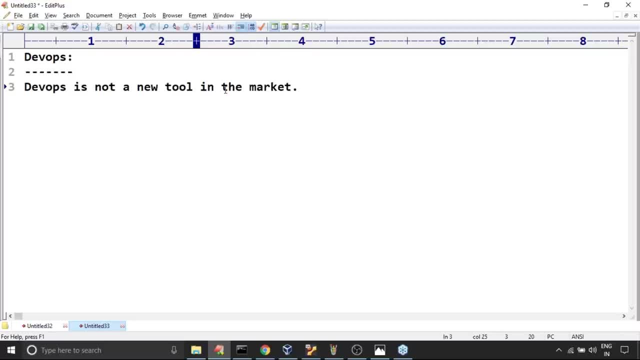 remember carefully, sir, it is a Martin: new tool are new technology in the market. okay, it is not. well, new tool, it is not a new technology in the market. okay, then what happens next? and actually, the devops such. okay, it is not a tool, it is not a technology. what is that? it is a culture. what we 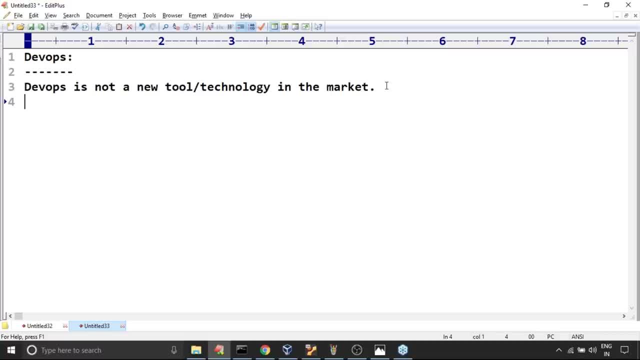 have to follow. it is a new process. what we have to follow. okay, like it is, it is a new culture. okay, it is a new culture. our process, sir, it is a new culture. what we have to follow, or it is a new process, what we have to follow: to develop, to develop, release, release, to develop release. 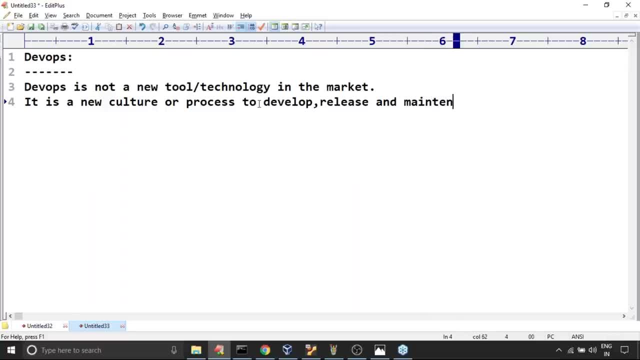 under maintenance, under maintenance, maintenance or software product: okay. maintenance or software application or project or product: okay, like a software product, like so, if you want to develop or release or maintain a software application application, complete life cycle of software application or software project or product. so a new culture came in the market, a new process we have to follow. 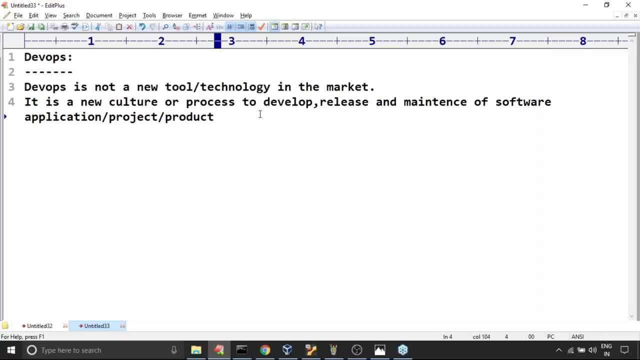 okay, like a new culture. a new culture came in the market, right. so next, with the with the higher quality, with the higher higher quality. okay, so with the high quality, i have to develop a project. okay, with the in in faster way, in very faster way. okay, like a within. 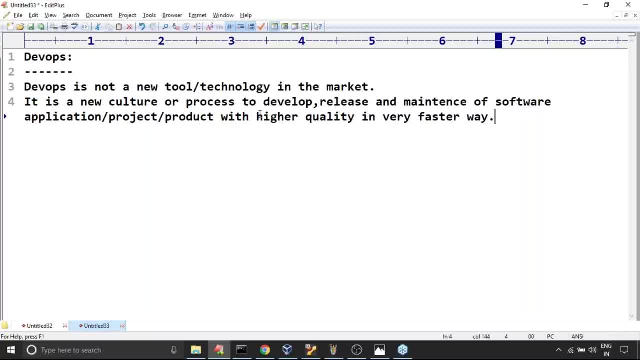 very less time. only i have to do that. okay. so if you want to develop your project, if you want to maintain your project with the high quality and faster way, the best process. a new culture came in the market, or a new process came in the market. okay, that culture or process itself is 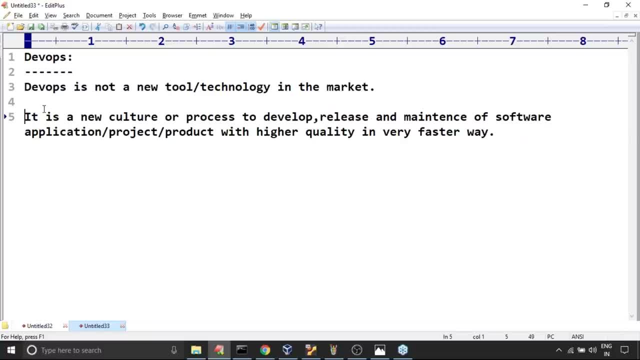 nothing, but they were everyone in the position to understand. yes, friends. so so don't feel it's a technology, don't feel it's a tool. don't feel it's a tool, don't feel it's a technology, it is a culture or process. okay to develop, release, maintenance of software application with the 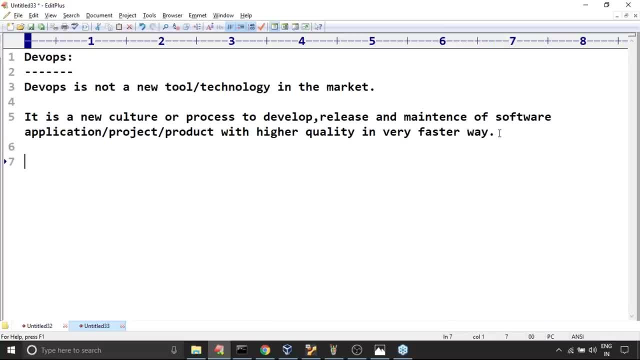 higher quality in very faster way. okay, like. so the beauty of devops is we can achieve. we can achieve by using automation tools. remember this one, sir: by using automation tools. okay, let's see what it is. okay, so we can. we can use a device. okay, so, we can use a device. okay, but let's. 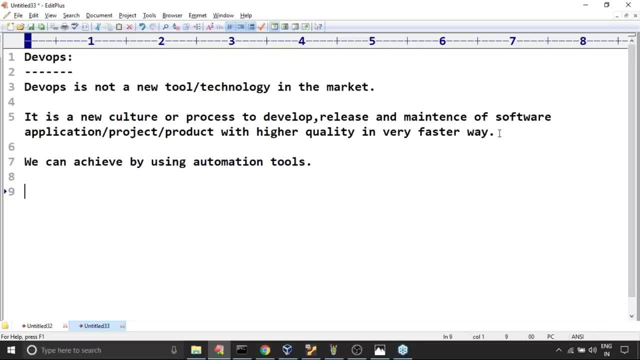 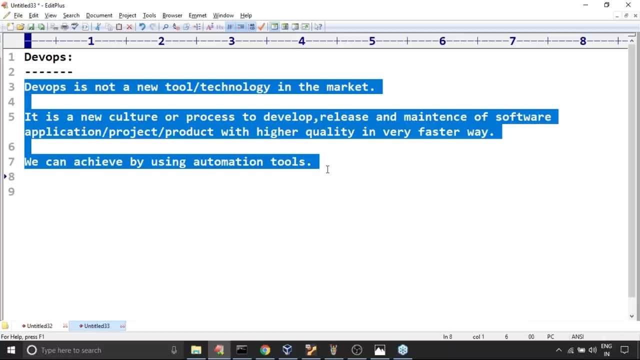 like, sir, what is automation tool? okay, all these. which tools are there? these part i will discuss. okay, just a basic idea what you people should aware. sir, dev apps is not a new tool. dev apps is not a new technology. dev apps is a culture. we have to follow our process. we have to follow. 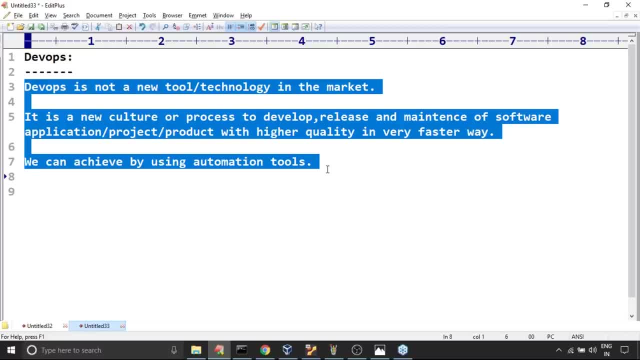 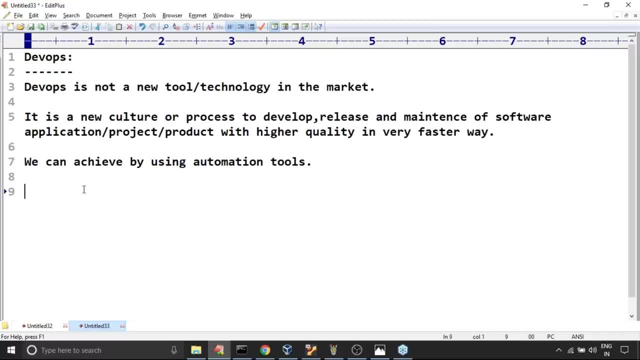 to develop projects with high quality and in shorter time. such type of thing, such type of new culture or new process, itself is nothing but dev apps. any doubt up to this, please confirm. are you in the position to understand the words? words right, okay, well, next. uh, sir, in for any software. 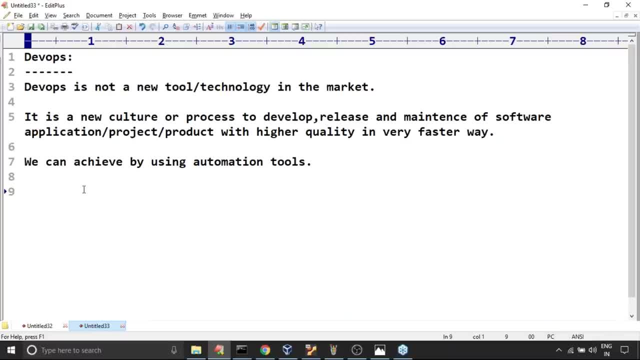 development, in the, in the organization, sir, for any software development and maintenance, for any software project, there are two types of two types of two groups of engineers are working, sir, okay, for any, for any software, for any software software product, for any software product, two types of two types. 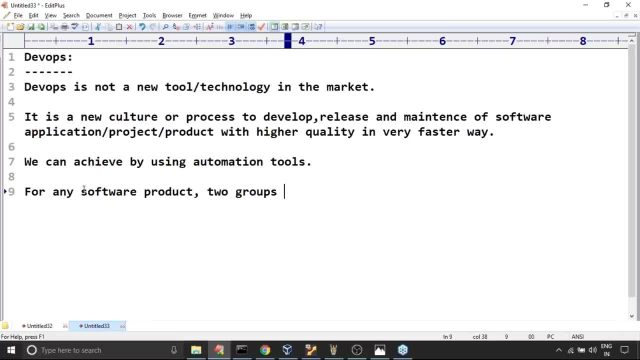 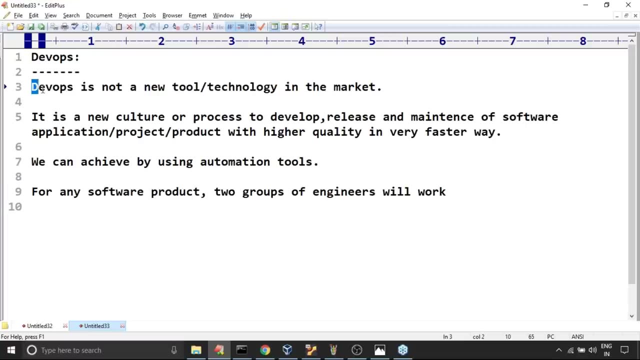 of engineers. two groups of engineers will work together. remember this: two groups of engineers, engineers are required. our engineers will work, sir. okay, will work, will work. so for any software products have you heard about, sir? have you have you observed right? the first one is a development group. what is the first one? 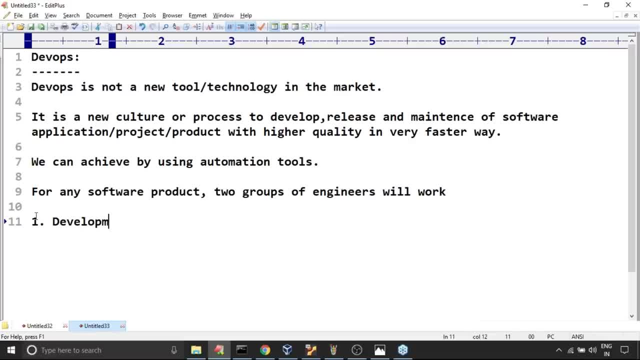 sir, can you please spell out where you respond? what is the first one? development group? development group is the first one. second one, sir, development group. second one is, uh, sir, non-development group, which is also known as operations group. operations group. these people are considered as operations group, sir, non-development group, non-development group, non-development group. okay, or sometimes. 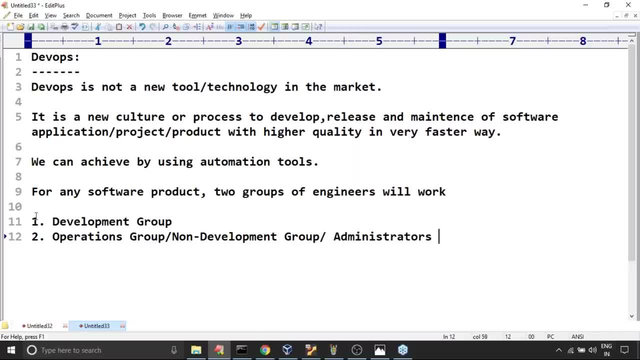 we can use administrators group, administrators group, okay, like we can use the word. so if you want to understand the dev apps first, you should give a these two groups, okay. dev apps is nothing but development and operations, development and operations. like, sir, what is development group, what is operations group? first you should aware, then you can understand the word of devops very easily. 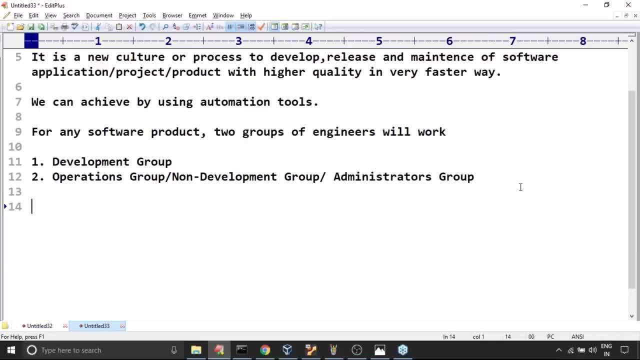 any doubt are you getting right. so what about these, sir? sir, further, there are again. this classification can be divided into, sir. within the development group, there is again coding group. is there next time after that? coding, coding, coding group. is there next time after that? do you know? 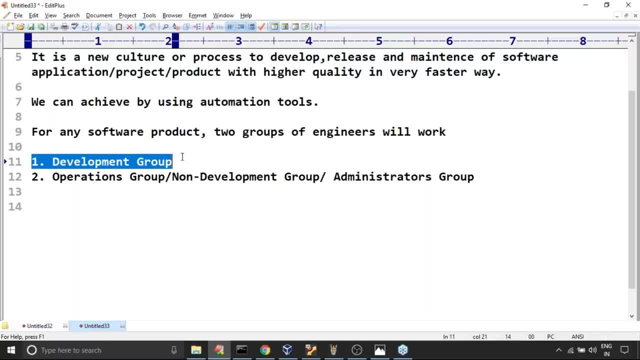 sir, what we call testing group, like multiple, multiple subgroups, are there, but anyway, our concentration is always on main, only these groups. okay, again, okay, if you want, again, again this class classification, again this classification. this classification can be divided into small set of groups, a small, small set of groups, but anyway, these are small sets of groups, we are not required. 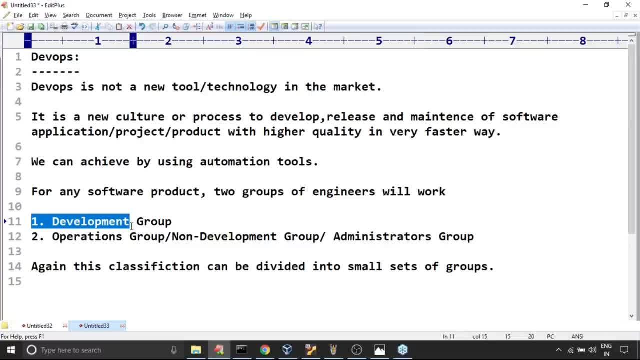 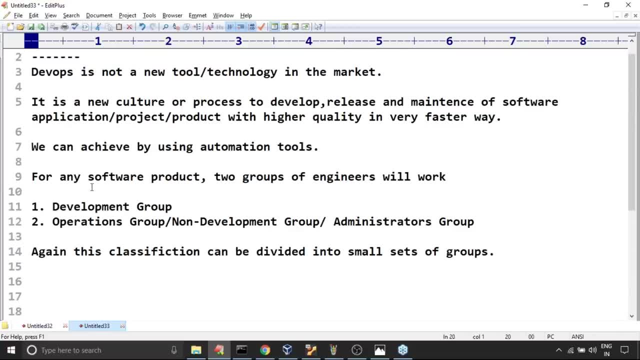 to. we are not required to worry. our concentration is always on what is the development group, what is the operations group, like you people should aware. any doubt about up to this we will discuss in detail, don't worry at all. okay, like sir, what is the development group? so to the development group. 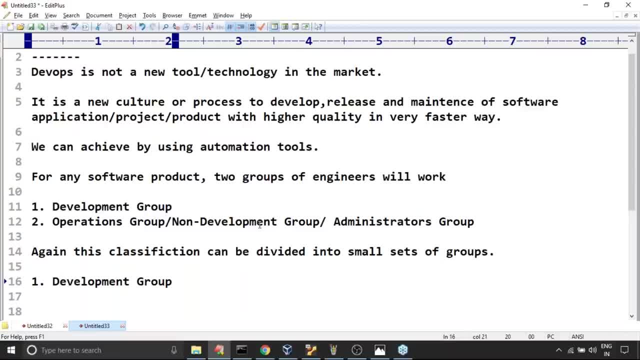 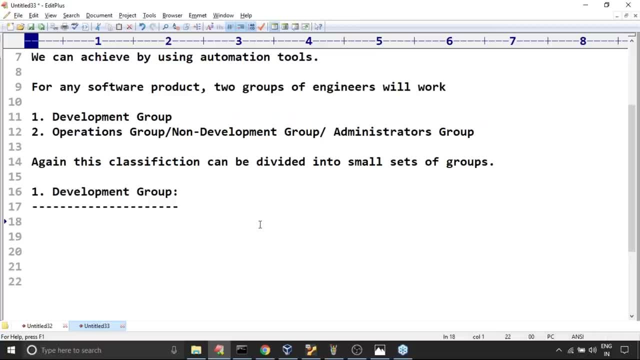 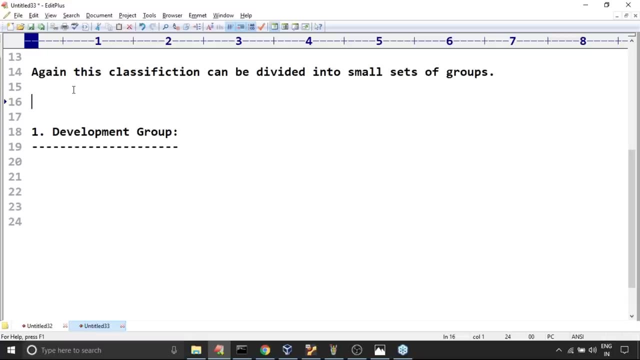 to understand devaps word first. you should have clear clarity about this. these ones are development group and operations group. so what is that? what is the development group, sir? usually, if you want to develop a project, a project sir, which persons are required? can you please confirm generally, generally? 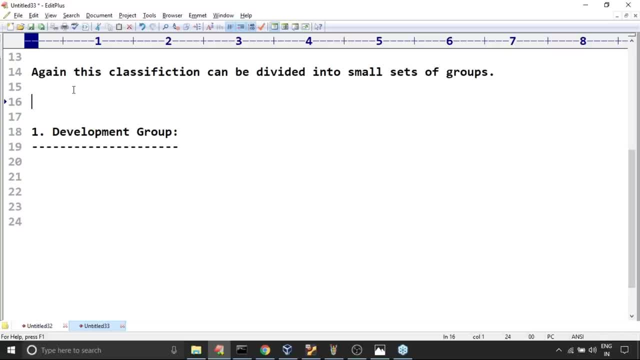 which persons are required to develop your projects? sir, i want to develop your project. which persons are required? i want to develop your project. i want to release to the client. sir, generally, which roles? yeah, excellent, developers are required. developers are required. are coders- can i use the word? 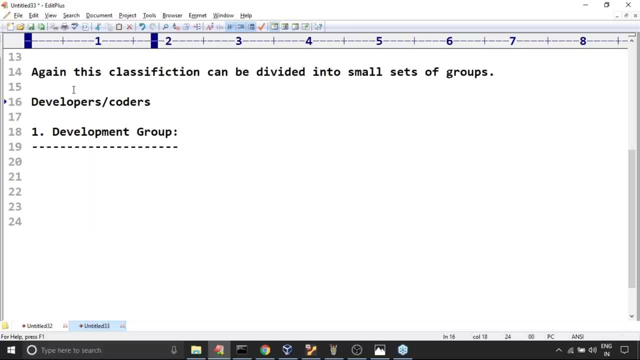 developers are coders. next and after that, do you know? business analyst must be required. remember that a bit very carefully, sir. sorry. here this person is called business analyst. one minute, one minute? okay, no problem. business analyst must be required. who is the responsible to gather requirements from the client? business analyst must be required, okay. next and after. 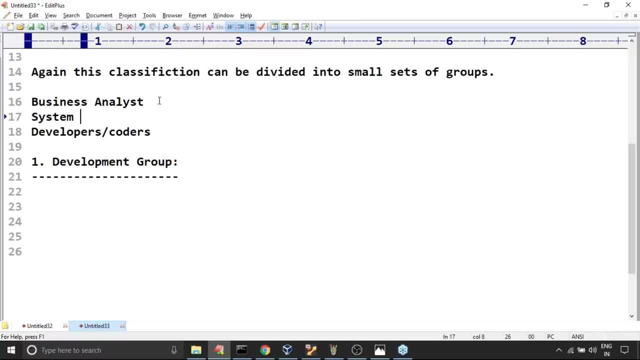 that? do you know? system and list must be required. okay, he's the responsible to analyze the requirements. whatever this business analyst got, okay, will be converted into functional requirements or specification. like he's, he's responsible to analyze system and list must be required. next, uh, design architect must be required. have you observed design, design, architecture. 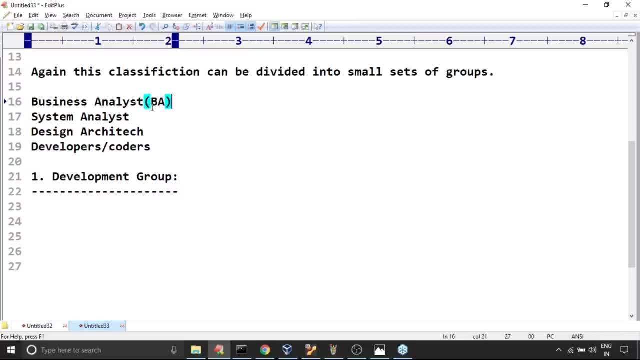 do you know this? b business analyst: shortly the people are going to use ba system and lists shortly are going to use yes here. next design, architect, design, architect, architect is required. architect d a. okay, like we can. next, developers are coders most of the times. we know we are talking about. 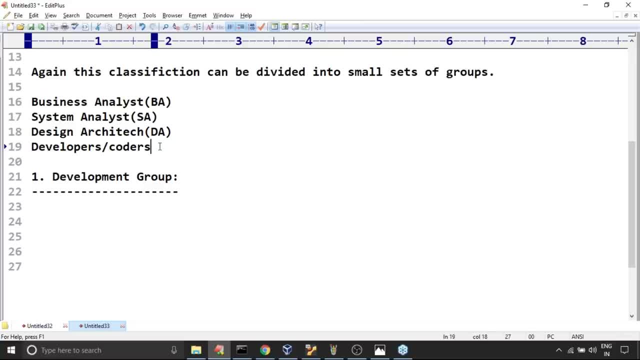 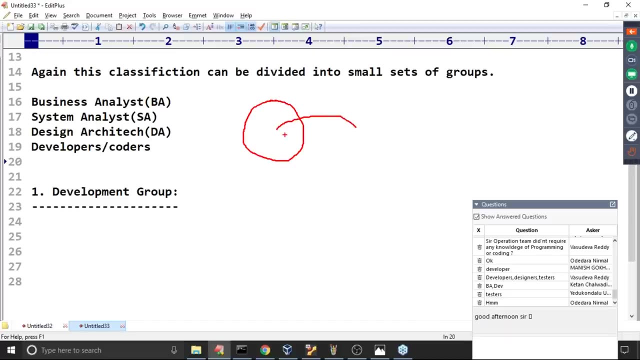 this one: developers are coders, okay, like next developer, once the developer developed the code. remember this one: once the developer developed the code, that total code we have to integrate together and we how to release, we have to convert into: okay, deliverable thing. okay, this thing is: 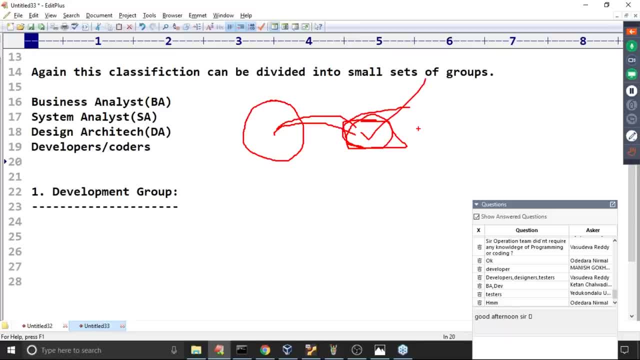 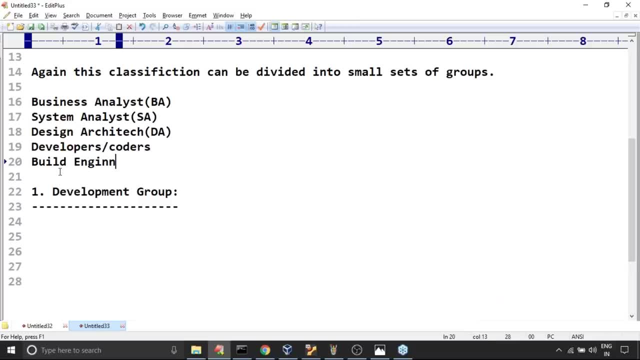 called build, build, build applications are er file, rare file, jar file, something like a build engineer is required, correct or not? bill engineer, sir. build and release engineer. somewhere you may heard about this role: build engineer. what is the meaning of this build? i will explain in detail, don't worry at all, sir. next, uh, testers are required. are not testing units? are? 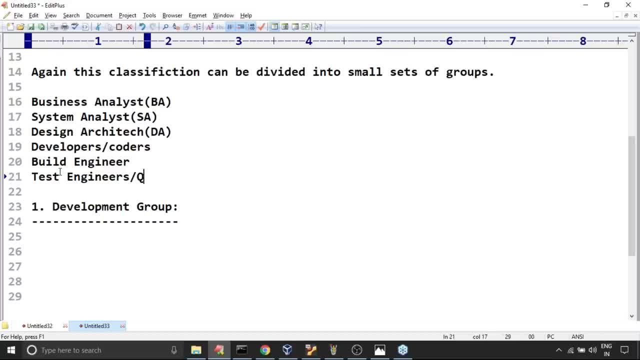 required or not? can you please spell out: test engineers are qa team is required. something like qa is required, like: so now take very, very special care about this one. all these people, either directly or indirectly, are responsible to develop a software product. okay, so these people are. belongs to which groups are development group? most of the people are going to fail. 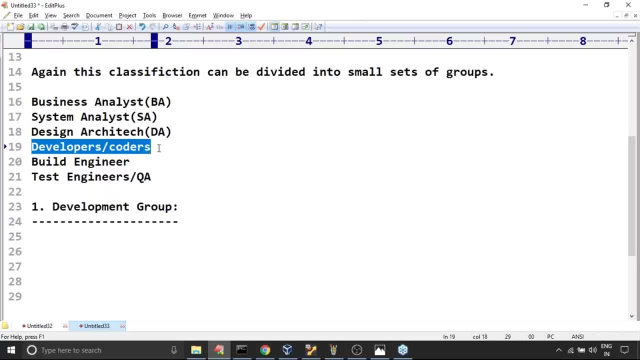 development group means developers are coders. no, no, no, okay, it is the dev team. developers are coders, are either part of development group. there are all these people who are responsible. okay, to develop, to deliver a project. such type of for this group is by default considered. 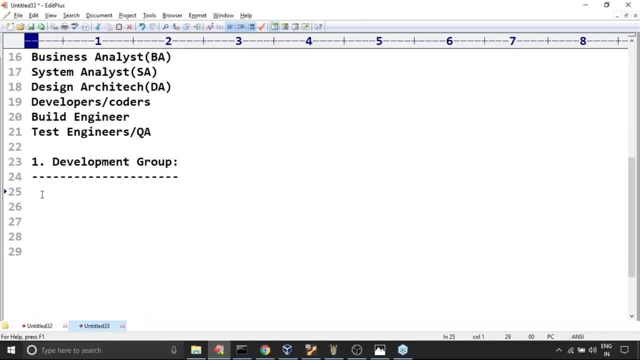 as a development group, so i can use the word. the people, okay, the people who are involving, the people who are involving- okay, involving the people who are involving- okay, just who are involving in planning. planning means: do you know? requirements, collection, requirements, analysis, design, like a planning, these all 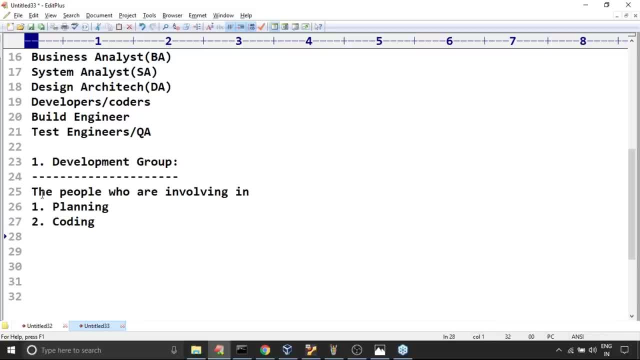 together is by default considered: planning next the coding, coding next, build, build the application next and after that, you know, testing, testing the people who are involving in these activities, who are involving these. these areas are considered. yes, are considered. yes. development development group: okay, are considered. yes, development group. remember a bit very carefully. 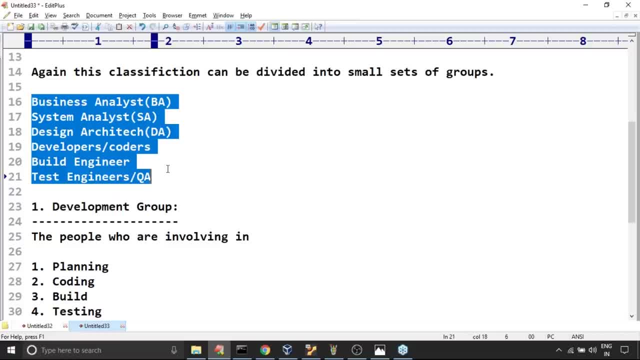 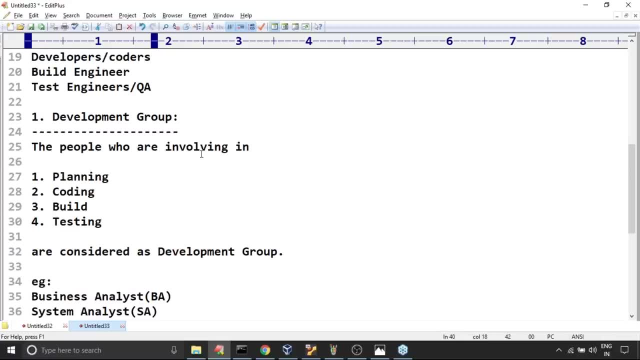 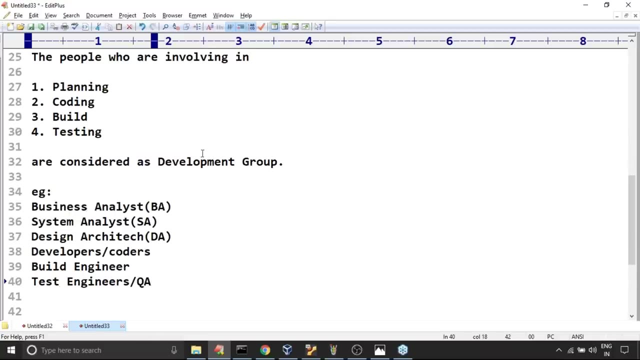 sir, so i can use the word. all these people are considered. yes, development group. only any doubt about this? yes, normal, was there ready? yes, have you observed right? okay, all these people, the people who are involving in sir planning, requirement collection, requirement analysis, requirement analysis, like a sort, like a development group? yes, development group. 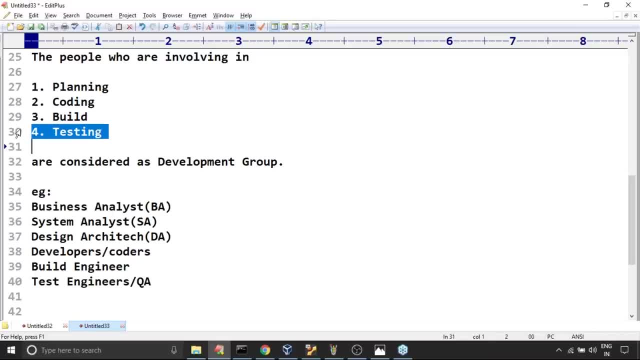 all these people, the people who are involving in the development group- yes, development group, okay. so these are the examples what you people should be aware. why build? okay. next, code plans and the build going to build testing engineering. what will be coming next? alright? next is so that building engineering is going to not be with right. first of all, several developers. 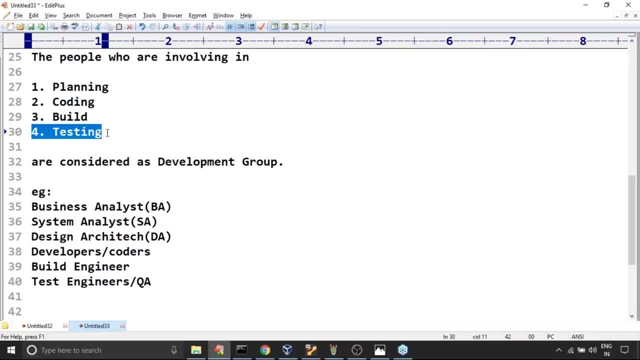 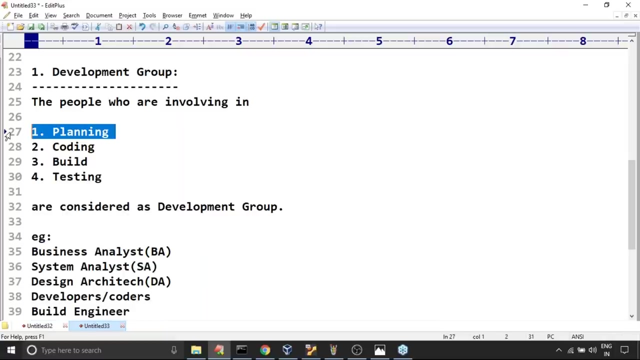 are responsible to code. okay, the total code should be integrated and converted into the builder. now that build, we have to send it to the qa team for testing purpose. yes, okay, while the concept is going on, you people will get much clarity. just observe the basic terminology. right, yes, normal, are you getting? so what? what? they are responsible, okay, so requirement gathering. 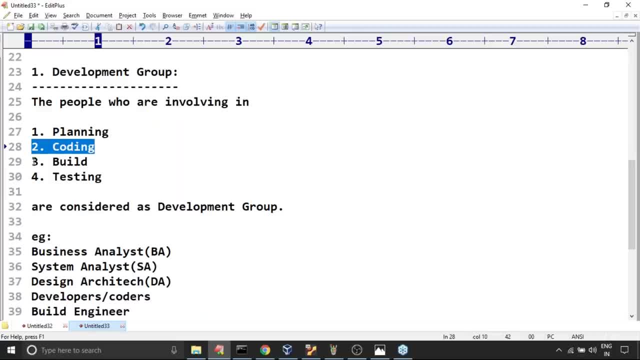 requirement analysis and the design like quarters are responsible. next, build, sir, build. we have to discuss each activity in detail. don't worry at all. there we have to talk. okay, almost it's a, it's a big course, almost around two to three months course there, all these things we are going to. 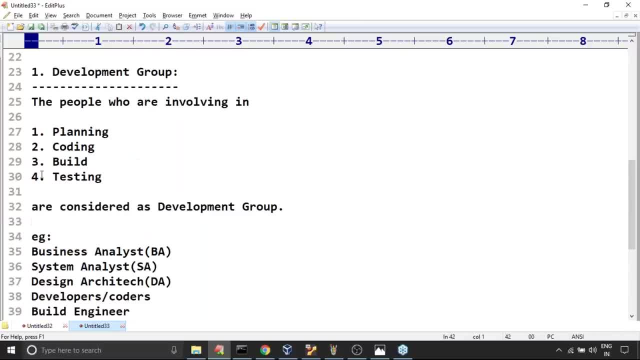 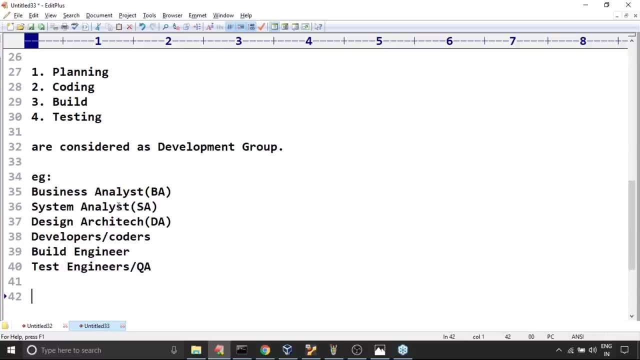 get just aware. so operation so up to this development group. not required to keep any explanation right clear. so what is the other group i forgot? what is the other groups? are i forgot? you have to tell what is the other group: operations group. remember this one operations group, okay. 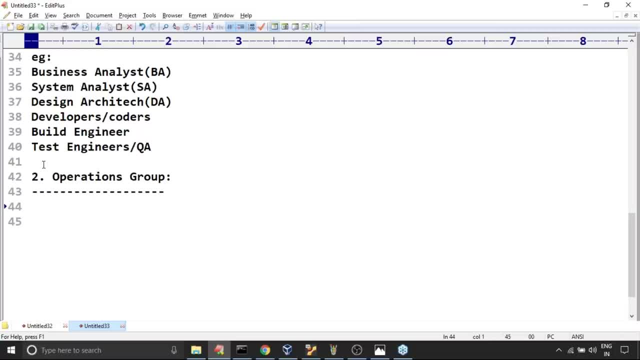 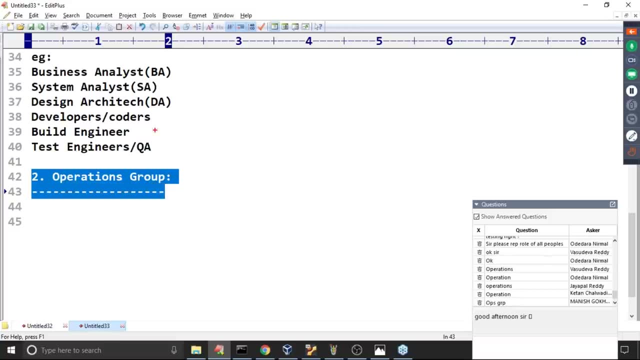 like sir. now i have one small doubt sir. okay, sir, this word you have to aware clearly very, very important, sir. sir, the project developers are okay, ready to move to the client mission. okay, legend carefully- ready to move to the client mission, development group, job completed, assume that. so, to move to the client mission, so we have to configure required software. 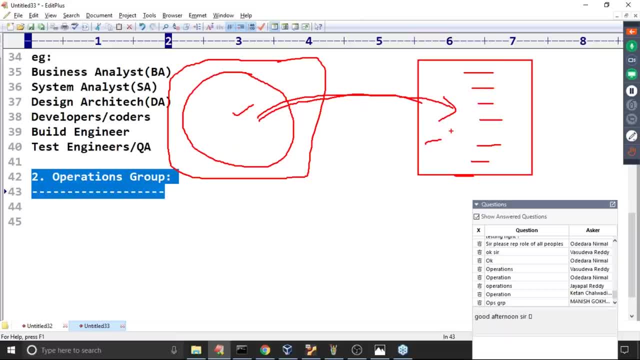 well, that's one we require. to configure required softwares are not. yes, okay. so for the configuration engineer is required. remember this one, sir: configuration engineer is required. cme means configuration engineer. don't feel okay, compile time error, okay, like next. next thing is okay. to maintain this system, system admin must be required. if it requires database, database admin must be. required. again, database admin must be required. if database Hits instance database should be required, if a database database admin must be required. regarding database, aquí será solicitado dash estudar anti-m negócio. press the database and has Gary J 및 계. Bitte, not a question now TO DI DEEC INCfare leong, small talk to you. more. most required, we require db peninsula. come here the umbrella e platen multi coworkers, yes, sir, and of course, òn f capturaro. I think it will be a question Doctor vs grandmother here. another question, Hello, how do the upper case file a data base? well, igual how you. 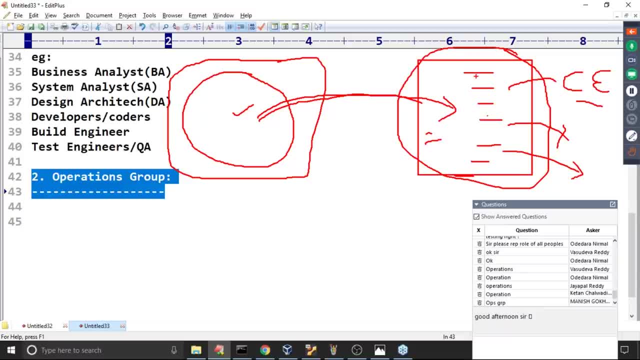 be required next. so whether applications are working properly or not, whether the system database, everything is working properly or not, monitoring team must be required. correct line monitoring monitoring team must be required. so all these people are by default considered, yeah, operations team. now you should aware. so these people nowhere related to the development, these 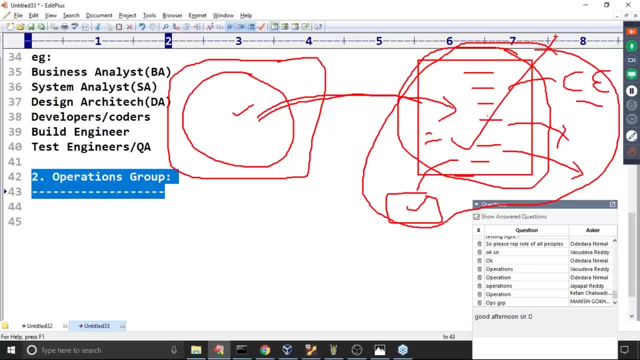 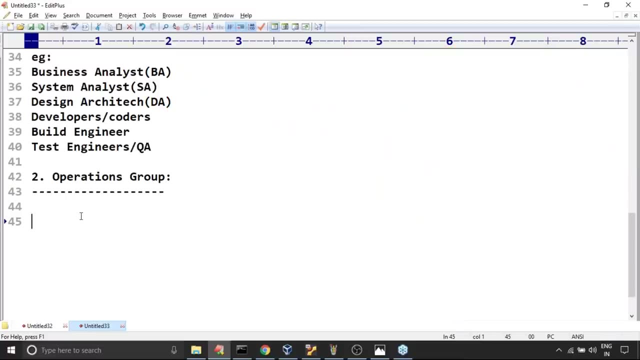 people nowhere related. the development, sir, project is ready, project is ready. we have to. we have to talk about the configurations system, management system, admin. okay, like these people are by default considered: yeah, operations group. remember a bit very, very carefully about this one. okay, like sir. now the people who are involving: okay, so here, just the people, the people who are involving. 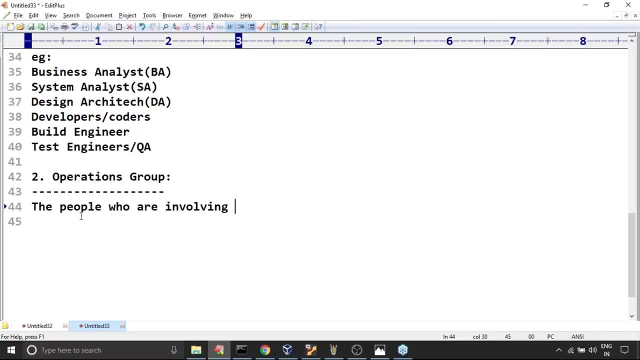 who are involving the people who are involving in, who are involving in. okay, release, okay, release release. sir, project release, sir, project project release release. okay, like project release. next, deploy, deploy deployment- we have to deploy, deploy, deployment release. next, operate operations. operate next and after that, monitor, monitor, okay, monitor. so. 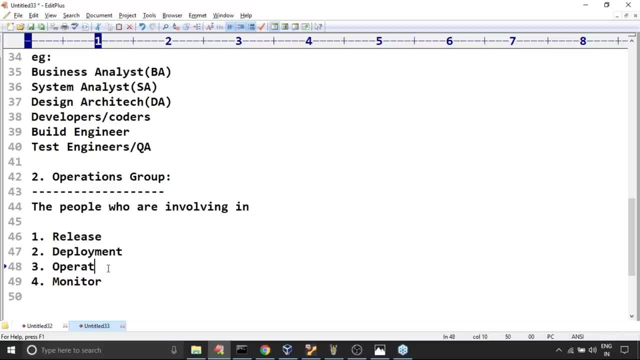 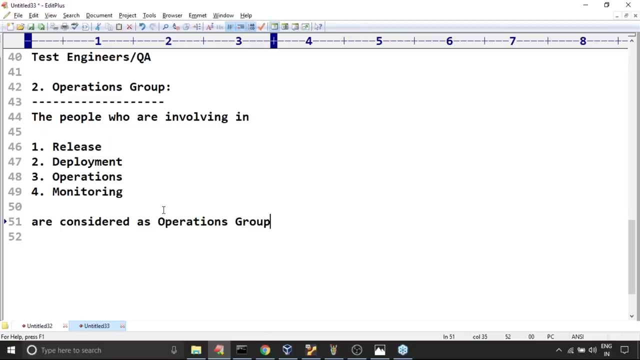 release, deployment, deployment, operations, okay, just operate. operate means operations, network, engineer, system, admin, like a monitoring, like the people who are involving in these, in these are considered. yes, are considered. yeah, operations group- remember this a bit very carefully, sir. operations group: so after project development, project, the complete development. 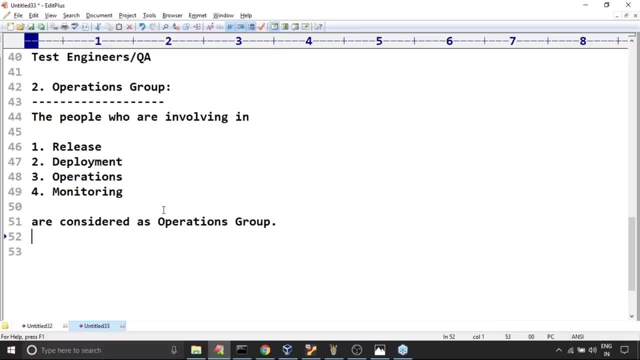 then the operations team will come in the picture. remember this one, sir. okay, like, can you please give example example for this? yes, respond: can you please give an example for this? yes, friends, so can you please give an example? configuration engineer. configuration engineer next, uh, can i use? 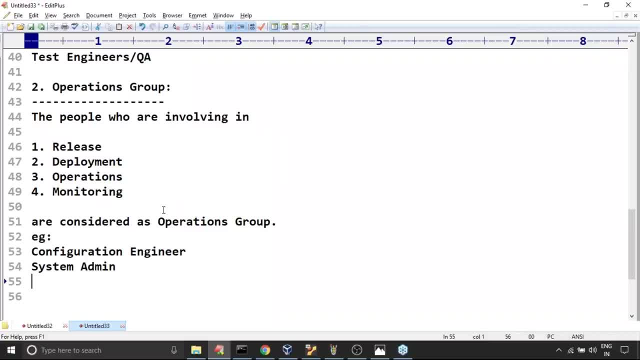 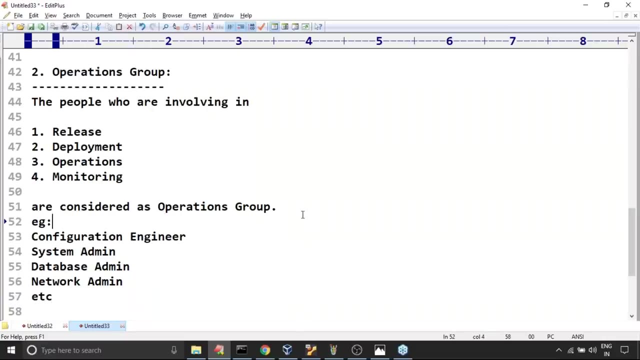 the word system, admin system admin system administrator database admin database database admin database admin, network admin: okay, network network admin. network admin admin- okay like. network admin admin like, etc. all these people are by default considered yes, operations team. remember, remember this a bit very, very carefully, sir. release engineers like release release engineers, okay, release engineers like all these. 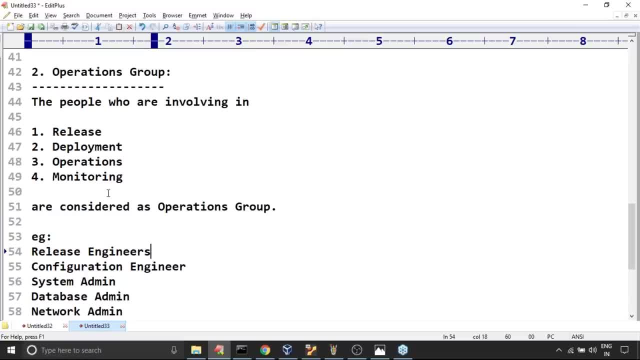 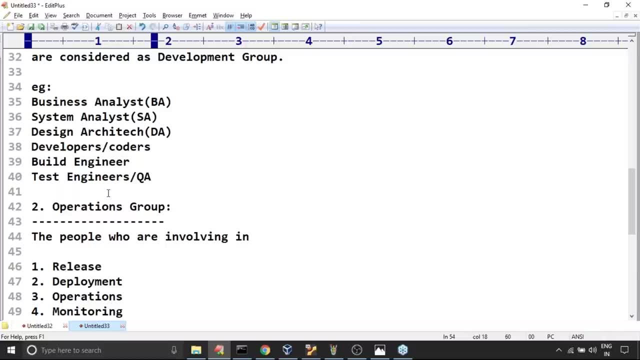 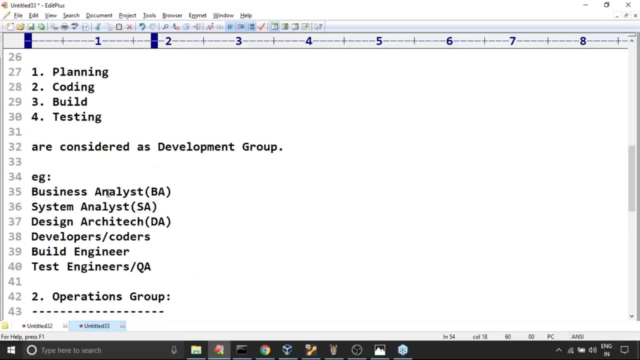 people are by default considered: yeah, operations group, operations group. but all the almost whatever we are going to discuss every day, we have to talk about these words. there you will get much clarity even at this stage. a bit abstract, don't worry at all. okay, like sir, now total. 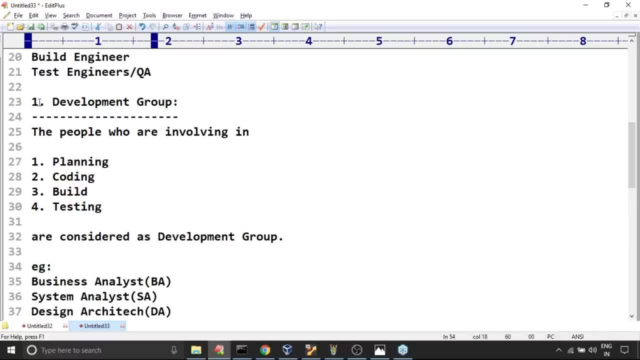 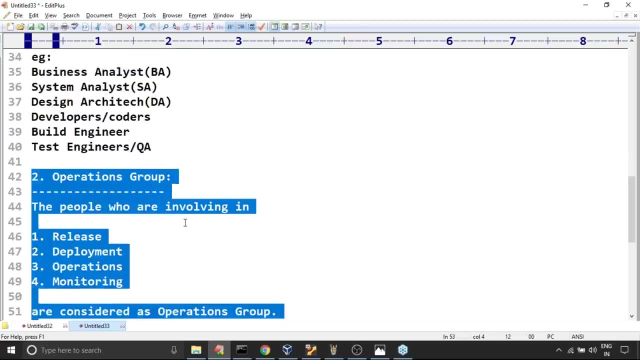 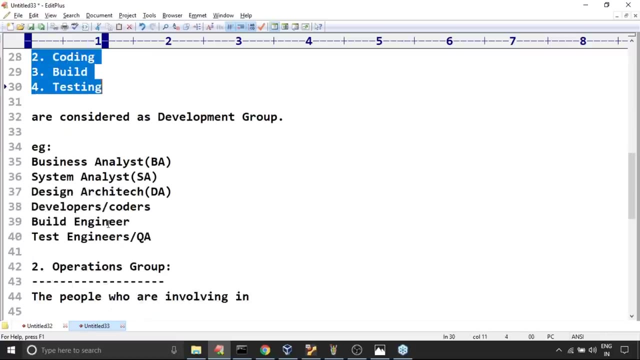 okay, total project project life cycle. there are two types of teams are going to involve. one is development group, the second one is operations group. okay, like so, development group is the responsible to involve in the planning, coding, build and testing. so once the development got completed, now operations team is going to start in the picture they are responsible to release. 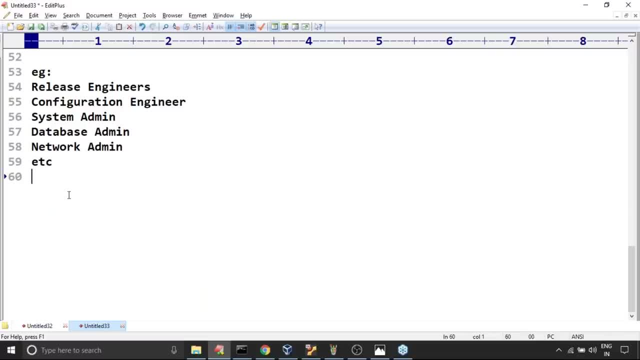 deploy operations under monitoring, like sir. now basic idea you people should got, i hope, correct right. yes, friend, are you in the position to understand the basic idea? what is the development group and what is the operations group? sir, dev apps is a combination, a combination of development, development and operations. dev apps is a combination of development and operations. 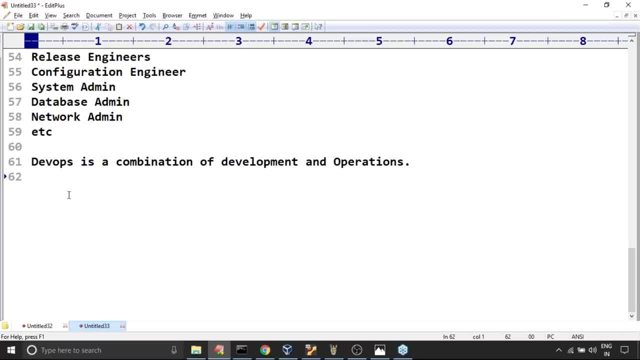 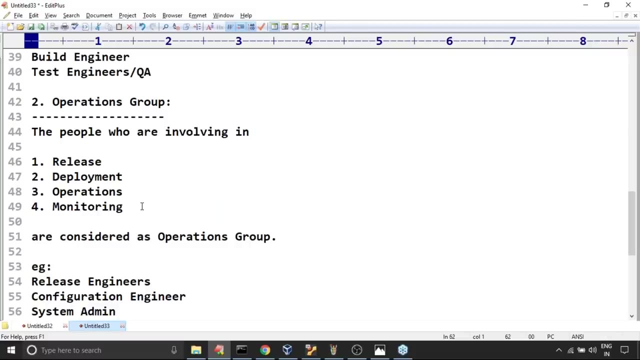 right, remember this one. so do you know? so the main objective of the devops is to establish, to implement collaboration between these two teams to deliver, okay, the project within the last time, within the last time, with the high quality. remember a bit very, very carefully, sir, the main. 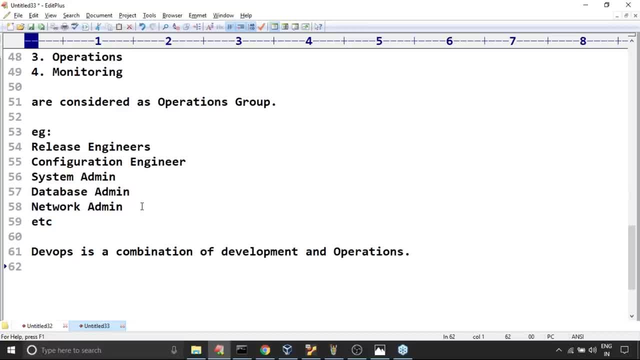 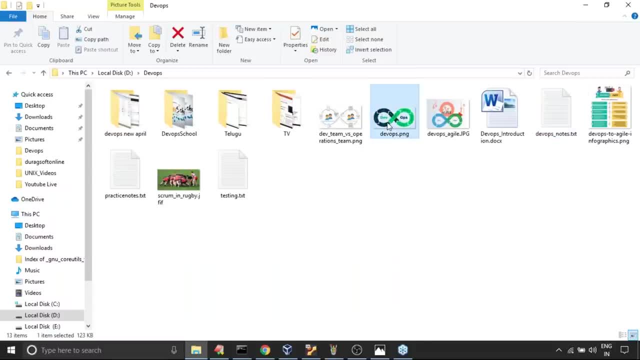 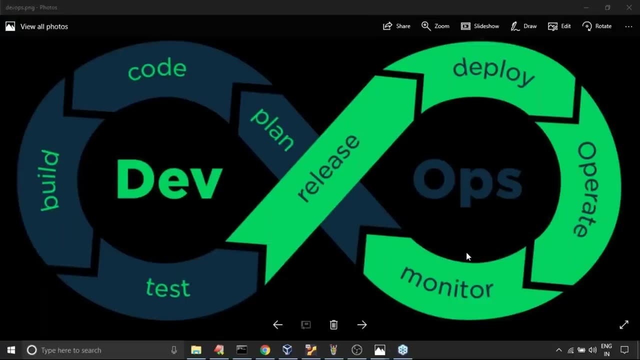 objective of devops is to establish, to establish collaboration between these two teams. and now, if you observed that i have one diagram, is there? okay, now, i hope this is the logo of the device. okay, now observe, are you seeing? is there any different, different thing here? can you please observe that here? have a available. 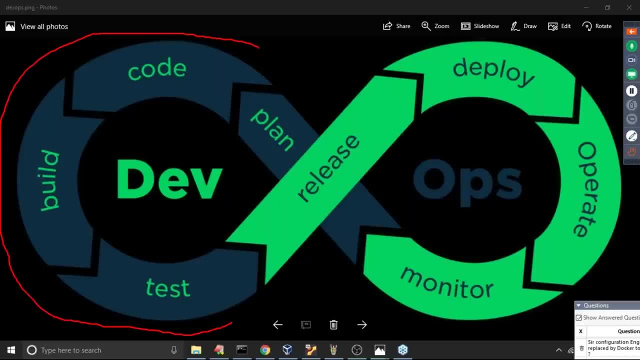 one, sir, these part is called a development part. okay, this is plan, plan, code, build and then test. okay, they are responsible for planning, coding, building and then test release. so, operations part: release, deploy, operate, monitor, like these partings by default considered: yes, okay, operations, now to s. 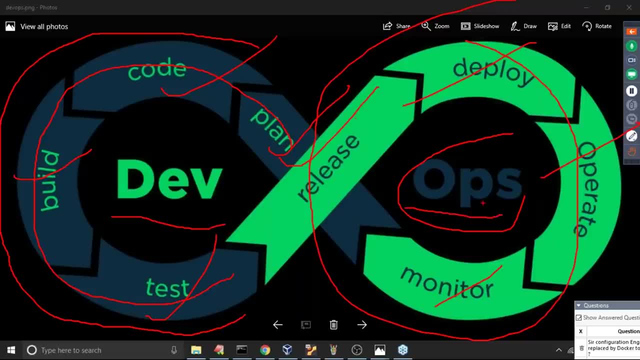 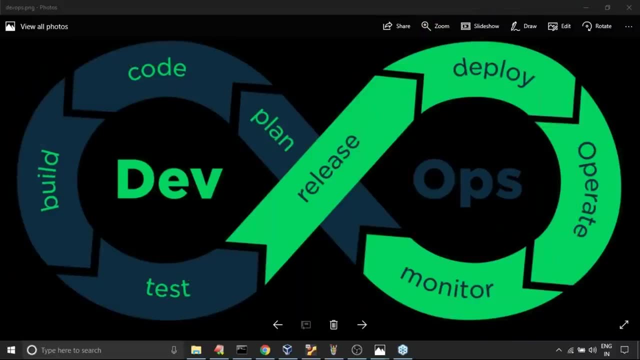 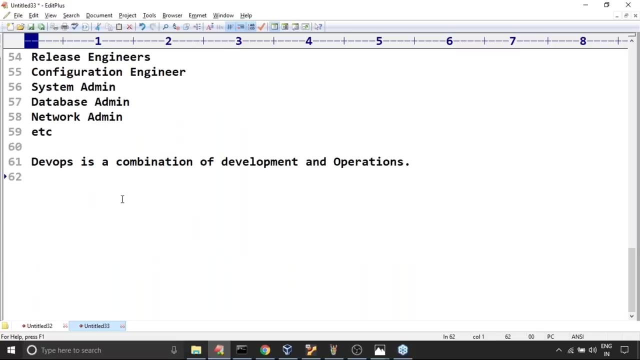 establish or to implement the collaboration between these two people as a single team to deliver and monitor the things effectively, which is this new type of culture? itself is nothing but okay. dev apps: are you in the position to understand? yes, friends, okay, which tools are required? those tools we are going to discuss in detail as of now. don't worry about the tools, just. 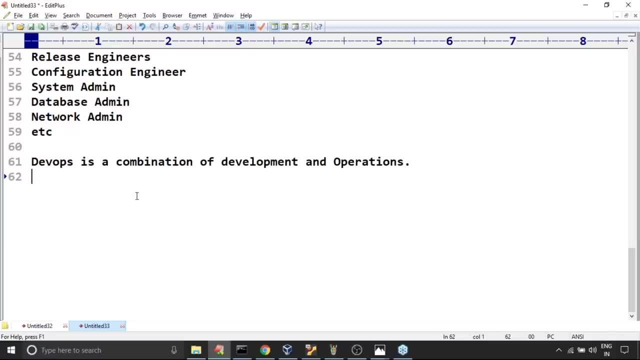 aware the basic terminology you have to understand, right? so the main objective, the main objective of devops, the main objective of devops, devops is to implement, okay, to implement, implement collaboration, to implement a collaboration between collaboration between development and operation teams development, okay, development under operation teams development. 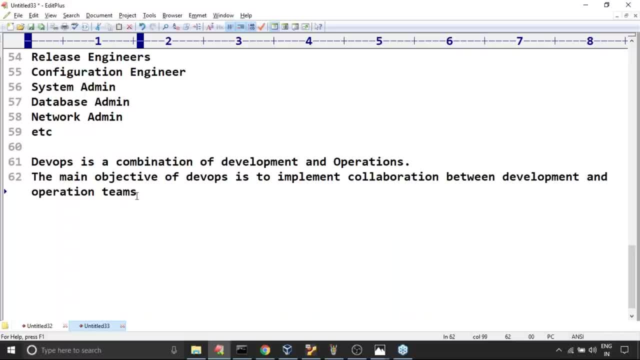 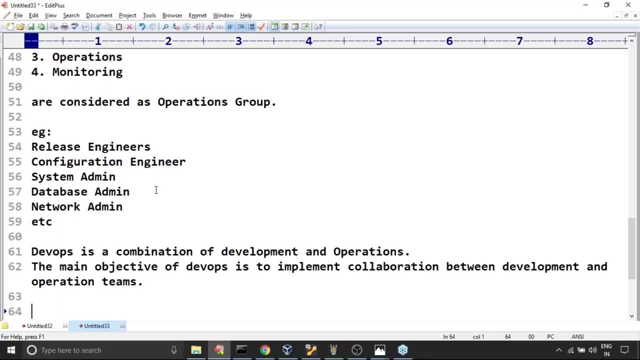 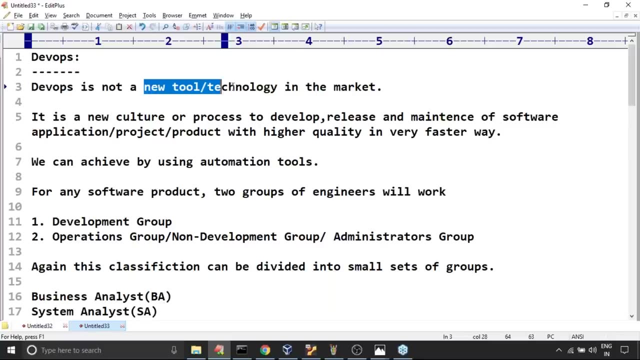 and operation: okay, operation teams to fulfill our requirement. that's also. this is what is the dev apps, sir. what is the meaning of development? what is about operations? right? so up to this, i hope it's very clear for you people, right? so it is not a new tool, it is not a new technology in the market. 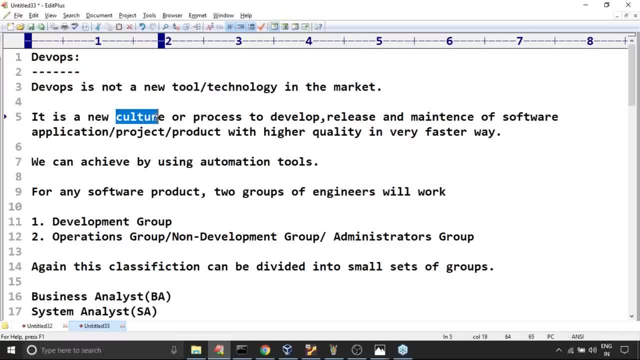 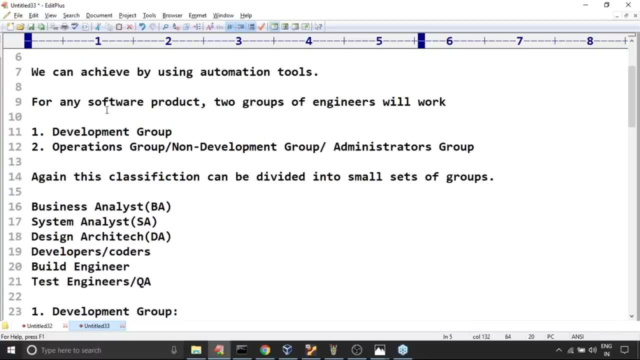 it is a new culture, new process. we have to adapt to develop, release and maintenance of software products with higher quality in faster way. okay, like how you can do that. there are multiple automation tools we are going to use. okay, like multiple automation tools we are going to use. okay, like next. uh, sir, what is the devil? what is the? 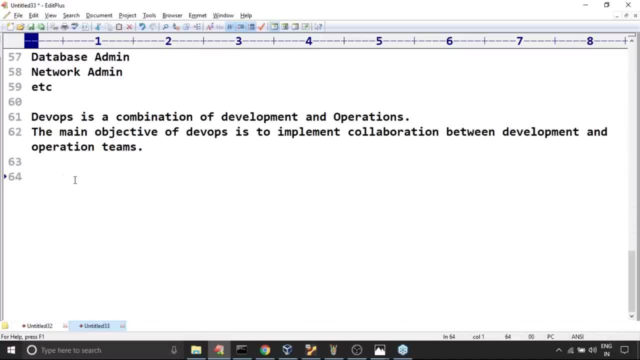 meaning of apps. okay now, basic idea. i hope you got up to this. clear, friends. okay, don't think too much about this. okay, just the basic overall idea because the total course we have to talk about these words only. okay, what's already told. don't worry about sir. configuration engineer will be replaced by docker tool in dev apps like. 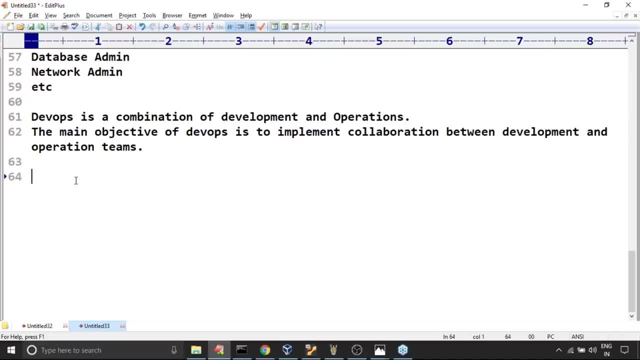 so don't worry about tools. this is not correct time. we will discuss all these things in detail, okay, now. so this is what what you people should aware, right, sir? now i have one small thing: is there, sir, to understand the beauty of this new culture, okay, we have to aware array what are various. 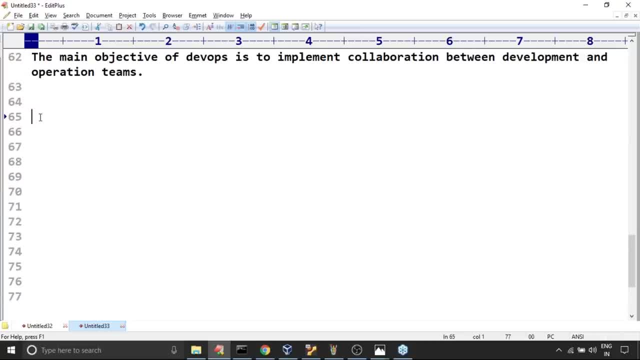 existing software development models. okay, why we have to go for these dev apps. then you will get much closer. okay to understand. okay to understand, to understand the beauty, the beauty of our this, this new, to understand this new, new dev apps culture. have you observed the word? now i'm not using. 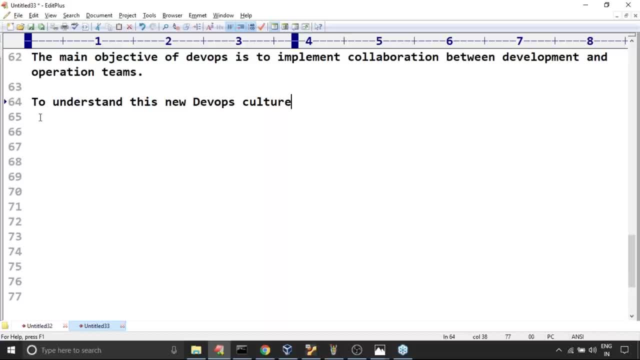 the word, the technology at all. to understand this new dev apps culture, we have to give it already existing sdlc models. remember a bit carefully, sir. we should aware already existing sdlc models. models compulsory, we should aware. okay, like sir, the first one, do you know there are several models? are there? have you heard about any? any sdlc model? 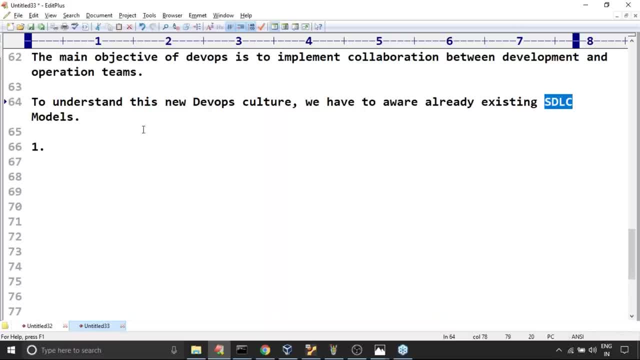 what is the meaning of sdlc, friends? why respond? what is the meaning of sdlc? okay, yeah, sdlc Schon bestimmte rechtlich inandezbehandanden sie mit den gleichordnung der reisen gak bewegt. in der beggerHoldung der kampf werke die neue geh asset artist Katrin Jaüzel. rural Qui点 ge der女er gehört. 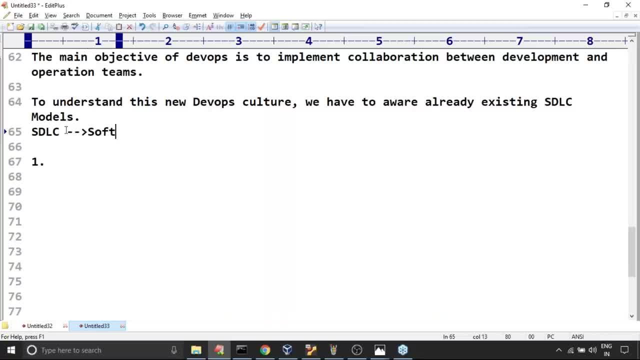 okay, yes, the LC means software, software development, software development life cycle, software development, life life cycle. ah, can you please tell what is the meaning? what is the meaning of HDLC? okay, can you spell out some software development software, SCLC models? yes, friends, please observe. sir, have you? 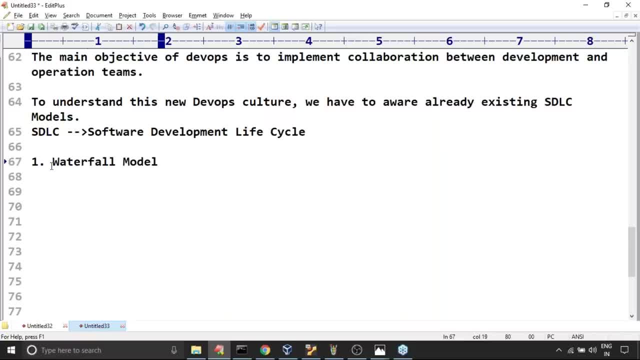 heard about waterfall model, I respond: have you heard about waterfall model from our childhood? on words, I hope you people may aware. have you heard about prototype model, prototype, prototype model. just name Sony. you are not required to very much about these. okay, even you don't know, also don't worry. 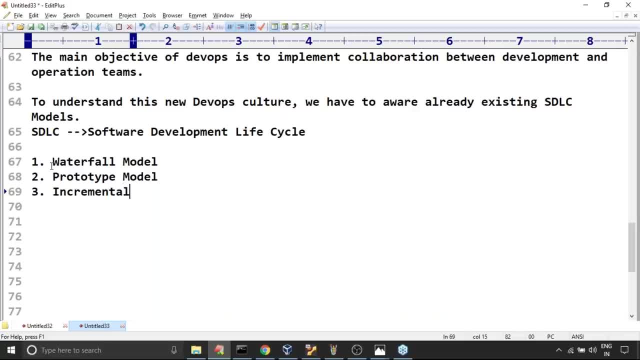 we will discuss a extra increment. incremental are iterative model. incremental are iterative model. okay, like next you may hot you born. Spirell model, spiral spiral model. okay, you may heard about red the model, red red model, rapid, rapid. okay, like next you may heard about, okay, red spiral model. 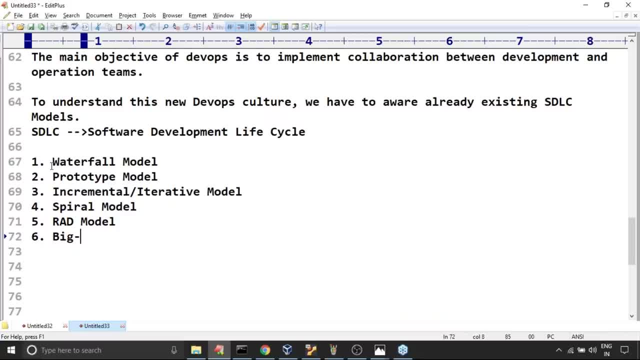 red red model next up, big bang model- okay, big bang, big bang model. okay, like next: uh, you may heard about fish model. okay, fish model. next v model v model. next agile model- okay, agile, agile model. okay, you may add, have you observed? so this is even you don't know about. 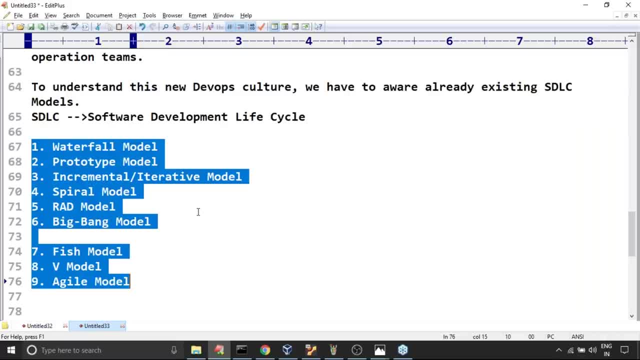 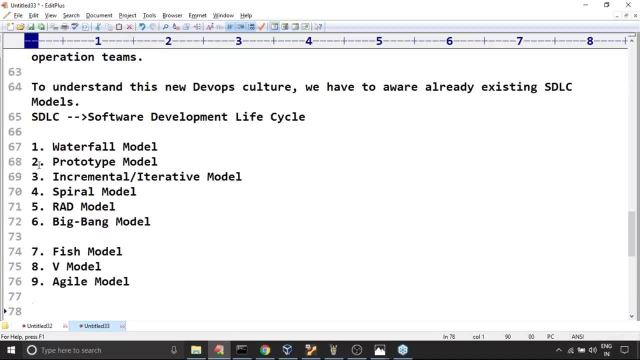 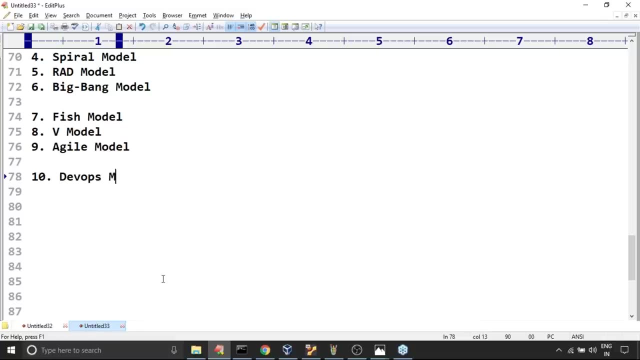 these words. don't worry, sir, i'm here to discuss, but anyway, whatever required we are going to discuss, us unnecessary, so we are not required to discuss all the things. okay, like. so if you aware these, then the beauty of devops you can aware very easily, sir. okay, devops. 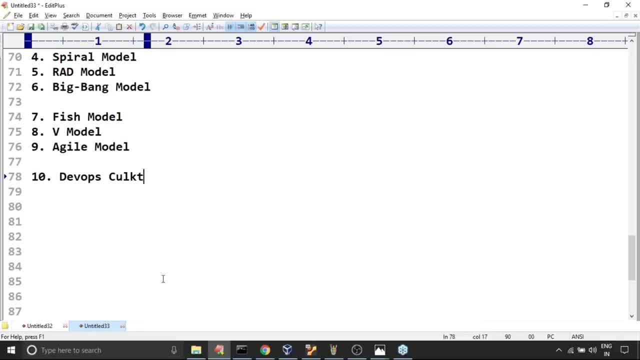 model i can use. okay, devops culture i can. i can use because it is also. it is. it is a. it is also a software development model. only it's also a software development model. only if you give it these, then you can understand the web sculpture very easily. the beauty of. 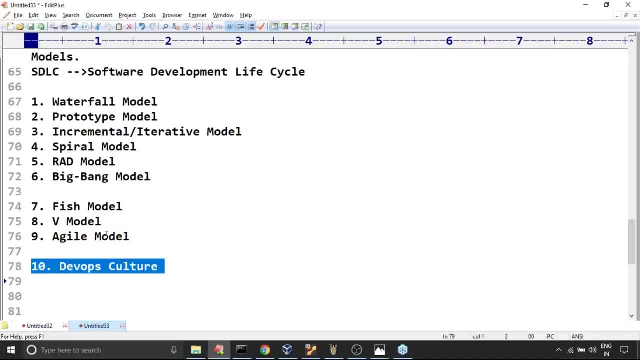 devops or why the software companies are running towards devops, then you can aware clearly, right, okay, but anyway, among these, the oldest model, waterfall models are the most recent model, i mean before devops, the most hot cake model in the market, agile model the most recent. 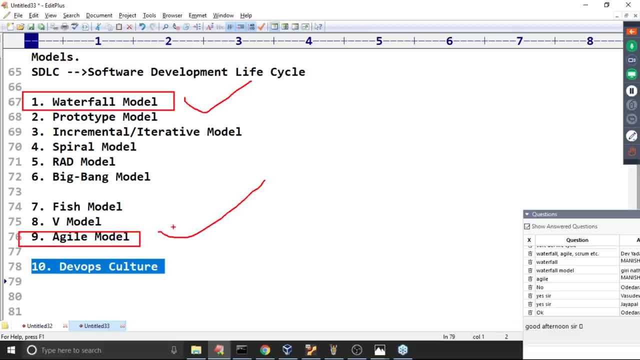 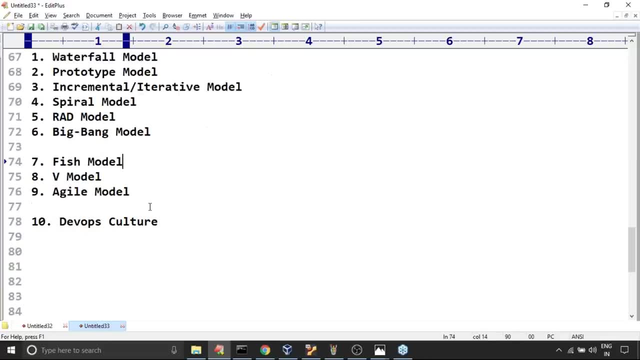 model in the market, agile model. you can learn it��. i mean, these are two things i will discuss. uh, until so, what is the need of going for devops so that you people can get much clarity? can i start this cinema? yes, friends. okay, all these models are there. earlier i handled one one. 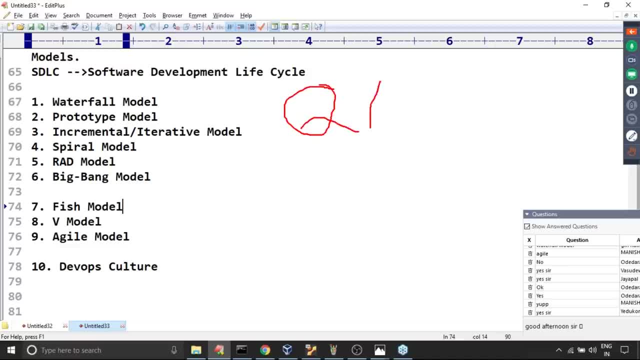 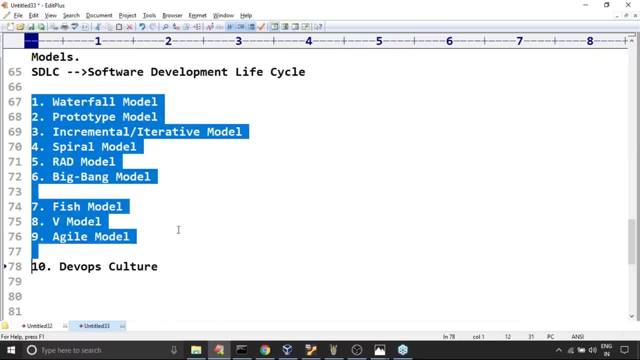 batch. okay, q j manual testing batch. i handled, sir, manual testing and selenium batches i took. i took this batch. i know all these models in detail. what is the advantage of this model? what are the limitations? okay, like i know, but anyway that are ______ alone today. i will get to the two things, okay, okay. so these are the two things i am going to ____ Canal. so three, first three, i am going to share the video and then i will share the other videos as we have more version. two first series, okay, one and two, three v, v, v, v and six v and but. 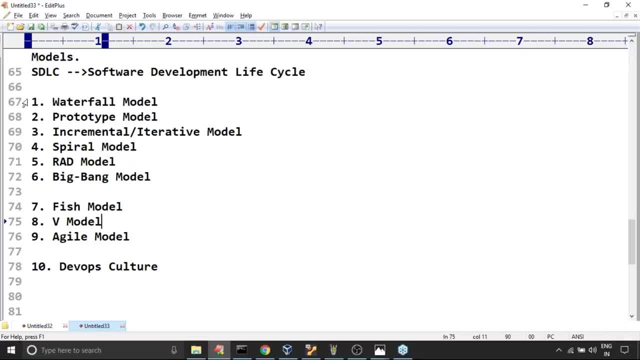 in the future. i want to see which one. the question now my de embarrassing and of course, they are almost around 10 sessions. we require to spend about this, but not required to worry just for the devops. just basic idea. okay, you have to get the first model. the last model i will discuss. 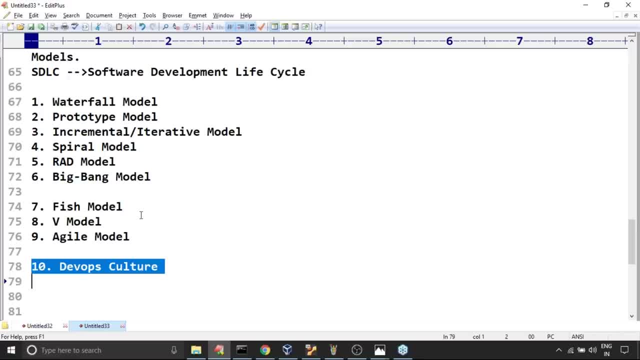 and then i will introduce the devops so that you people can feel more comfortable, i'm sure, sir, okay, like sir. now the first important terminology. let me talk about waterfall model. okay, waterfall model model like okay now here, just take a bit very, very special care. have you observed, sir, in 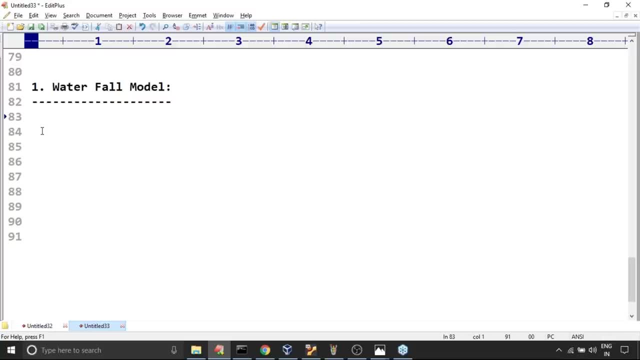 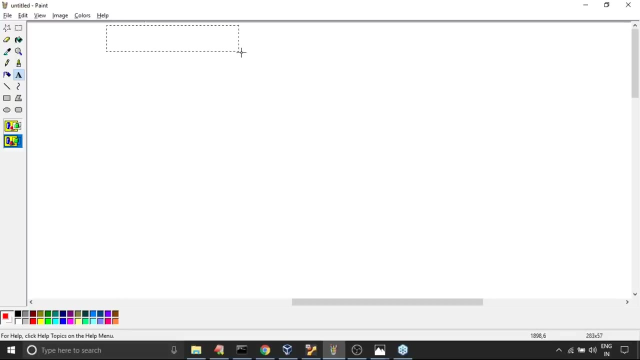 any in any software development model, sdlc. what are various stages or pages are there? can you please confirm the first one, respond. what are various various pages are there? can you please follow? okay, the first. the first thing is okay, i can use the word the first. the first one is a. 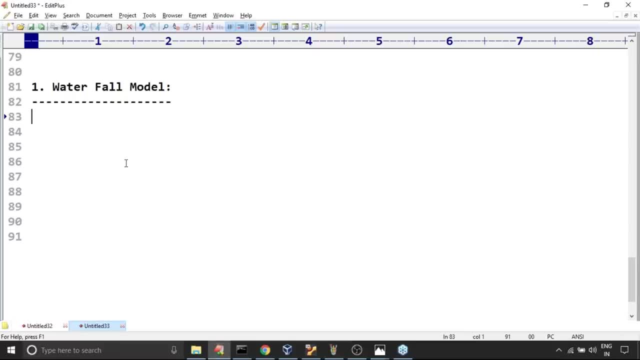 requirement: requirement: requirement analysis. okay, like, just observe the requirement: requirement gathering: requirement gathering: okay, requirement gathering gathering are- some people may use the word collection. okay, we have to collect the requirements, right. requirement collection: what is the second one, sir, can you please guide? requirement requirement analysis. requirement analysis. 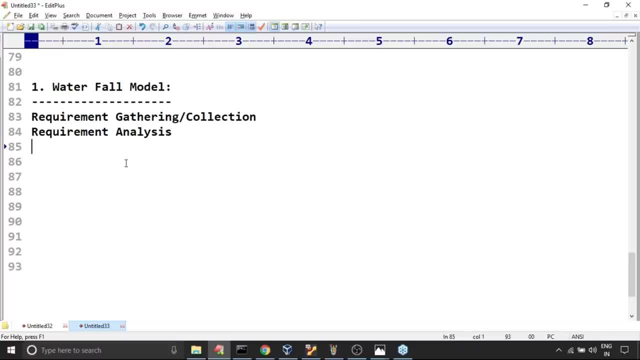 c said many the responsible to do that. okay, see, uh, see, yes, yes, yeah, is that responsible? like next after that: uh, design, okay, design, we have to take. okay, high level design documents, low level design documents like ui. okay, gi design documents. okay, like we, how to? we have to take a design phase. okay, like 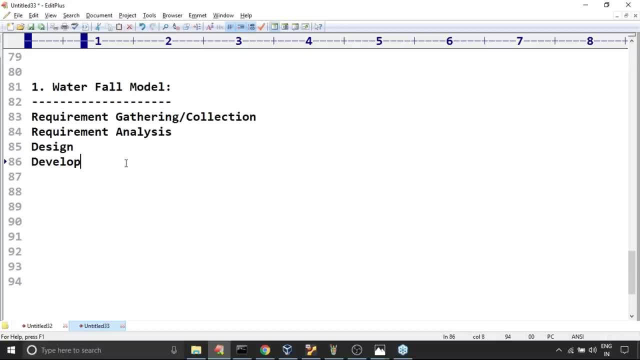 once the design completed. next we have to talk about development. okay or otherwise, coding- we can use the word coding- coding is the more technical word- instead of development, coding, coding, design, coding. once coding got completed, then we have to talk about testing. okay, once, uh, testing, testing itself got got completed, testing itself got completed, then we have to talk about 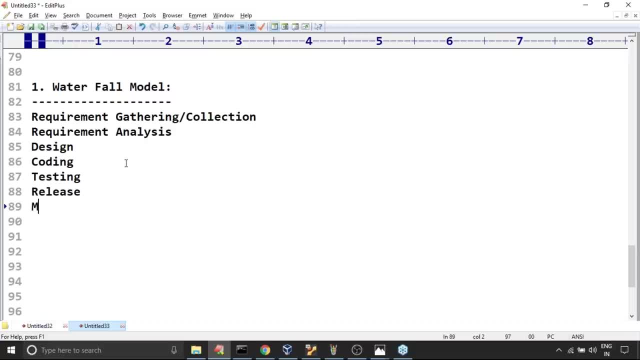 release, okay, release, and then maintenance will come in the picture. okay, release, and then maintenance will come in the picture. okay, that's all testing release, that's all maintenance, like that. so do you know here? so if you, if you consider this model, if you, if you consider this, 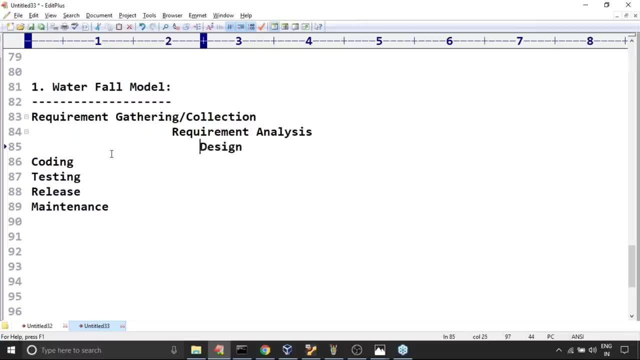 these models are. now, how this model is going to, is going to, is going to work is very important, sir. so, first step, first, what thing we have to, we have to, we have to use. can you please spell out, sir, first, first, what is that? what is the step we require to use? what is the phase first, what is? 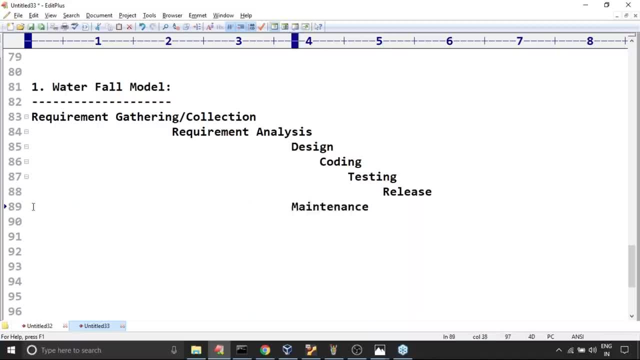 the first phase we have to use, okay, requirement gathering next, and after that, what the next one? we have to take care, okay, like requirement gathering analysis, like now there is one. how this model is going to work is assume that. assume. this is the first step. this is the second. 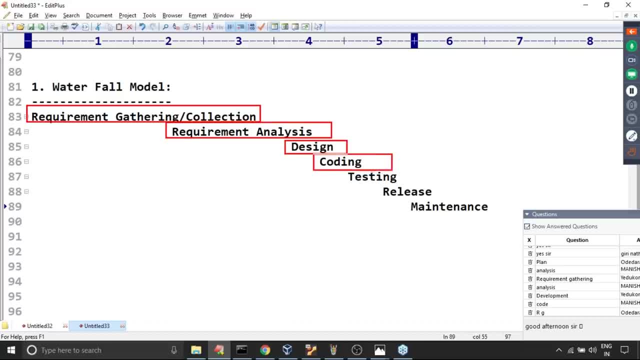 step: okay, this is the third step. fourth step: okay, like sir. next, uh, fifth step. fifth step. sixth step: okay, seventh step. now on the steps: uh, if you flow water, water, if you, if you just uh, if you are, if you are passing the water, how the water will flow? on this, on this, on this, and 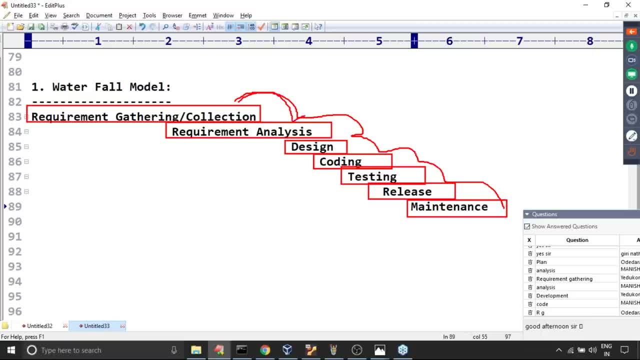 this, on this, on this. so it is flowing just like water from top to bottom. that's why this model is by default considered a waterfall model. remember this one, sir. okay, what are just the first? once first step completed, then only second step is going to start once the second step completed. 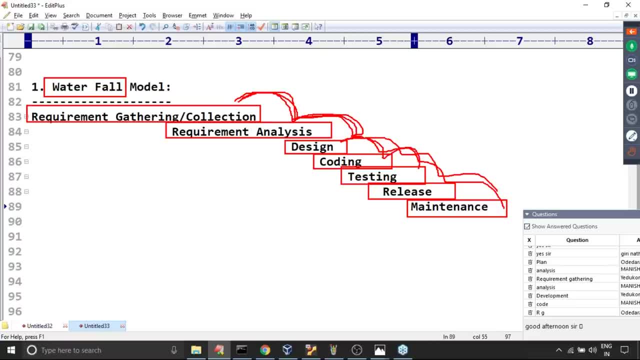 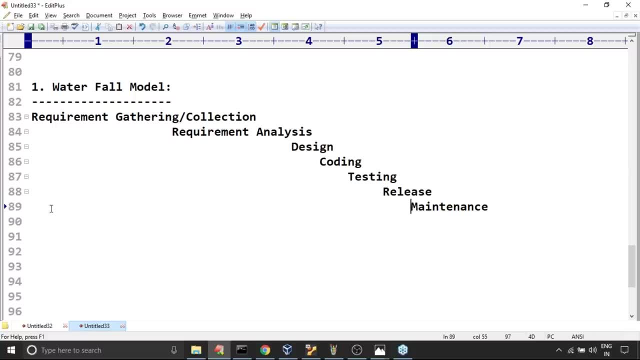 then only third one is going to start, then only fourth one is going to start, then only fifth one is going to start, like this model is by default concerned. yeah, waterfall model, by the way, the word waterfall. are you seeing waterfalls? falling of water. who respond? are you seeing falling? 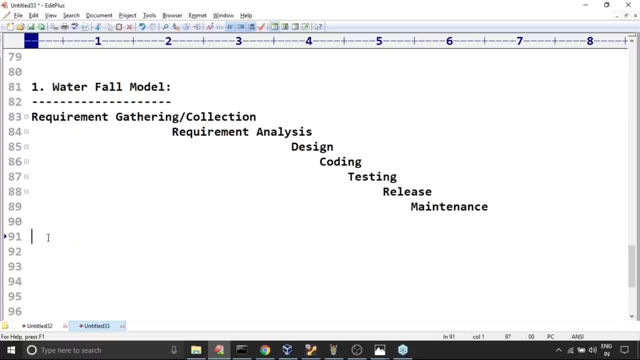 of water. that's why the word waterfall model. okay, like now here. so this model is also known as also also known as sequential, linear, linear sequential model. can i use the word linear sequential model? so this is first. you have to complete this one. after that, this one is: 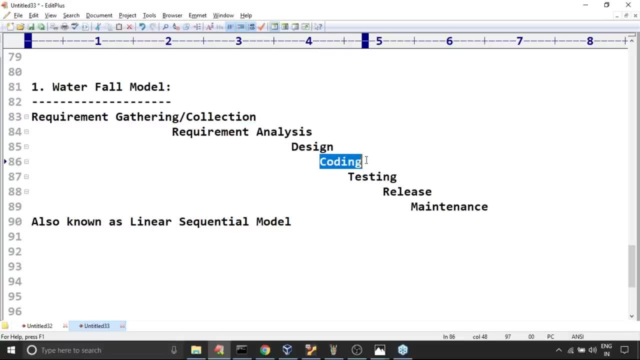 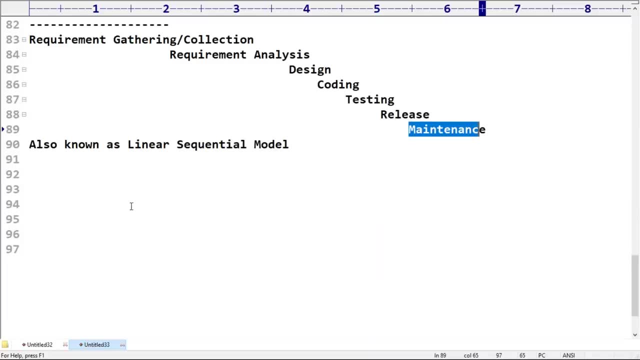 going to start, and then we have to start about this one, and then we have to talk this. we require to talk, we require to talk, we require to talk like this. all these steps are required in the normal waterfall model right now here. so what the advantages are there? what problems? 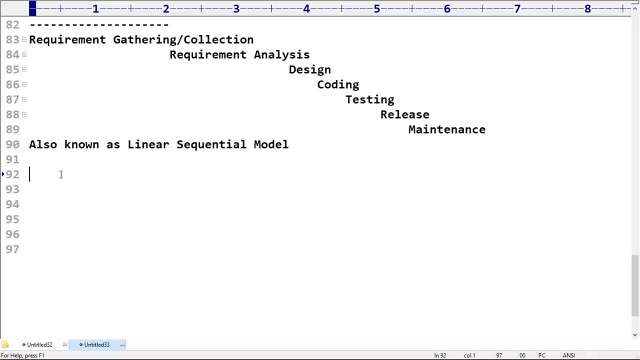 are there because? so just let me talk more on problems aside, because this model is not recommended. what are various models are there? what limitations are there? sir, very, very important point: take very, very special care. okay, like sir. is it applicable for gi projects? no chance at all, okay, whereas those days already. 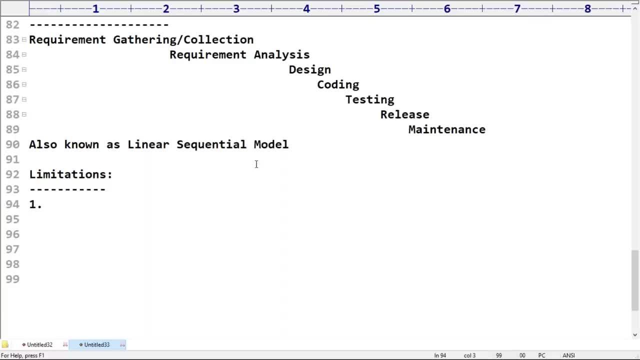 gone. it was a history, okay. 1950s, 1960s, first time the people used a software, product software. at that time. the model is waterfall model. remember. it's almost gone. it was history. no one is going to use. what is the reason for why? 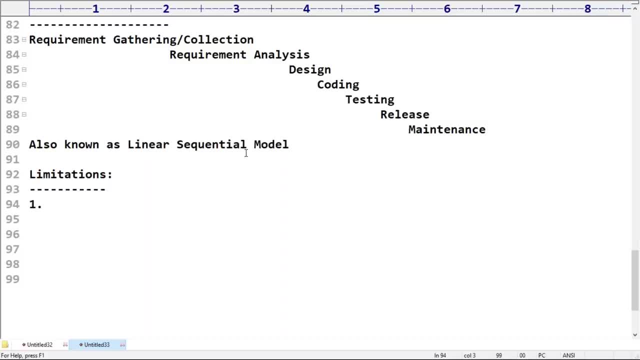 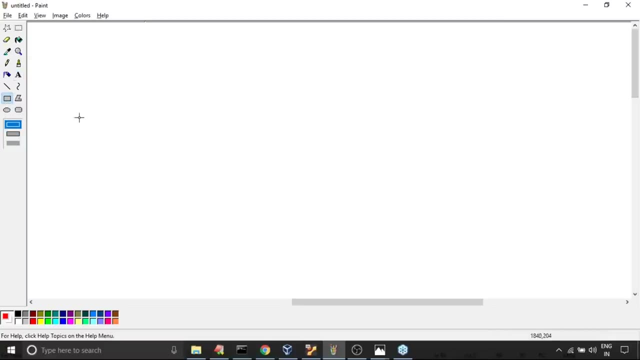 that, okay, like now. observe that very carefully, sir. do you know? there are two examples i will discuss so that you may get much clarity. layman examples: right? suppose i want to build. assume, assume that i want to build some, some three floor building. assume that, okay, simple sir. 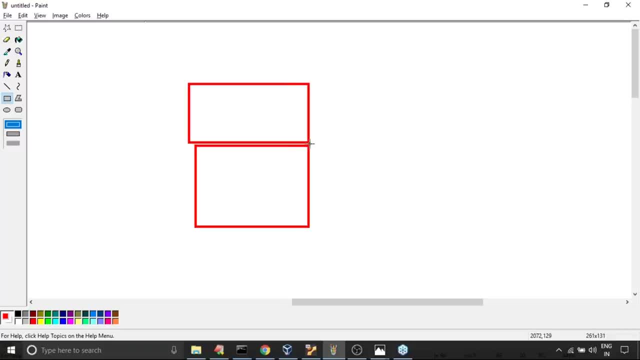 three floor building i want to build. assume maybe scale up until thousand floors also, no problem at all. so first assume that after that you have to build a three-story building, thousand floor building i have to take, i have to construct. okay, assume, sir. now do you know? 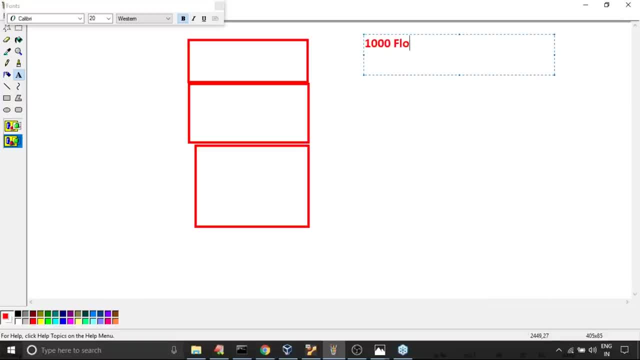 first, sir, this is about my, my requirement: thousand floor building. now, my requirement is observe that, sir, first floor, okay, pillars, and then slab completed. okay, under them. second floor, pillars and then slab, slab completed under them. third floor, pillars and then slab completed. okay, like after like all the thousand floors, sir, pillars and the slab completed, assume that pillars. 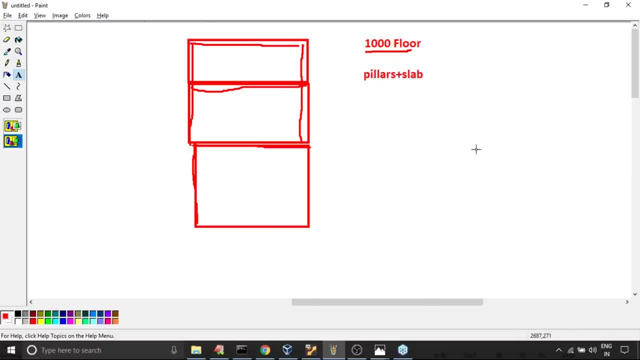 and the slab slab completed after that. now i want to talk about, okay, flooring of the first floor, flooring, flooring, flooring of the of the first floor, flooring of the first floor. next, i have to talk about flooring of the second floor next, and after that i have to talk about flooring of the third floor. like all the thousand completed, all the thousand. 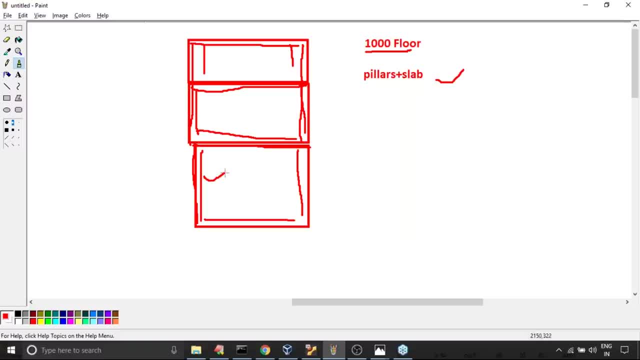 completed. now i have to talk about electric electrical work of the first floor, electrical work of the second floor. electrical worker, sir, are you going to do like this, one by one, one by one? is it unnecessary time, waste or not? array, you have to if you are going to. 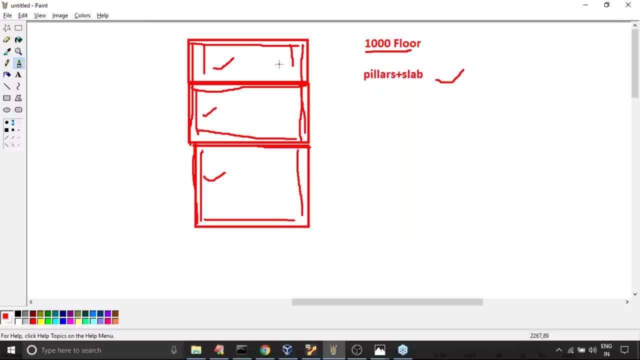 do: first activity in all thousand floors. second activity in all thousand floors. third activity in all thousand floors. so start to construct a thousand floor. bill, eh, minima, minimum, ah, sir. 10 to 15 years must be required. sir, you have to construct a thousand floor building. are you getting right? 10 to 15 years must be must be required. it's very difficult, it's very time based cost. cost is going to be increases, like anything. it is never recommended right now. my question is, sir, whenever second floor pillars started, why don't you start interior? 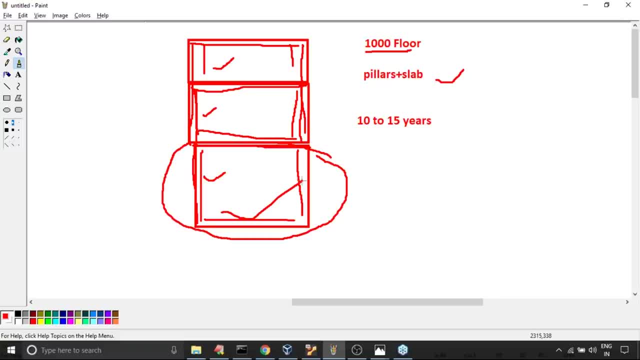 work up a store are you getting? why don't you start a interior workup first floor, so that there is a separate team is going to work in this, in this first floor interior work. meanwhile, second floor pillars and slab is going to be ready whenever third floor, whenever third floor pillars. 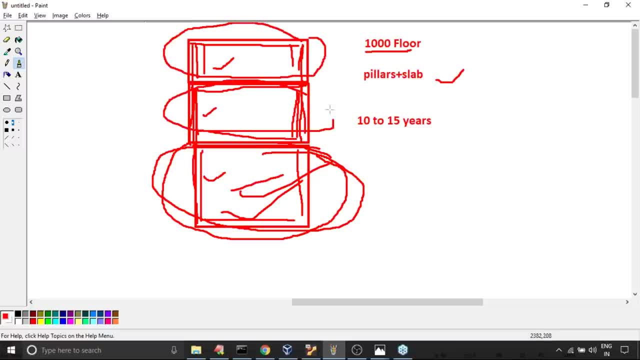 and slab is going to be there, interior work or second floor is going to start. next the paint work up the first floor is going to start. okay, like if multiple people are going to involve, like that, instead of doing one by one on by one parallely. if they are going to do, is it really? 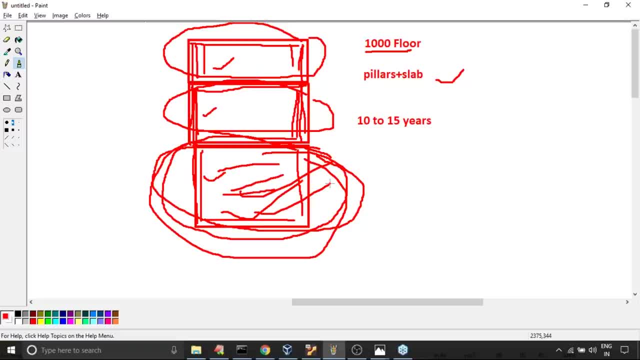 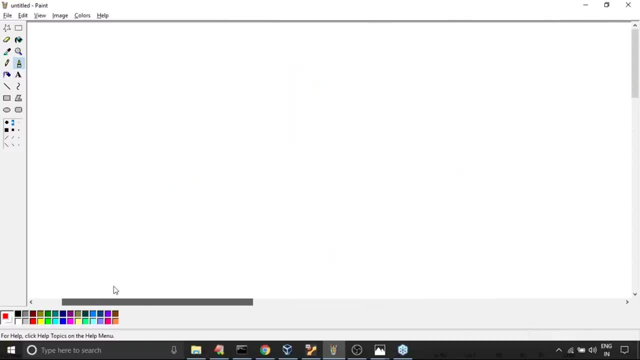 advantage or not? yes, friends, are you in the position to understand? okay, this is, this must be required, man, okay, like, suppose here best another example to understand. i will, i will, i will tell. just observe that, suppose here, assume that, okay, thousand thousand kilometers road, thousand kilometers national highway, national national highway, sir, we have to, we have to, there is a. 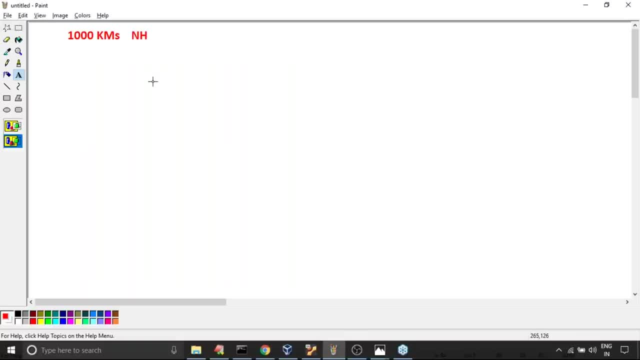 contractor got national highway he is responsible to construct. so what he has to do is first all the thousand floors, okay, first level road, all the thousand kilometers. first level road means raw material. they are going to flow and then they have. they have to keep some concrete. all the thousand. 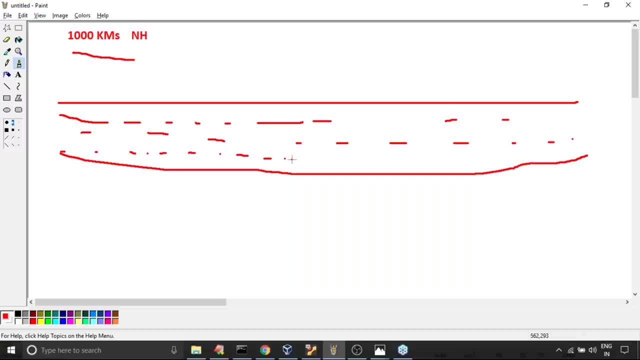 kilometers and then they have to go for us or what we call damper, or something like concrete, like he has to. no, no, no, they never going to do like that what they will do. yes, sir, these five kilometers, one team is working. okay, the first five kilometers: one team is working. 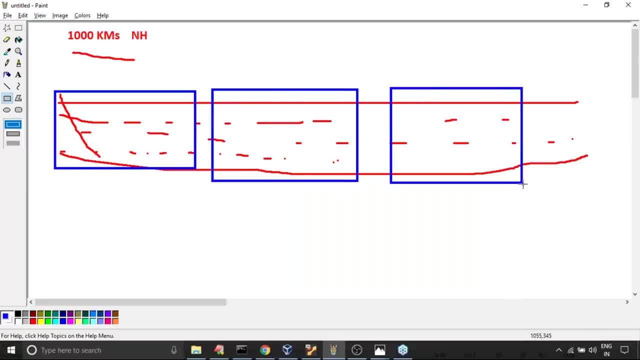 next the five kilometers. another team is working, next five kilometers, another team is working like: so these five kilometer, these five kilometer. there is no dependency at all why we have to wait. man, okay, in the first five kilometers only, first five kilometers only. all stages are going to be. 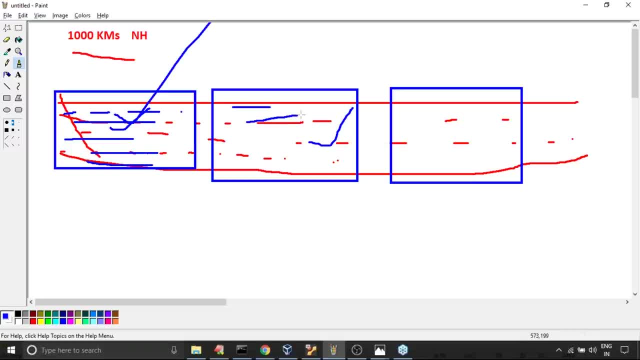 completed, ready to use next five kilometers. okay, so parallelly it's, it's going on like so. this type of development is always highly recommended. anyone, are you in the position to understand? this type of development is always highly recommended. anyone, are you in the position to understand? 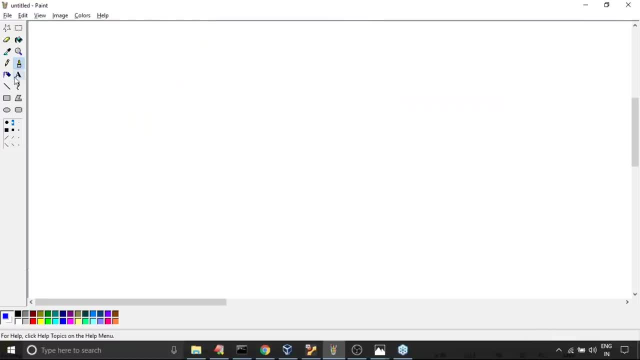 yes, friends, okay, like, suppose best example, if you consider hyderabad metro, hyderabad metro, if any person is coming from hyderabad, hyderabad metro or otherwise, university also metro is there, just observe that. array: first first, okay, first first metro, sir, hyderabad metro is assumed that, assume, assume that sub total, total, the 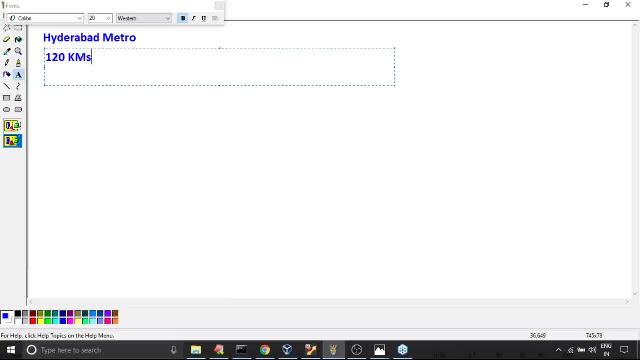 suggest, sir, 120, 120 kilometers, total 120 kilometers. sir, four lines are there. assume that four lines are there now. so all 120 kilometers, all four lines, first pillars has to be started, first pillars has to be constructed. next, after completing all 120 kilometers, four lines. 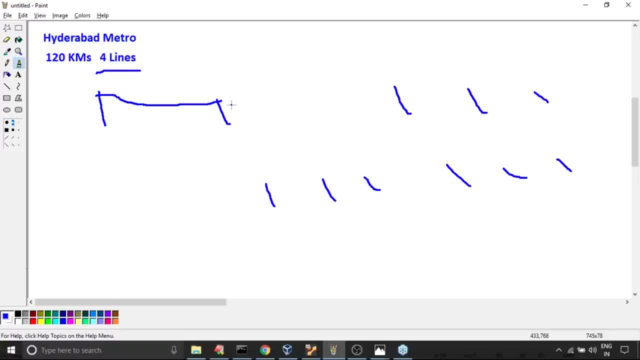 then then okay, next level work is going to start. no, the people are not going to do like that. what they will do? yes, they will start four lines parallelly. they will start four lines parallelly. okay, now, once a first line completed, even yet, it will be used. okay, after two or three months, next thing is going to be completed. 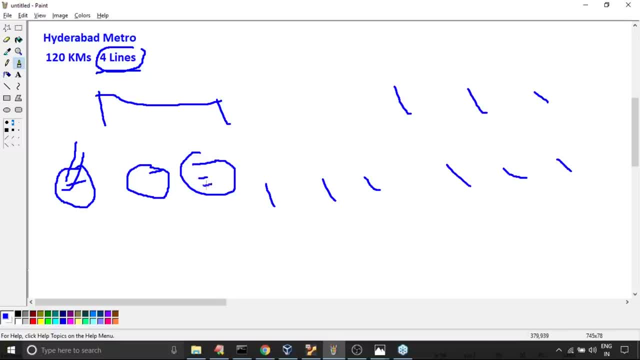 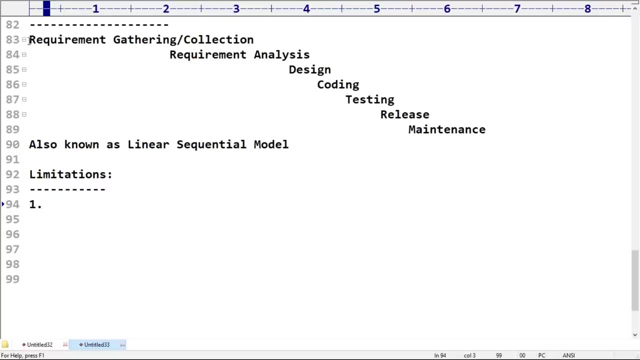 after two or three months, the next thing is going to be completed they never going to think about, from first to last, under the next level. under the next level, like: are you in the position to understand, okay, the problem with this waterfall model? are you seeing right? hey, once you started. 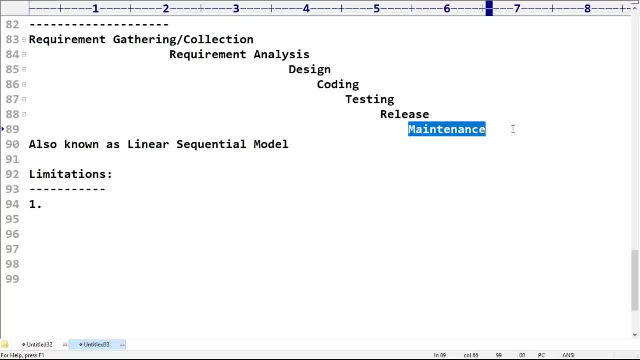 once you started here. next, until completing last one. okay, there is no, there is no changes in the middle. okay, once the last thing completed, then only we have to talk about next level. but how worst it is. yes, friend, so suppose here you are in the coding stage. assume that. so until until. 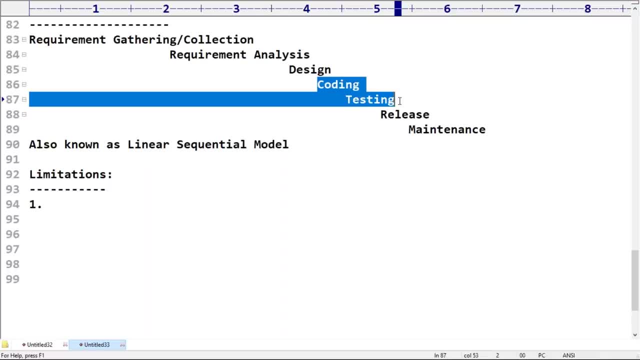 design completed. the developers and the testers should be vacant. they are not having any work. they are not having any work. okay, until coding completed. testing team will be just. they have to come to the office and they have to go free. okay, like it is, it is a bigger the. 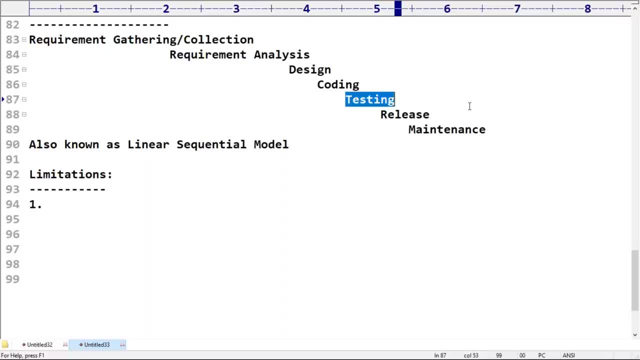 problem unnecessary, okay. cost of the project is going to be increases, like anything. development time is going to increase like anything. are you getting right? development development time will be increases. development time will be increases, okay. remember. next, the cost of the project: development, cost of development development will be increases, will be increases, okay, like. 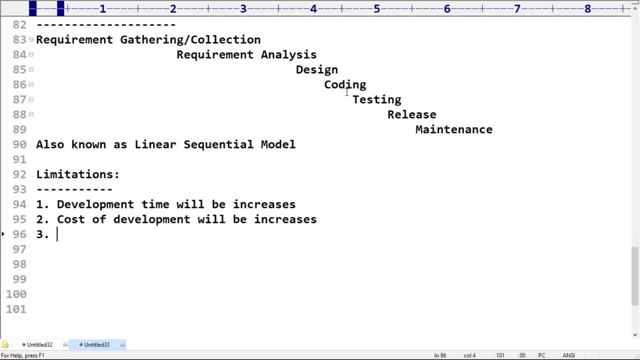 sir, observe next. next, it won't accept requirement changes in the middle. okay, suppose already coding started, sir. suddenly client came. sorry, i have some changes in my requirement. what we have to do, have you observed? coding already started now? now, suddenly client came. sir, we have some requirement. 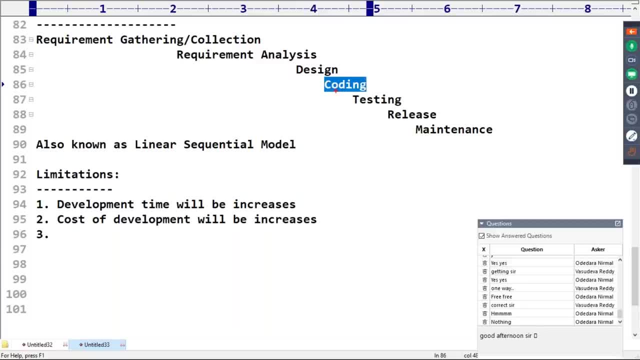 changes what we have to do? nothing, nothing. so again, again, we have to start from beginning. only, okay, like it is. uh, so it won't accept it, won't? it won't accept the acceptor. changes in the middle, changes requirement: changes in the middle: okay, it won't accept the requirement. 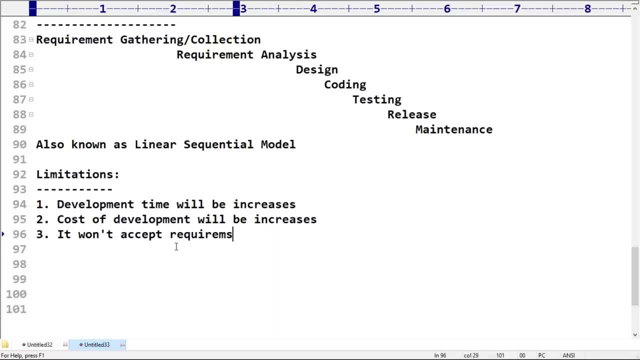 changes. requirement changes in the middle. okay, like requirement changes in the middle. if it is not going to accept requirement changes in the middle, then the client satisfaction is very, very low. okay, claim the client satisfaction. claim the satisfaction is very, very low because so in day, two, day, uh sir, every every day the changes, new trends are going to come. sorry, okay, i don't want this. can? 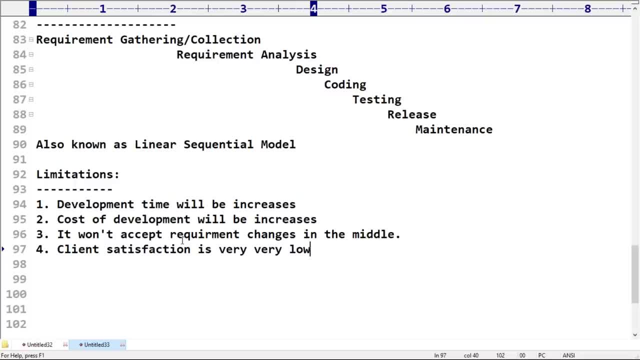 you please change my requirement? can you please change the requirement like? so this model is not in a position to provide support. remember a bit very carefully about this. are you in the position to understand, right? client satisfaction is very, very low, low. okay, like next? uh suppose here, sir. 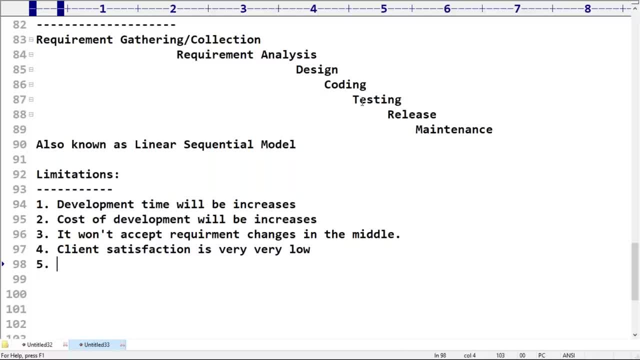 if there is a bug, if there is a bug, when the bug is going to be identified somewhere at last stages, at last stages, do you know, bug identification. the cost of bug fixing is very high because then it will be after completing total product. then only we have to identify the. 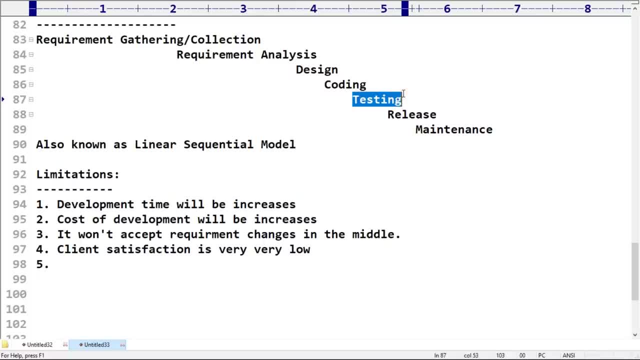 bug are you getting? after completing total product, then only we require to identify the bug. okay, so now fixing? okay, fixing is bug. bug fixing is a very costly. bug fixing is very costly because- because, okay, we can't identify. we can't identify bugs in early stages of life cycle. remember these ones are in yearly early. 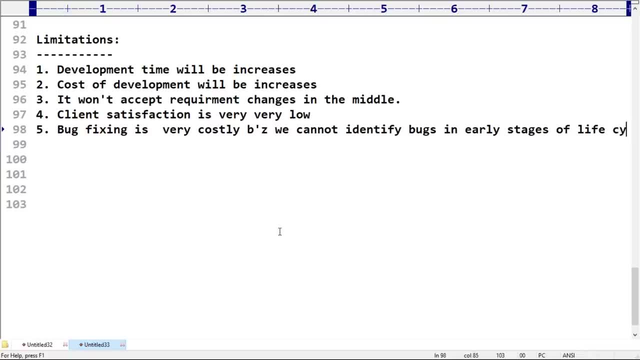 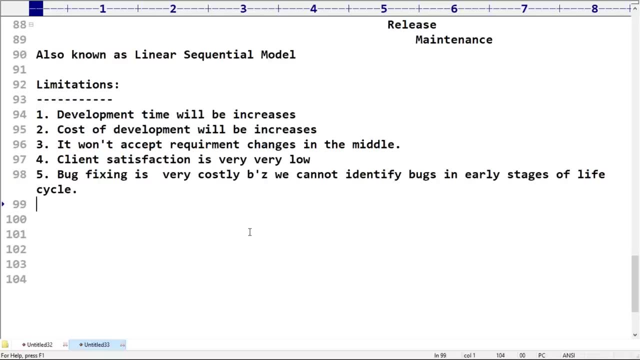 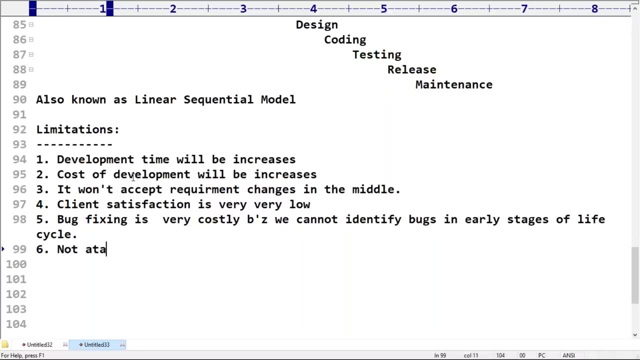 stages of life cycle. okay, we can't identify bugs. okay, like next: uh, not suitable if the requirements keep on changing. have you observed right? if the requirement keep on changing. sorry man, this type of model is a waste. so not suitable, not at all suitable. suitable if requirements keep on changing. requirements keep. 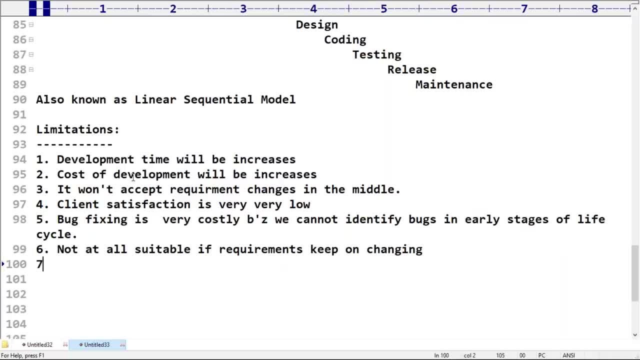 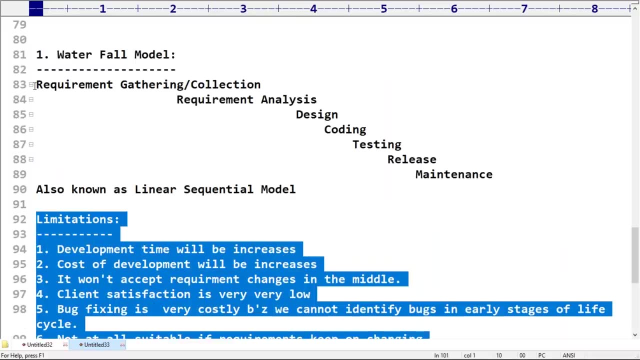 keep on changing. next: not suitable for large projects. remember this one: not suitable for large projects. not suitable for large projects like so n number of problems are there. that's a like so n number of problems are there. that's a like so n number of problems are there. that's a why waterfall model was a history. no one. 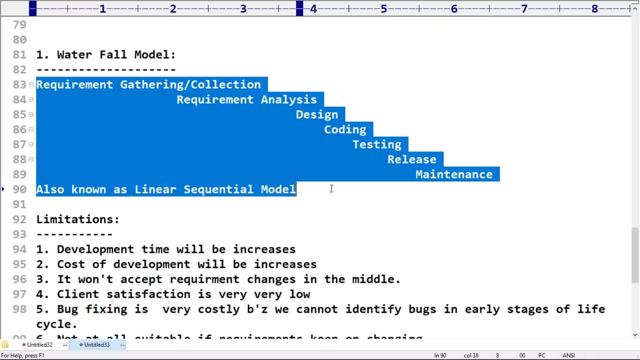 why waterfall model was a history? no one. why waterfall model was a history. no one is going to use this model. is going to use this model. is going to use this model? any doubt, any, any doubt about this one? any doubt, any, any doubt about this one. any doubt, any, any doubt about this one? okay, like then, immediately, master sir. 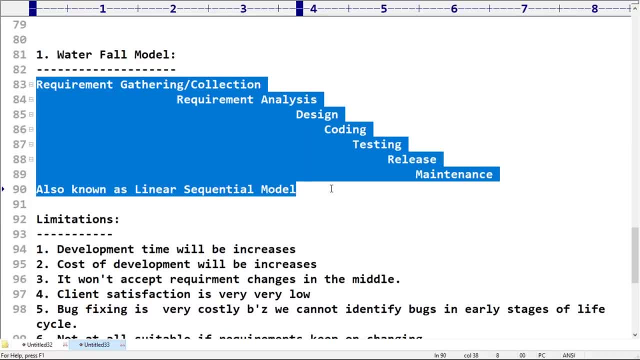 okay, like then, immediately master sir. okay, like then immediately master sir. sir, here you are telling all the sir, here you are telling all the sir, here you are telling all the limitations, maybe some advantages also limitations, maybe some advantages also limitations. maybe some advantages also there. okay, advantages are okay everything. 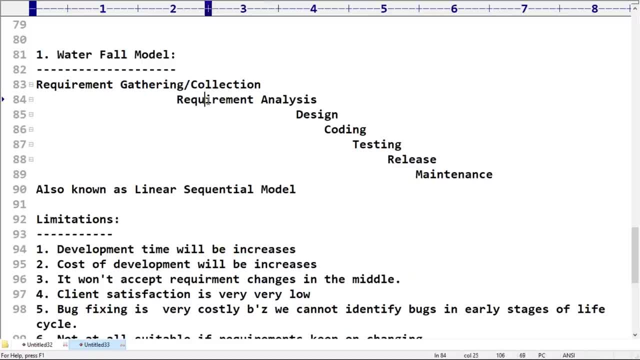 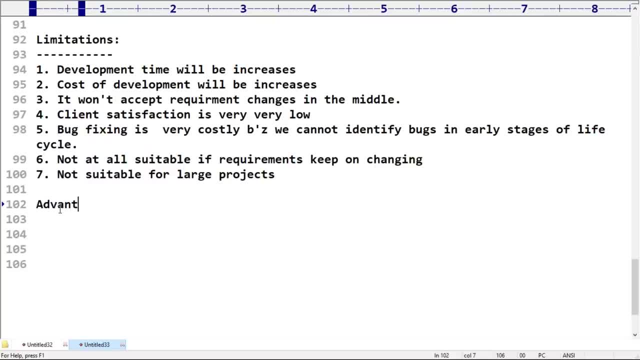 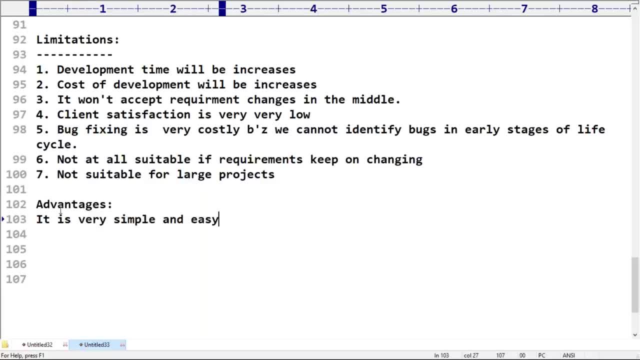 is a is a very simple. it is very, very simple and very simple. it is very, very simple and very simple. it is very, very simple and easy to implement and easy to implement and easy to implement and easy. easy to implement the correct or not. easy, easy to implement the correct or not. 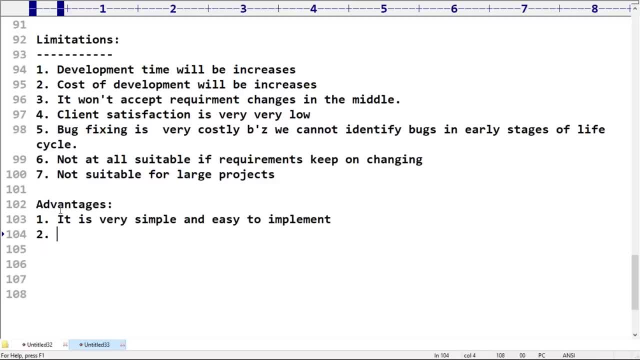 easy. easy to implement. the correct or not. it's very simple and easy to implement. it's very simple and easy to implement. it's very simple and easy to implement. okay, next turn after that. okay, like okay. next turn after that. okay, like, okay, next turn after that. okay, like it is, it is easy to next. best suitable. 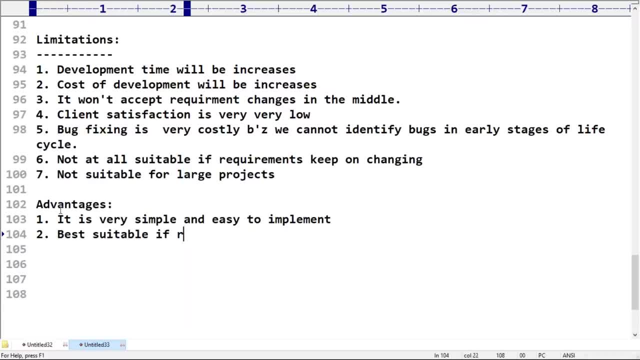 it is it is easy to next best suitable. it is: it is easy to next best suitable if the requirements are fixed, if the requirements are fixed, if the requirements are fixed, okay, best suitable if requirements. if okay, best suitable if requirements. if okay, best suitable if requirements, if requirements are fixed. 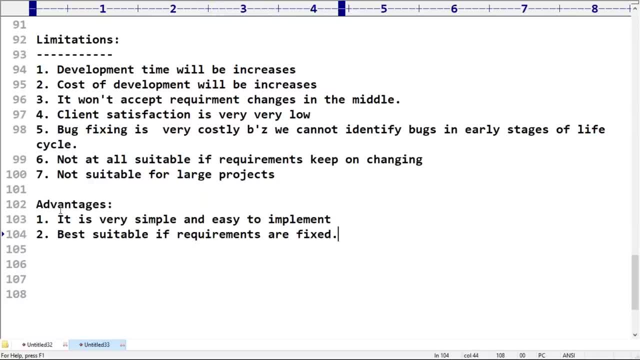 requirements are fixed, requirements are fixed. if requirements are fixed. next best if requirements are fixed, next best if requirements are fixed. next best suitable for small projects. suitable for small projects. suitable for small projects: okay, best suitable for small projects. okay, best suitable for small projects. okay, best suitable for small projects, for small small projects like. 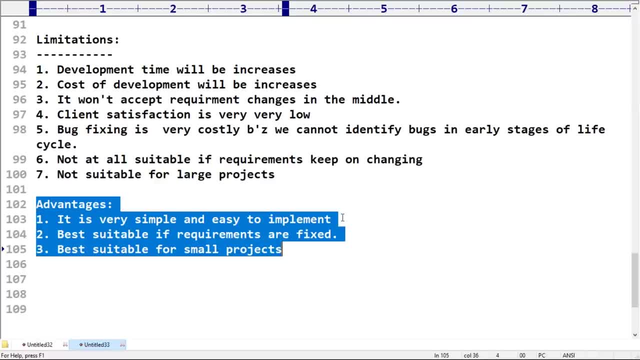 for small, small projects, like for small, small projects. like okay, but anyway, it was the history, that's okay, but anyway, it was the history, that's okay, but anyway, it was the history. that's why what is the use of knowing? why, what is the use of knowing? 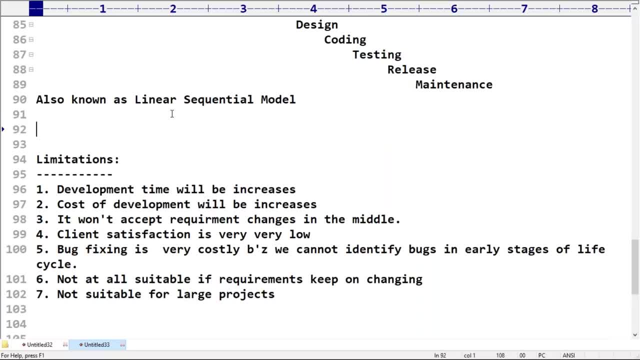 why what is the use of knowing advantages? it is meaningless observe the advantages. it is meaningless observe the advantages. it is meaningless observe the problems especially right. why this model problems especially right, why this model problems especially right. why this model is not suitable, why this is not suitable, why this? 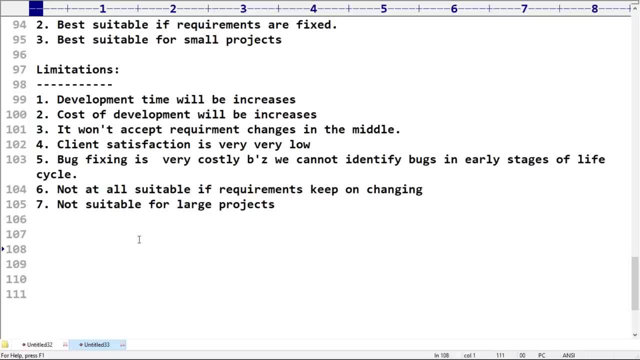 is not suitable. why this model is not using that much frequently? model is not using that much frequently. model is not using that much frequently these days. you should have clear clarity these days. you should have clear clarity these days. you should have clear clarity. any doubt, any doubt. 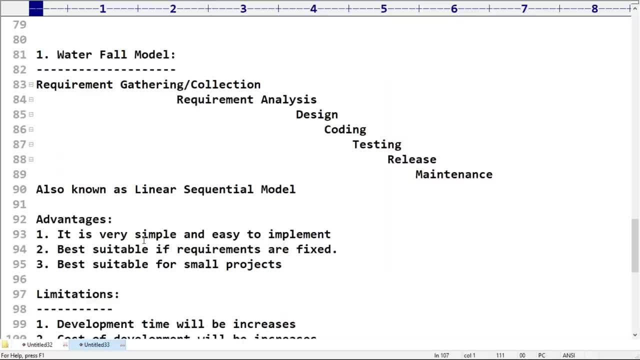 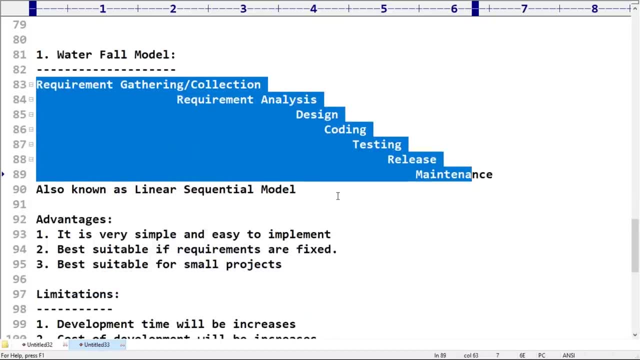 any doubt. yes, yes, yes, was every day, was every day, was every day. okay, no overlapping between the pages- okay, no overlapping between the pages. okay, no overlapping between the pages. like there are multiple: okay, like so. like there are multiple- okay, like so. like there are multiple, okay, like so. why waterfall model is not frequently? 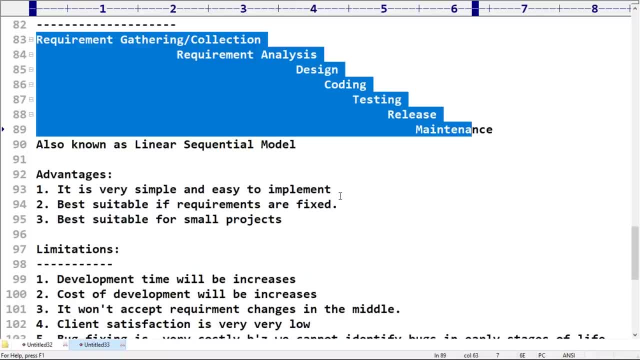 why waterfall model is not frequently. why waterfall model is not frequently used, this not frequently. no way the used this not frequently, no way the used this not frequently, no way. the people: why the people are not using this people, why the people are not using this people, why the people are not using this model, why it was the history. so now i 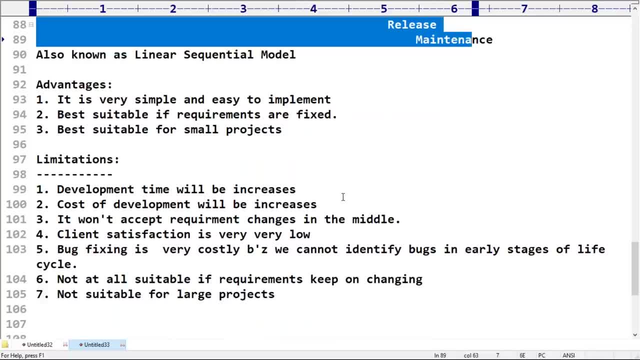 model why it was the history, so now i model why it was the history, so now i hope you are in the position to hope. you are in the position to hope, you are in the position to understand this one right, understand this one right. understand this one right. okay, like now. 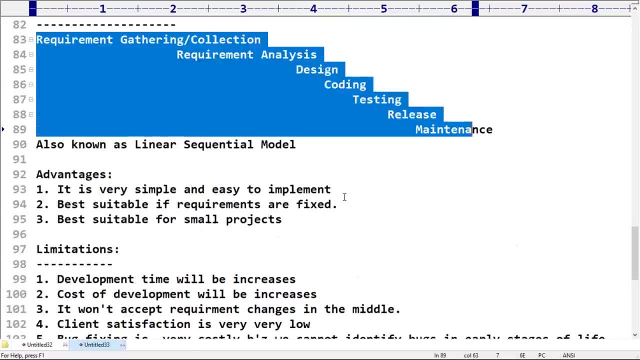 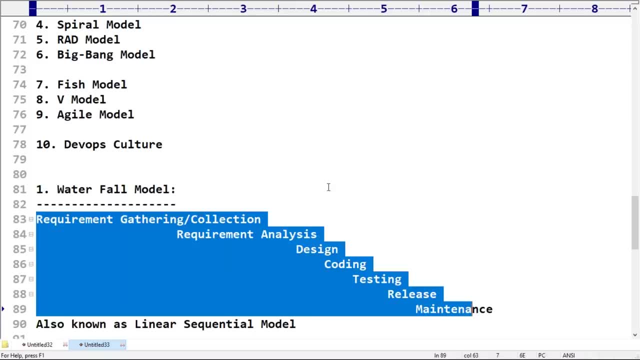 okay, like now, okay like now, now, now, now, now, take, take, take, very very special care. okay, very very special care. okay, very very special care, okay, so the most, so the most. so the most recent model, recent model, recent model for the webster, the most recent for the webster, the most recent. 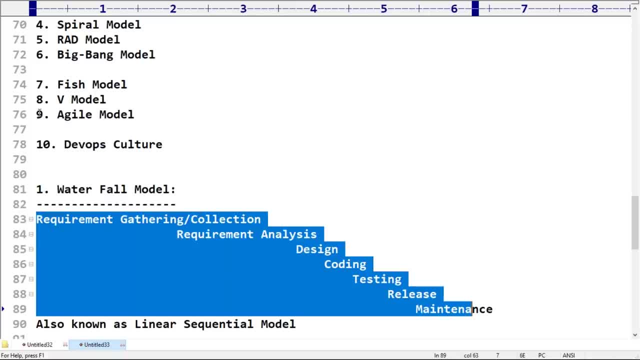 for the webster. the most recent hot cake model: hot cake model in the in. hot cake model. hot cake model in the in. hot cake model. hot cake model in the in the market is, have you aware, the market is. have you aware, the market is, have you aware, as i, as i, as i. 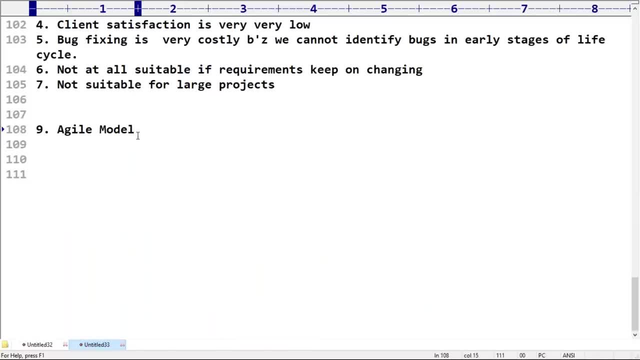 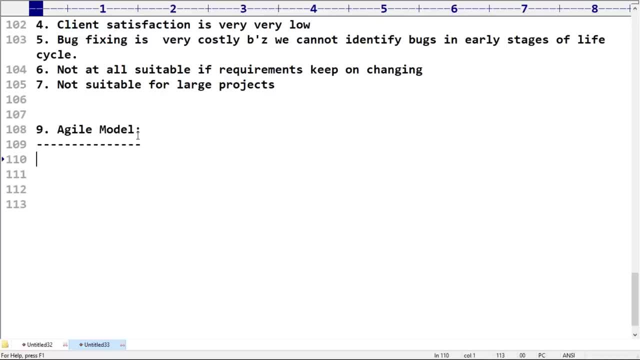 yes, friends, do you know? last, if, if you in the software company, in the software, in the software company, in the software, in the software company, in the software company, if you can ask any person, ah, we company. if you can ask any person, ah, we company. if you can ask any person, ah, we are using agile as i, model as i. 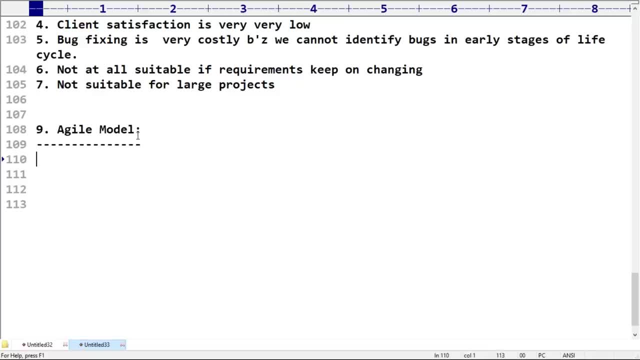 are using agile as i model, as i are using agile as i model, as i methodology. we are using as i as i- okay- methodology. we are using as i as i- okay methodology. we are using as i, as i- okay, like, like, like. so now i can use the word. this is the. 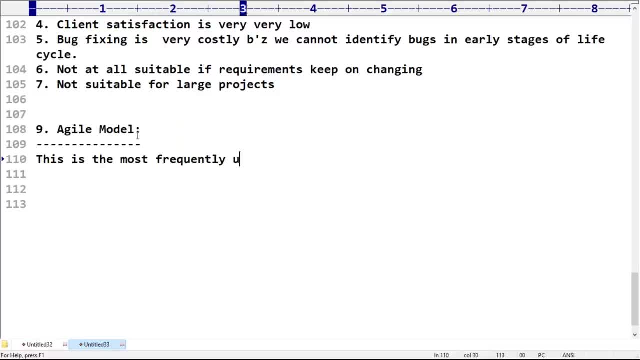 so now i can use the word this is the. so now i can use the word this is the most frequently. this is the most most frequently. this is the most most frequently. this is the most frequently used under. frequently used under. frequently used under: hot cake model: okay, in in software. 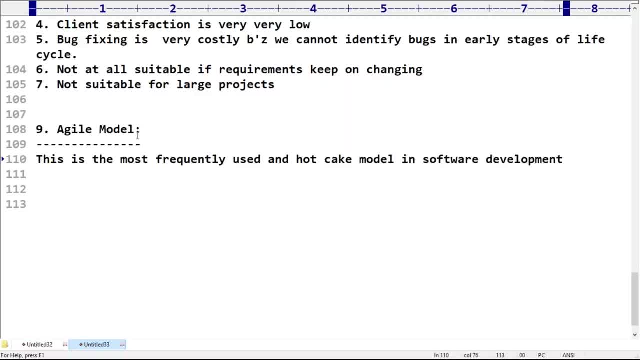 hot cake model: okay, in in software hot cake model: okay in in software development. development development, okay, but not now. okay, now the trend is okay, but not now. okay, now the trend is okay, but not now. okay, now the trend is the dev apps, the dev apps, the dev apps. okay, remember, this is the most frequently. 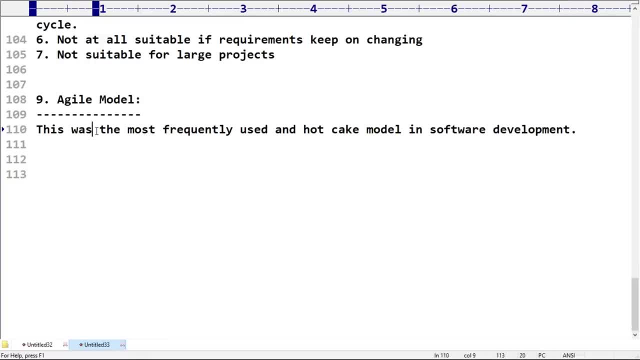 okay, remember this is the most frequently. okay, remember this is the most frequently. this was, this was, this was. i can use the word was, but the most i can use the word was, but the most i can use the word was, but the most frequently used, frequently used. 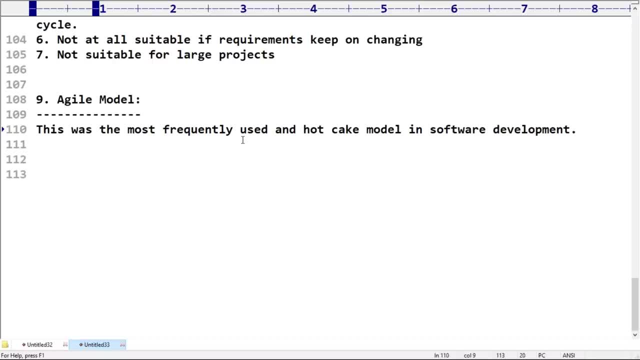 frequently used on the hot cake model in software. on the hot cake model in software, on the hot cake model in software development: almost around development, almost around development, almost around 10 to 20 years. this model last 10 years. 10 to 20 years. this model last 10 years. 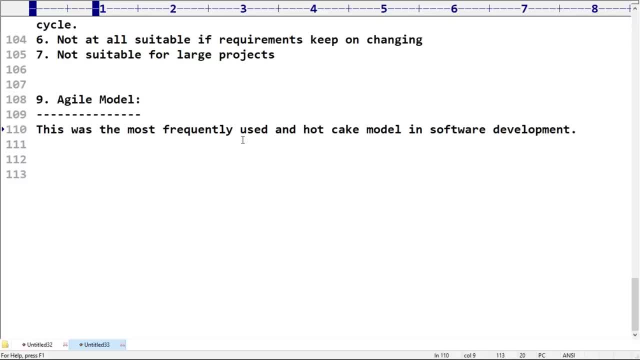 10 to 20 years. this model last 10 years, last 10 years around, last 10 years around, last 10 years around- this model was the hot cake in the market. this model was the hot cake in the market. this model was the hot cake in the market. okay, like. 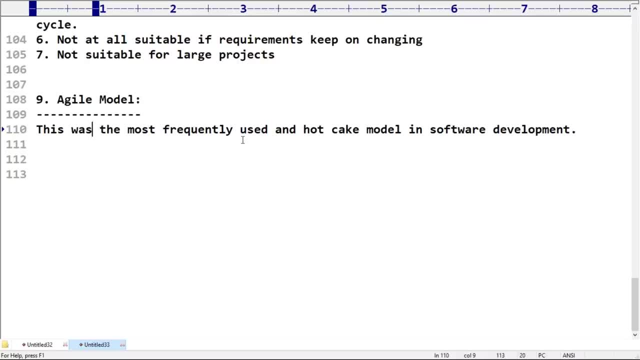 okay, like, okay, like, sir, now. so as i made the agile model, sir, now, so as i made the agile model, sir, now. so as i made the agile model is divided into multiple sub models. are is divided into multiple sub models. are is divided into multiple sub models. are there, sir? 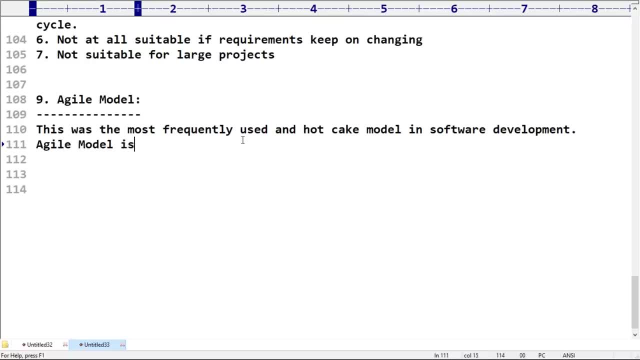 there, sir, there, sir, okay, just these words are very important, okay, just these words are very important. okay, just these words are very important. sir, sir, sir. agile model is divided into agile model is divided into. agile model is divided into multiple sub models, multiple sub sub, multiple sub sub. 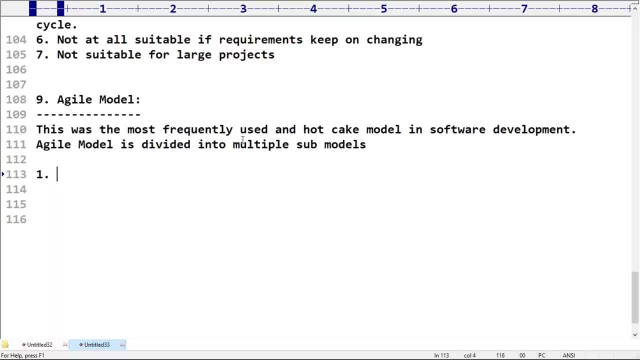 multiple sub sub models, models like suggest, models like suggest, models like suggest: observe these. of course we are not observe these. of course we are not observe these. of course we are not required to worry, required to worry, required to worry about these things, even the people who, about these things, even the people who. 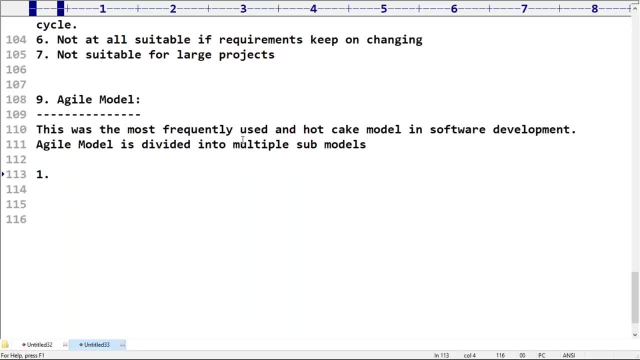 about these things. even the people who are working in the companies also are working in the companies, also are working in the companies also, it is not required just hear the words. it is not required just hear the words. it is not required, just hear the words. okay, first one rational. 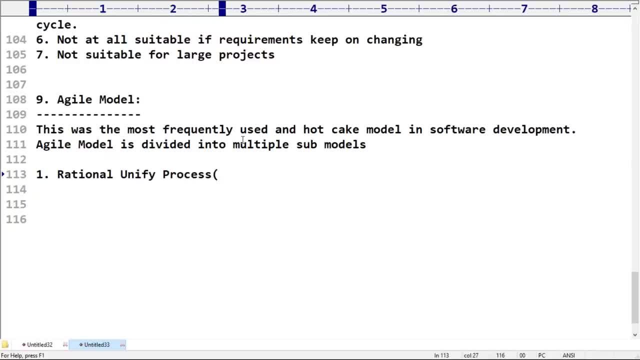 okay, first one rational. okay, first one rational unify process. okay, what are the first unify process? okay, what are the first unify process? okay, what are the first ones are: can you please fill out ones? are: can you please fill out ones? are: can you please fill out rational unify processor? 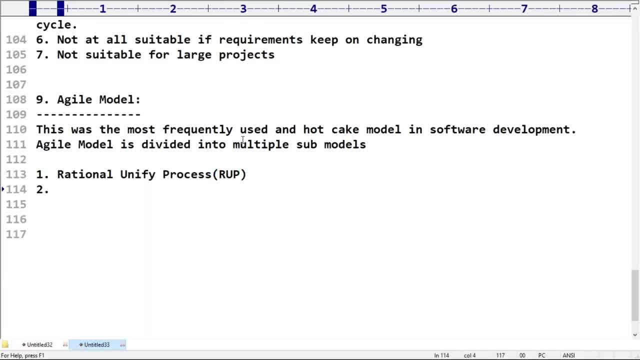 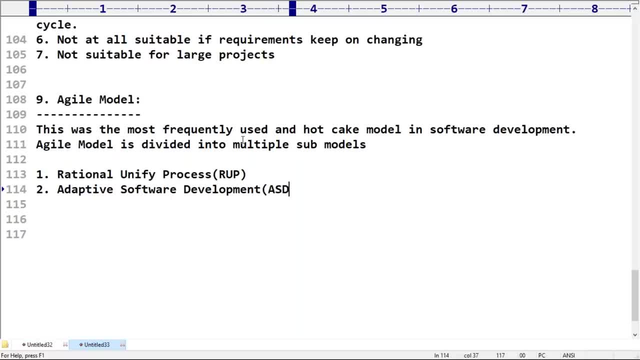 okay, development, okay, development. do you know we can use the word? do you know we can use the word? do you know we can use the word? a s d okay, a s d adaptive software. a s d okay, a s d adaptive software. a s d okay, a s d adaptive software development. next, 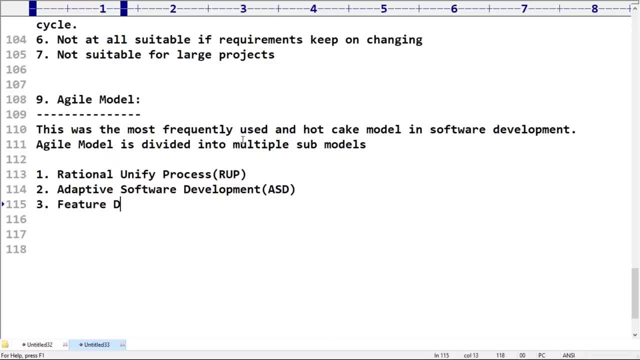 development. next development. next feature given development. sir feature feature given development, sir, feature feature given development, sir feature driven driven driven, driven driven driven uh development, sir. development feature uh development, sir development feature uh development, sir. development feature driven development. okay, like a f driven development, okay like a f. 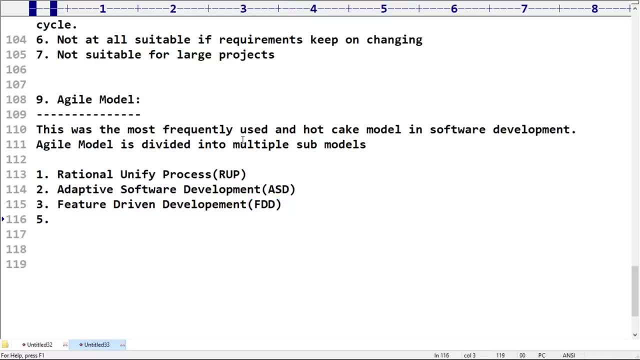 driven development. okay, like a f d d, we can use the word f d d. okay, like d d, we can use the word f d d. okay, like d d, we can use the word f d d. okay, like next crystal clear: okay, crystal crystal. next crystal clear: okay, crystal crystal. 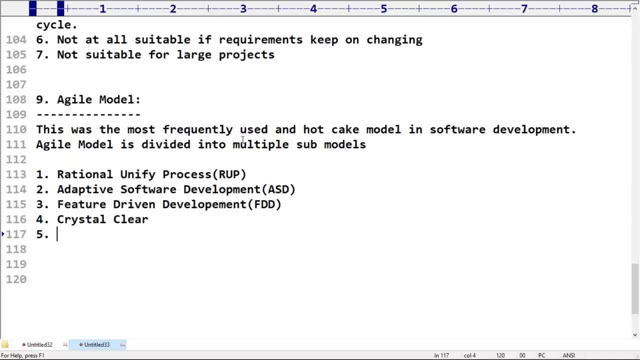 next, crystal clear. okay, crystal crystal clear. it is also one sub model of clear. it is also one sub model of clear. it is also one sub model of agile crystal, agile crystal, crystal, crystal, clear, dynamic, okay, dynamic, dynamic, clear, dynamic. okay, dynamic, dynamic, clear, dynamic, okay, dynamic, dynamic software, dynamic software development. 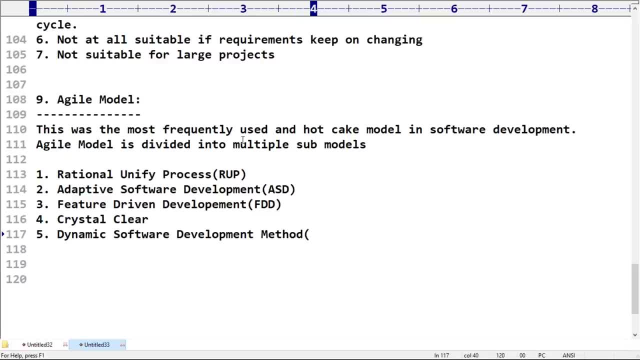 software dynamic development. software dynamic development, development- okay method. don't worry, all development okay method. don't worry, all development okay method. don't worry all these names, you are not required to these names. you are not required to these names, you are not required to worry, just worry, just. 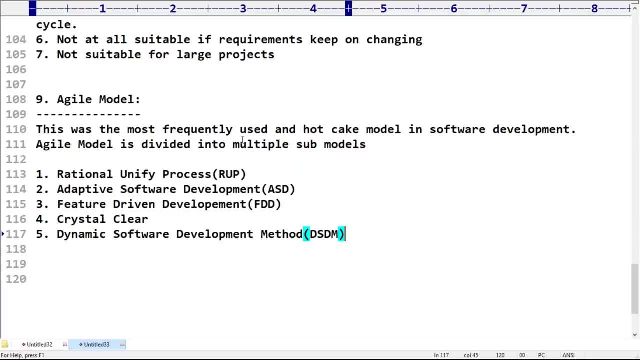 worry, just aware the words. so that's all d s d aware the words. so that's all d s d aware the words. so that's all d s d m m m. okay, like next, uh, extreme programming. okay, like next, uh, extreme programming. okay, like next, uh, extreme programming, extreme, extreme programming, extreme. 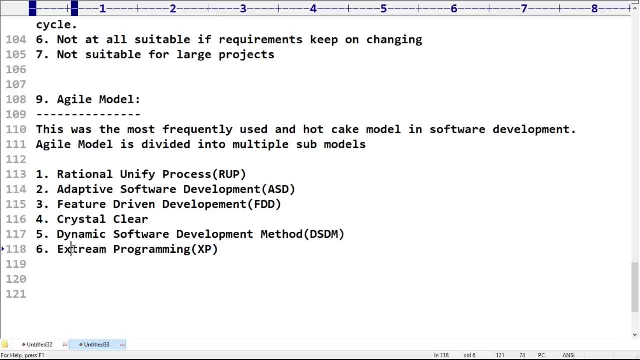 extreme, extreme programming, extreme, extreme, extreme, extreme programming, extreme programming, xp programming, extreme programming, xp programming, extreme programming, xp. okay, extreme x stream. okay, okay, extreme x stream. okay, okay, extreme x stream, okay, xp, something like okay, next, uh, next, the most valuable. i hope this word you people may heard. 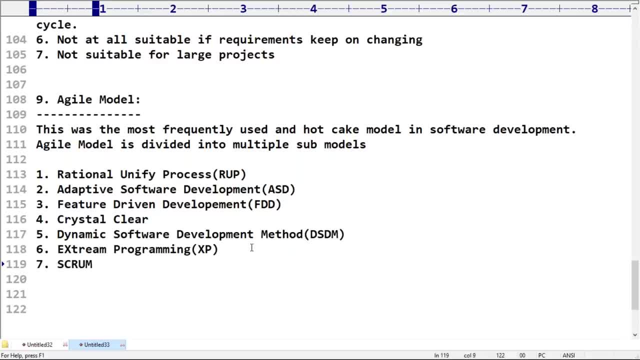 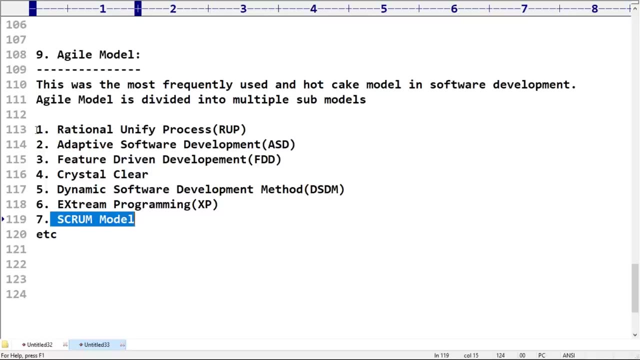 scrum, scrum. have you heard about this one? we respond: scrum, scrum, model. have you heard about this scrum? okay, like now, the people, especially you, are working in the companies. this word is the very popular word in the company in exile. remember that there are multiple sub models are: 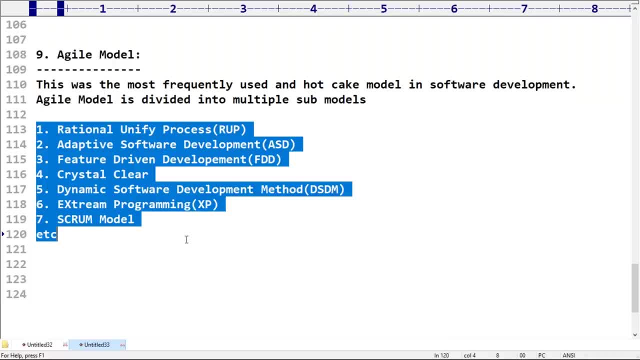 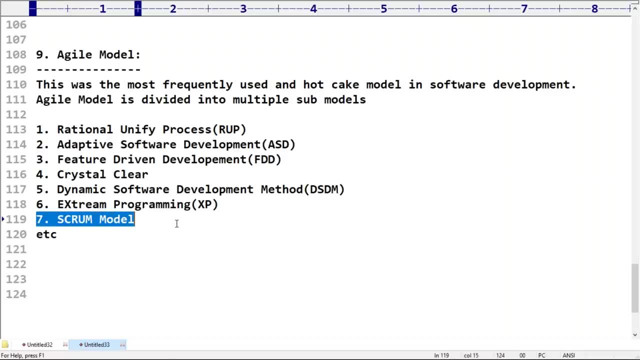 there. but among all these sub models, among all these sub models, okay, which model is the very popular, sir, scrum, scrum model is the very, very popular. remember a bit very carefully about, okay, yama, all these models, yama, all these models, models, which model is the most popular? and? 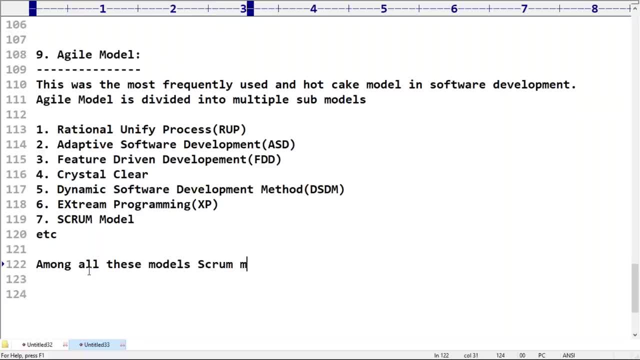 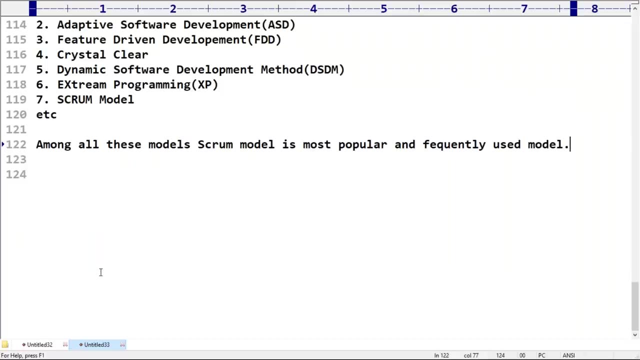 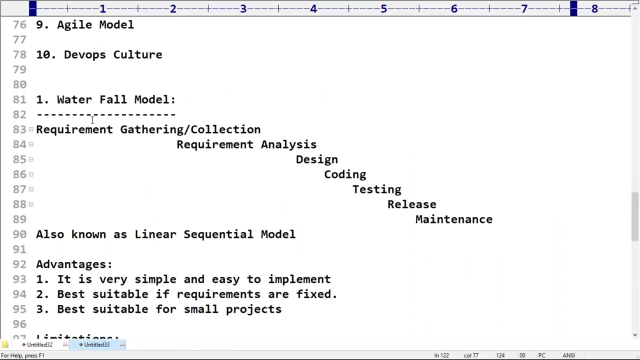 frequently used scrum, scrum model. scrum model is the most popular, most popular under frequently used model. okay, like any doubt, are you getting why this one is the most frequently used? what is the meaning of scrum? we will discuss in detail, don't worry at all. just a way, sir. so world model, oldest model. we saw the model which was almost 1950s, 1960s. we. 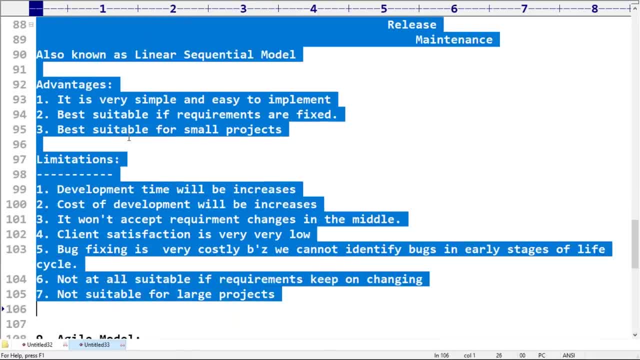 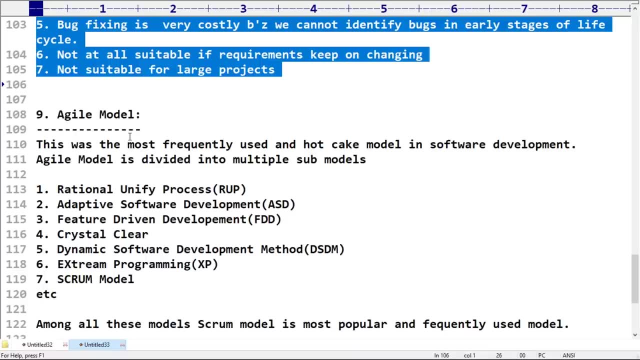 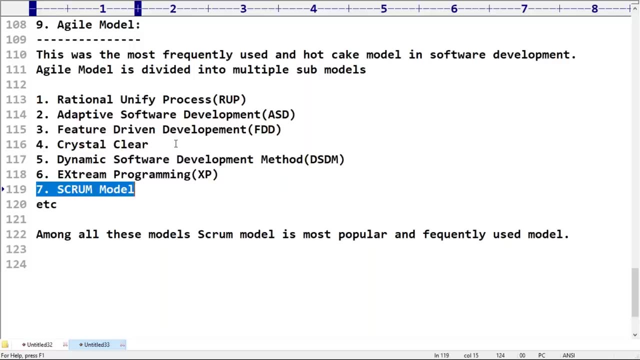 saw waterfall model. this waterfall model is the linear sequential model. linear sequential model. this is not at all required. okay, now the most recent model in the software industry to develop software says agile model. in that multiple sub models are there, in that scrum is the most popular model. okay, like now, sir, what is? 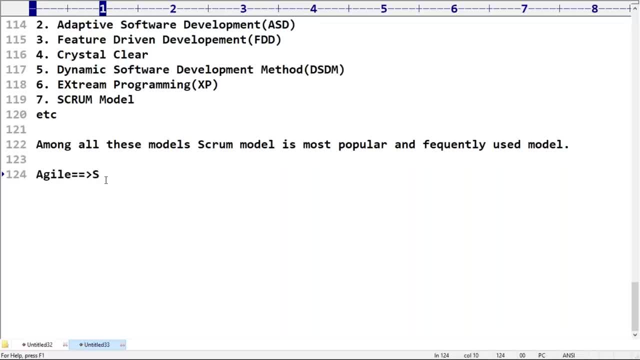 a style. what is agile? do you know? agile means speed, speed, speed. everything should be speed in that. what is a scrum? scrum, you should aware. there is one more word i want to introduce. okay, there is one more word: sprint, sprint, i want to, i want to introduce. so, total, three words are there. 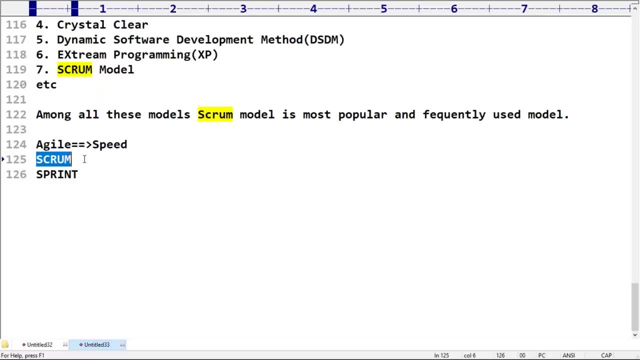 in the agile model. scrum is the sub model. scrum is a agile based model. okay, in that, sprint will be there. what is the meaning of sprint? any, any idea, any, any idea, anyone, the people who are working in the companies? okay, sprint, sprint. what is the meaning of sprint? okay, uh, remember, not sprint means not fixed. 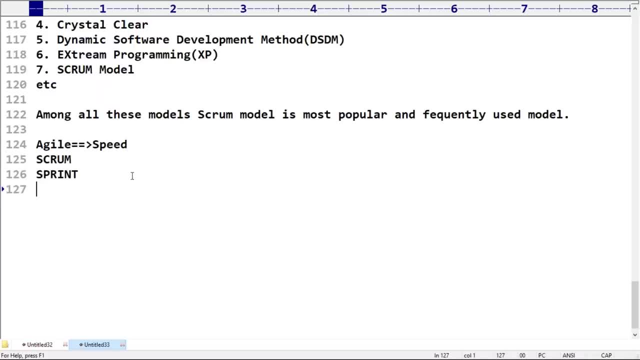 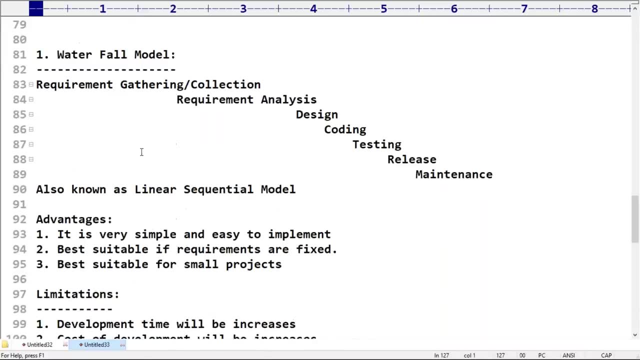 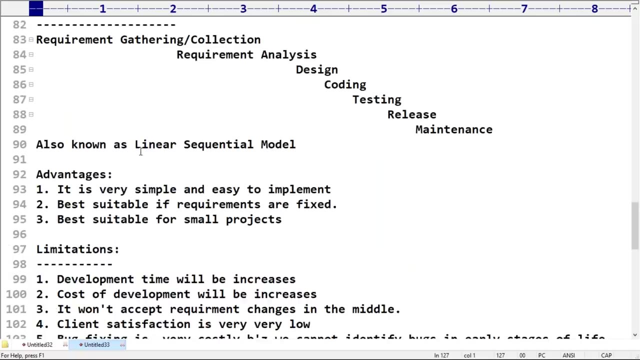 duration. don't tell uh abbreviations. yeah here, just uh. uh, take a bit very, very special care about this one, sir. waterfall model: the biggest problem is the biggest problem if you consider with the waterfall model, two important things: it is a linear sequential model. linear sequential model. 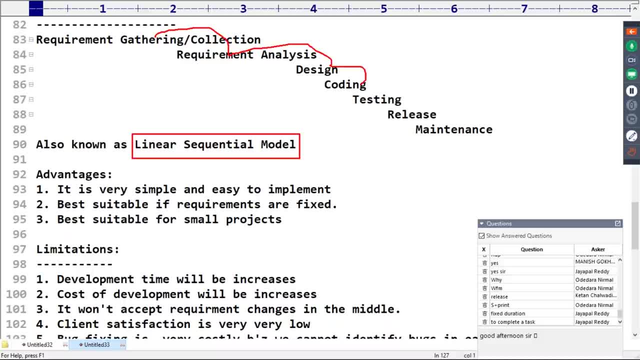 is a linear, sequential model. linear sequential model. because of that, step by step is going to be happen. because of that, development is going to be increased, just like anything. development development is going to increase like anything. next and after that, development time cost is going to increase. requirement changes won't be accepted in the middle. but but, sir, agile model, forget about. 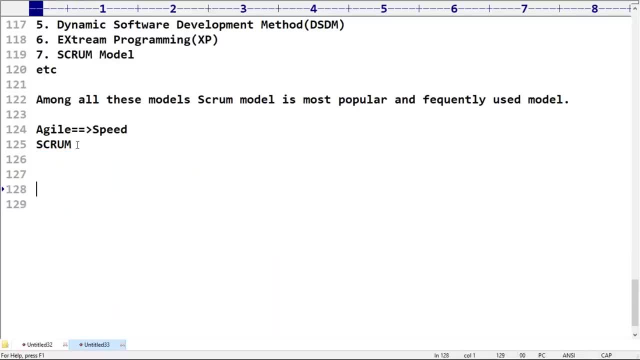 the sprint. i will, i will, i will cover in detail. next, scrum, scrum is, scrum is a agile based model. snr, c, r we can use in this yom. by the way, it is a in a binary scale. uh, let say unit model. uh, it is a single linear, sequential model. usually doesn't matter how many räätufthis has number. so 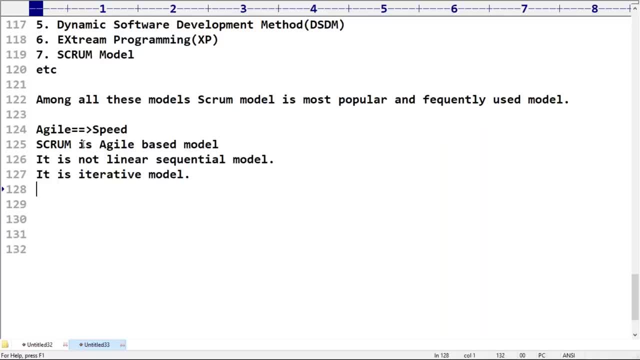 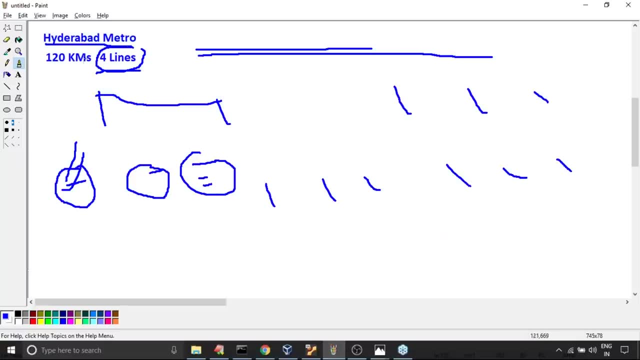 um model? what is the meaning of iterative model, sir? have you remembered three examples i covered. okay, so if you want to implement metro project for 120 kilometers of four lines, what we will do is: uh, so we won't continue for 120 kilometers at a time. okay, we will. we will convert into small, small. 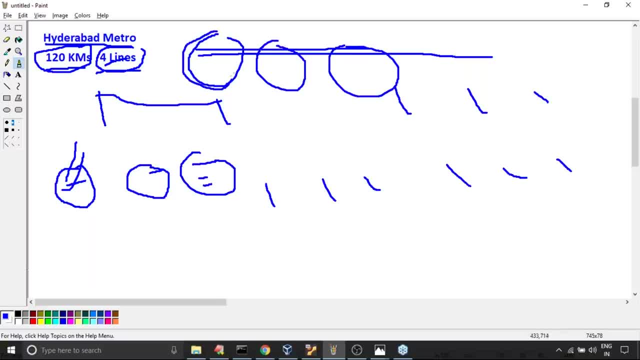 parts we will convert into small, small parts. okay, for this part, all stages are going to be developed. so, for this part, all stages are going to be developed by a set of team. a set of team, okay, like now. have you observed right now multiple small, small divisions? i want to take a total. 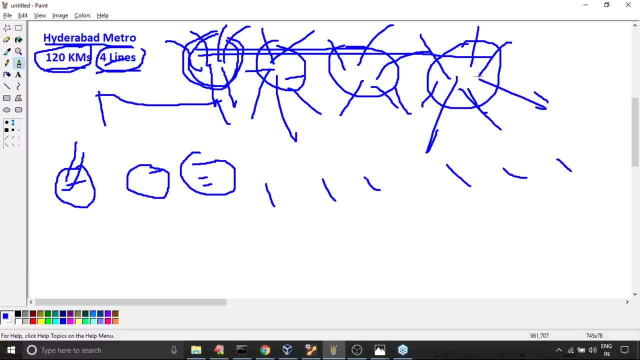 total activity i want to divide into small, small under the required team. i will, i will. i will hand over this worker for the required team. sir, for complete life cycle. for this complete life cycle, i will hand over the required team. okay, like the same way, this is small. 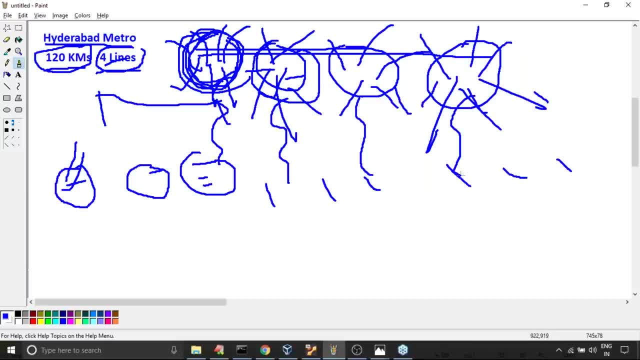 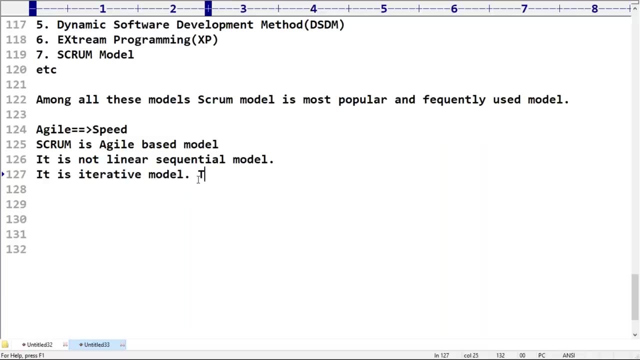 part, this small part of total software project is called a sprint. remember a bit carefully about this one. what is the word sprint? sprint means, sir. here it is an iterative model, i told right. so iterative model. now, total software, total software will be software. total software product will be, will be developed, will be developed, the total software project will be developed. 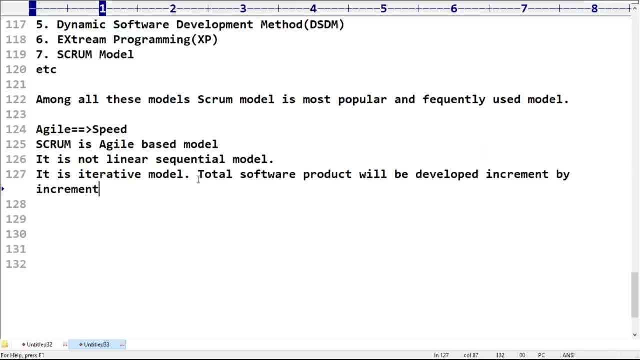 increment by increment, increment by increment, increment, increment by increment, and each increment is called a sprint. remember a bit very carefully, sir. so what is the meaning of sprint? okay, so the portion, the, the part of the individual part of the project, okay, which is by default considered as sprint. are you getting the words? i respond three things you people should aware. 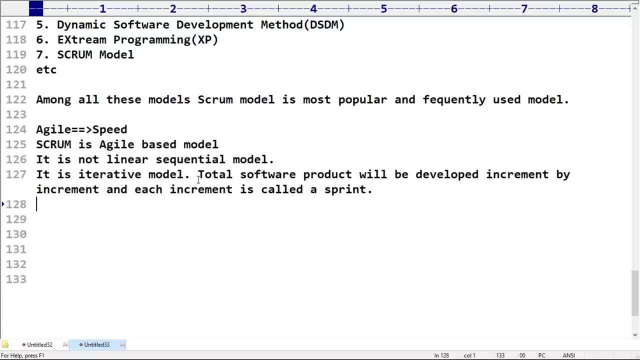 is agile, as i mean sir, as i, as i, as i mean sir, do you know, speed, speed, something like scrum is a agile based model. remember a bit carefully, right? so in the scrum, in the scrum, each individual part is by default considered as a sprint, sprint, like sir. best example, just the best, best example, example. 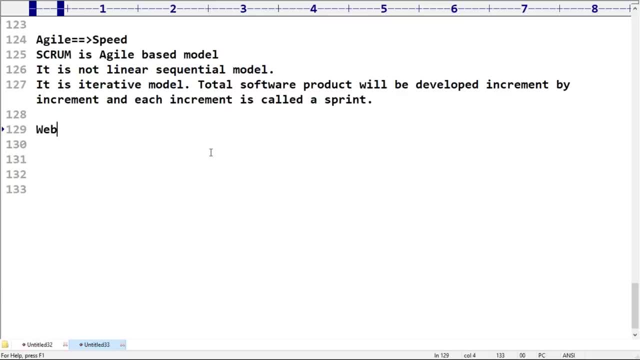 is. i want to build a website, a website, website of 100 pages. are there, sir? i want to build a website of 100 pages. what we will do is we want to build all 100 pages simultaneously. so what in the, in the waterfall model, what will happen? all 100 pages. development completed, completed. now i show to the 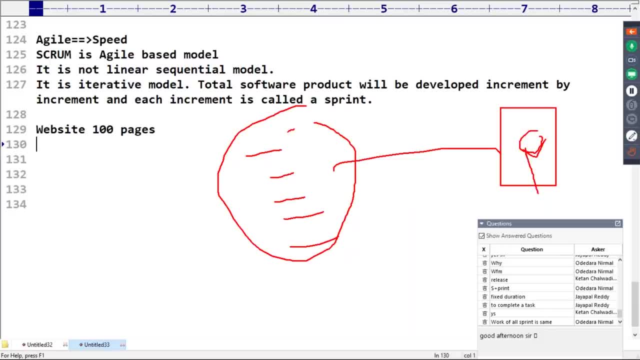 client: okay, suddenly client is asking: hey, this color is not good. can you please change the color? wow, two words are you getting? so now you have to change the color for all. you require to change the color for all hundred pages. are you getting all the hundred pages, sir? okay. 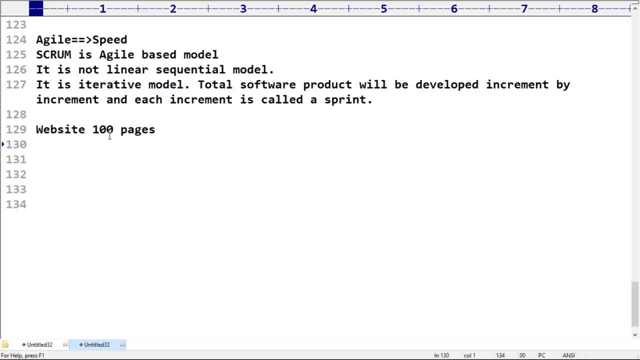 now what we will do is what we will do. so these hundred pages will be divided into around the some 10 pages, 10 pages like now. observe that, 10 pages, 10 pages, like, part by part. okay, now, these are 10 pages. first we will develop. we will develop these 10 pages in that one or two. 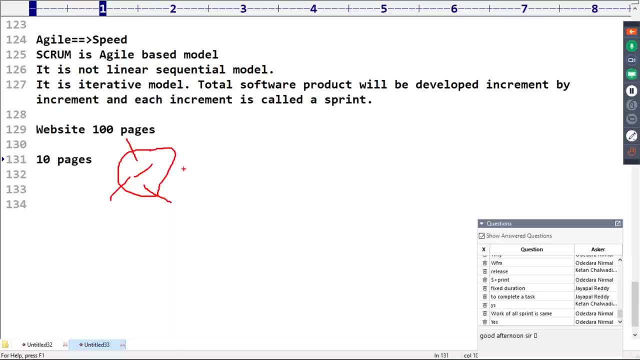 or three developers, one or two tester and ui engineer- okay, i mean ui, ui designer, front-end designer, like i will add whatever, whatever required to develop these 10 pages, almost a two, nine members are required. these seven to nine members, i will, i will assign this. this is print okay. 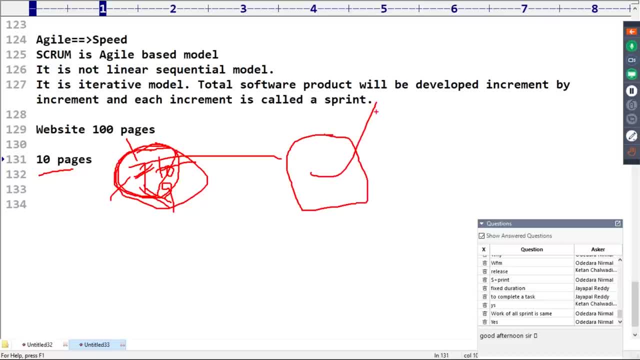 now this sprint is going to be delivered to the client. are you getting this print is going to be delivered to the client now, immediately. client is telling: sir, okay, the color is not good, can you please change the color? oh, then, immediately. so the remaining 90 pages development not yet started. now, 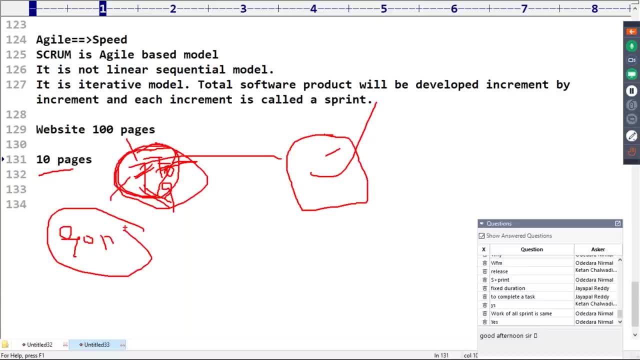 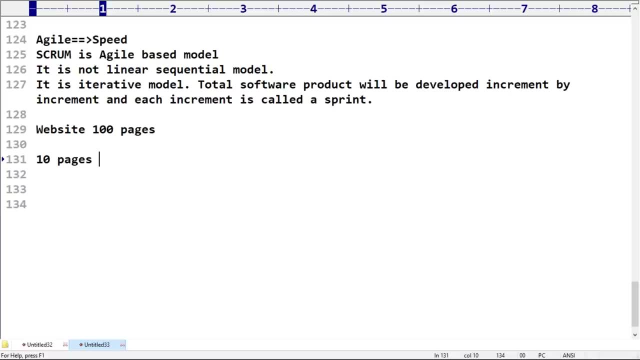 are you going to accept this change, requirement change in the middle or not? yes, friend, is it possible or not? your response: is it possible or not? yes, requirement change is going to be acceptable. next, yeah, so sprint. so do you know? in small, small pieces, continuous delivery. have you observed the? 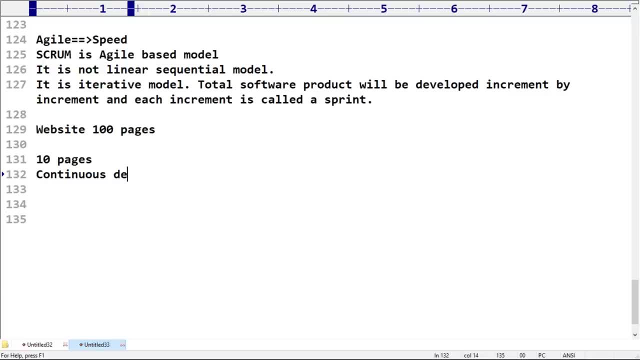 board. have you observed the board? continuous, continuous delivery. continuous delivery. you can use continuous delivery. is there? first 10 pages. we are next. remaining 10 pages in the next 20 days. remaining 10 pages next. okay, like so. continuous delivery, sir, here. continuous feedback. continuous feedback. client is always keep on giving, so which is going to accept requirement? 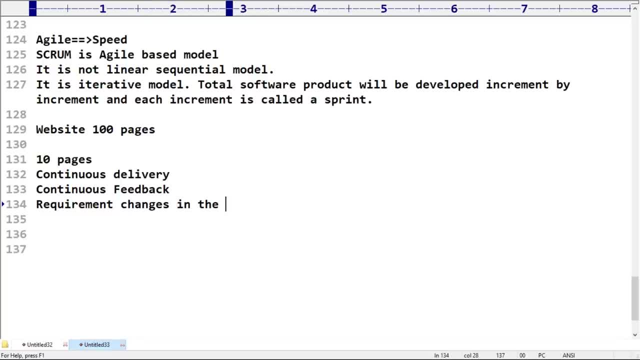 changes in the middle requirement: changes in the middle in the middle requirement changes in the middle in the middle. next, the client satisfaction claim. satisfaction is very high, i'm sure, because if he's, if he's asking any change, no problem, we are in the position to provide. 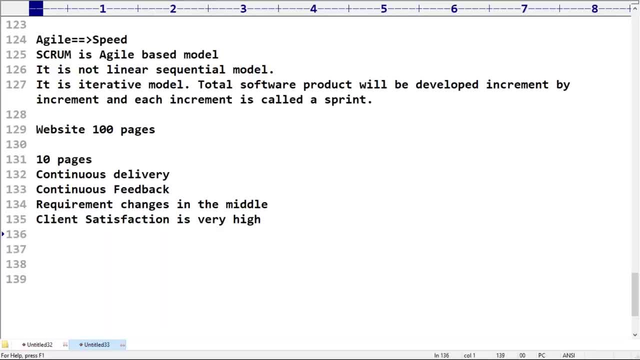 support. okay, like: do you know? continuous delivery, continuous feedback, requirement, changes in the middle. client satisfaction is very high. okay, like next, lesser development time. okay, lesser development time. what is the reason for that? yes, so in the first sprint, two to three developers, next ui engineers, ui, ui designer. 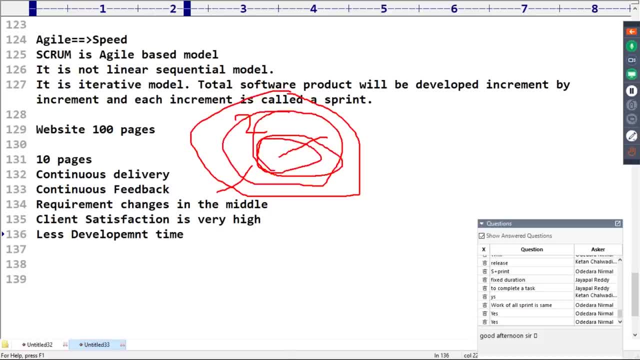 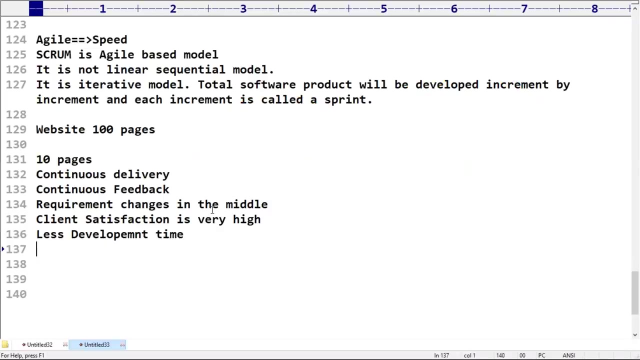 next tester. all the people are working together. all the people are working together. collaboration is there in the second sprint. uh, so all the people. two to three developers, ui, uh, ui. developer. next test engineer, like all the members, will work together simultaneously on that small piece of work. okay, that's why parallel development is possible. okay, lesser development time next. 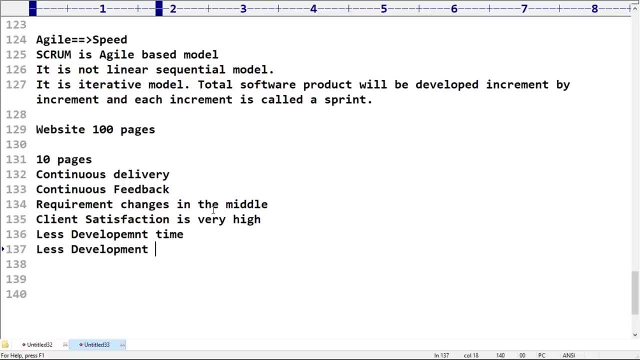 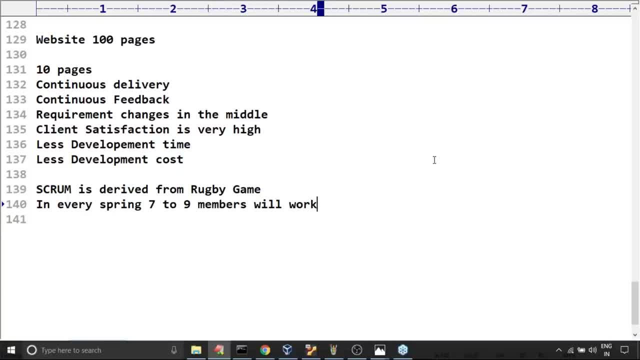 7 to 9: 9 members will work. sir. okay, sprint in every sprint. 7 to 9 members are going to work. next, each sprint, each sprint will be delivered will be will be delivered in in from one week to three weeks time. from one week to three weeks time, general words, three weeks time. remember that. 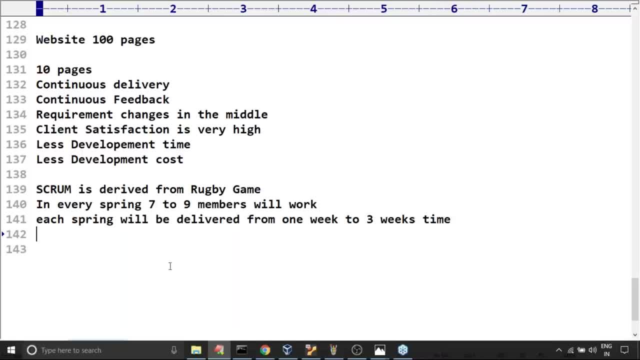 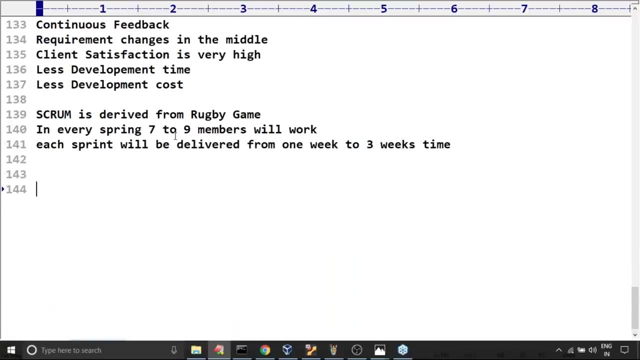 okay, like 7 to 9 members will be there each, each sprint, each sprint will be delivered. each sprint will be delivered from one week to three weeks time. okay, this is about the agile scrum model. all the people- layman's also- can understand. what is the difference between sprint- sprint? 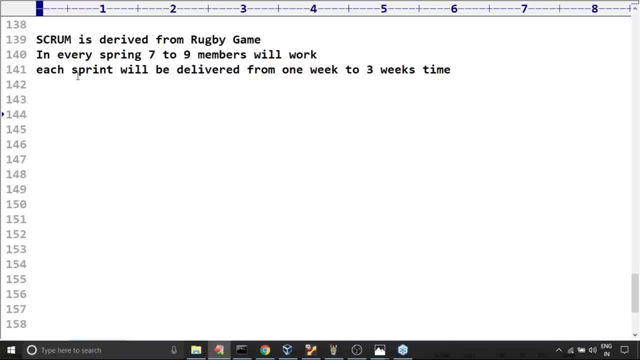 or agile scrum model and waterfall model. what is the difference, right, anyone? can you please tell? yes, friend, are you seeing the difference? waterfall model, waterfall model. okay, here, just observe very carefully: linear, sequential model, but this one is incremental model or iterative model. next, uh, next uh, waterfall model. waterfall model. requirement won't change. requirement changes won't be accepted. 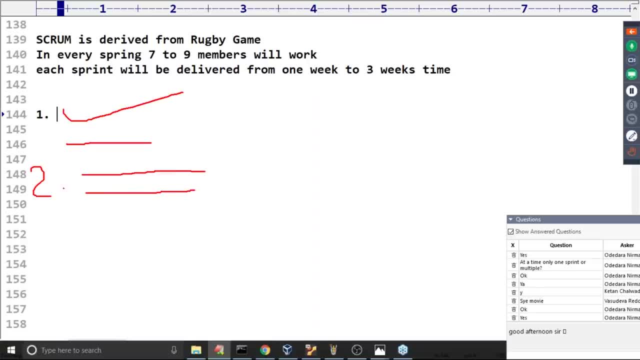 in the middle. but here's a scrum model requirement: changes are going to be accepted in the middle. next, uh, so every stage is going to be started after the previous stage, but here parallel development is always possible. okay, developers and the tester can work simultaneously together. okay, like next, and after that, development cost is, uh, less in. 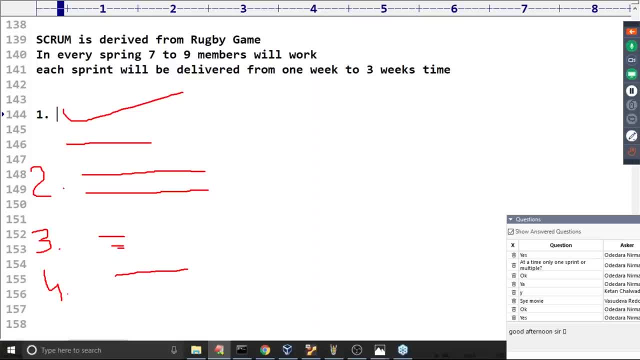 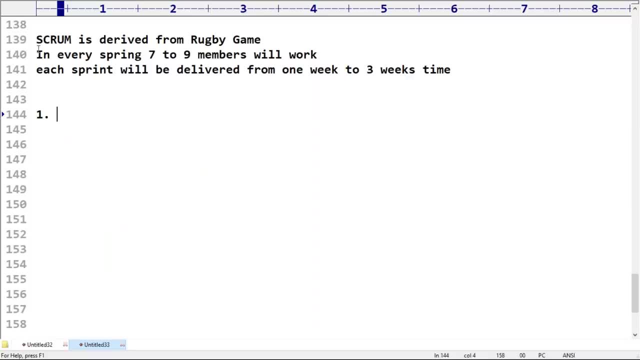 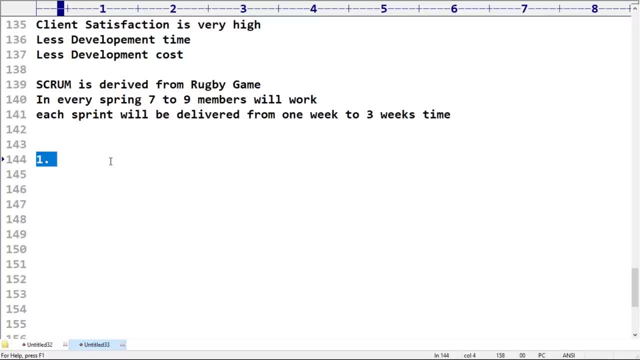 you need doubt about this. but anyway, we are not going to talk about uh, okay, sir. yeah, here normal is asking one small doubt. okay, normal doubt is: uh, sir, in one sprint. okay, sir, in one sprint all team members work of a particular members. uh, all team members means no, no, a group of members will be. 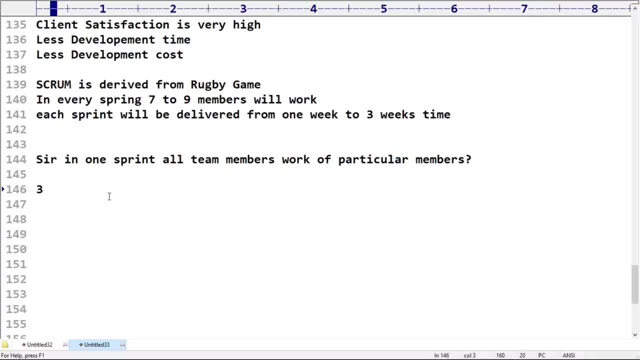 allocated. okay, from the total team: okay, three, three developers, something like three developers: one ui, ui, ui, ui, designer. okay, one ui designer next, and after that, one tester, one test engineer, one test engineer, something like that are you getting now? so almost one scrum master will be there, scrum. 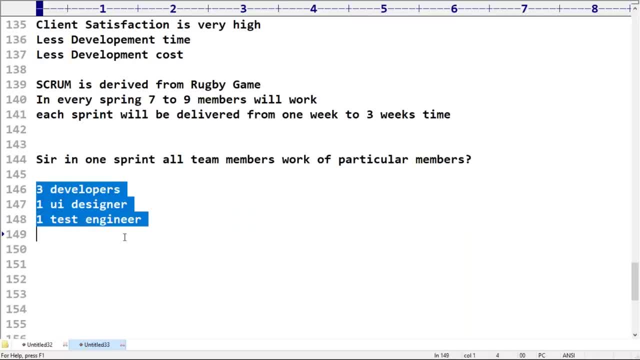 master will be there, like: okay, this is, though, these, these people, these people, uh, okay, some seven to nine members will be allocated for that particular sprint. different members will work together. okay, like next another. another three developers will be allocated for that particular. another ui designer, next another test engineer. 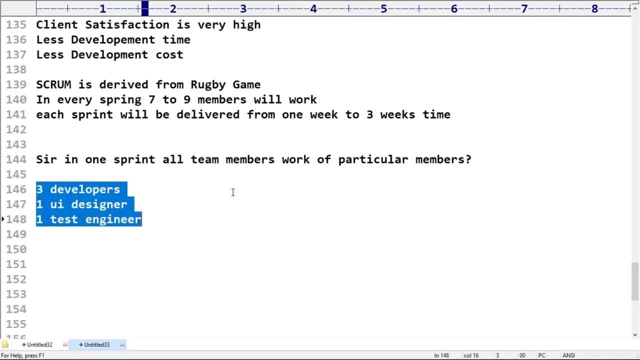 will concentrate on the second sprint. something like parallel development is possible. clear up to this. are you feeling comfortable? what is the already waterfall model? is there? okay, why this scrum model? why this is very much popular, sir, you people should have clear clarity about this one. okay, as i will, as i'll ever think, with the speed, speed. 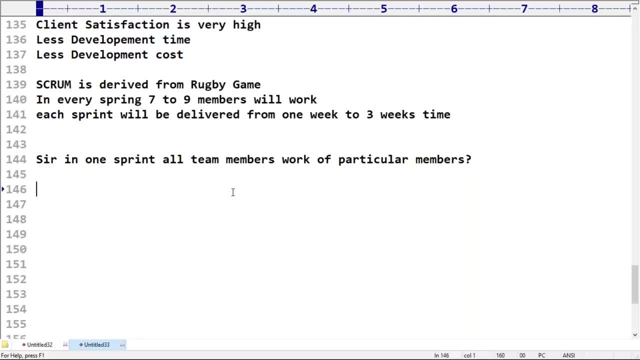 speed like now. okay, i have one big girl doubt guided out: a such a type of beautiful model is already there- why we have to go for devops model or devops culture. okay, now do you know why we have to, why we should go for devops, why, why? 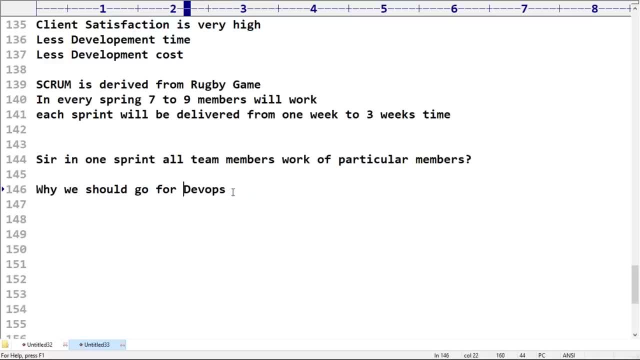 should. why should go for dev apps? okay, now take very, very special care. most of the people are going to feel. most of the people are going to feel: okay, dev apps is a nothing but agile model. dev apps is also based on the agile. okay, like most of the people are going to feel, remember that. dev apps, dev apps. 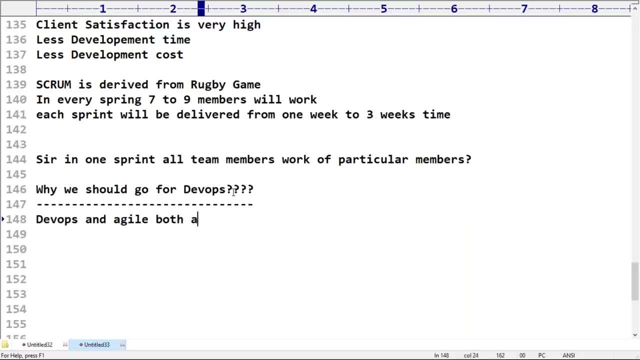 and as i'll as i'll. both are different models. first, important clarity: okay, even though there are some areas are even there are some areas are. similarity is there, but bad. okay, some areas, similarity is there, but still both are different. remember that. so similarities are there, okay. 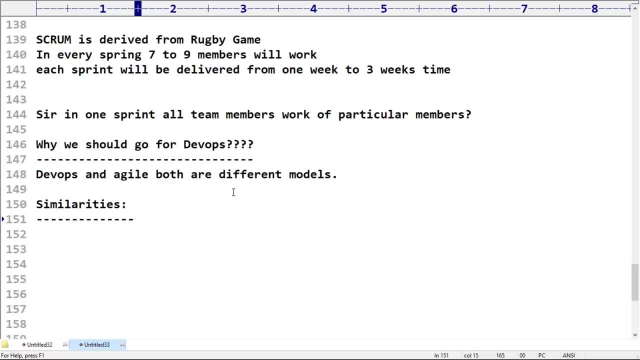 remember a bit very, very carefully, sir. which similarities are there here, right? so the first similarity: remember that both are software development methodologies. okay, both, both are software development methodologies, development methodologies. okay, like sir, i can, i can use. so what is the purpose of dev apps, sir? we are going to use, we are we are going to use for software development, right, both are. 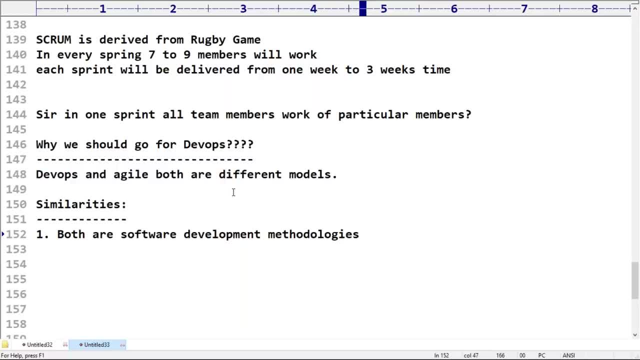 software development methodologies. okay, like one minute. one minute, sir. one is: uh, sir, this is almost for the last 20 years it is there, but dev apps is the recent, recent thing. but anyway, both are. both are software development methodologies. okay, like next. the second ones are both models. 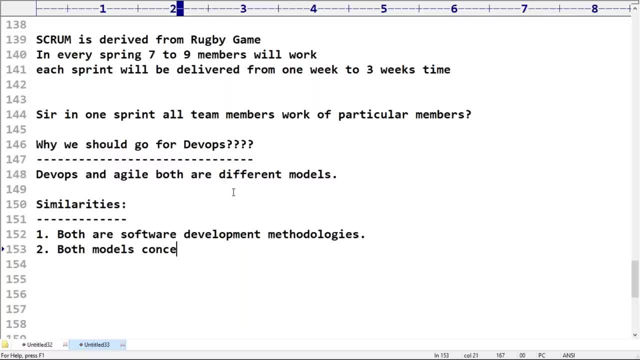 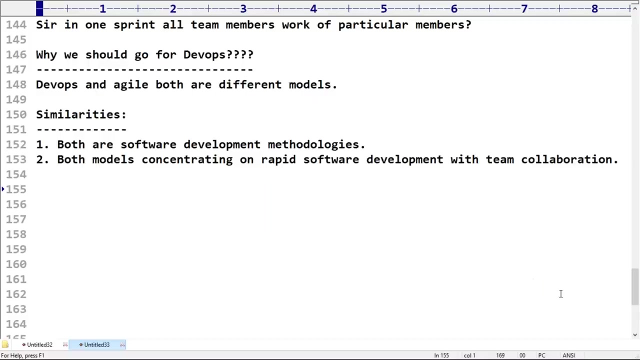 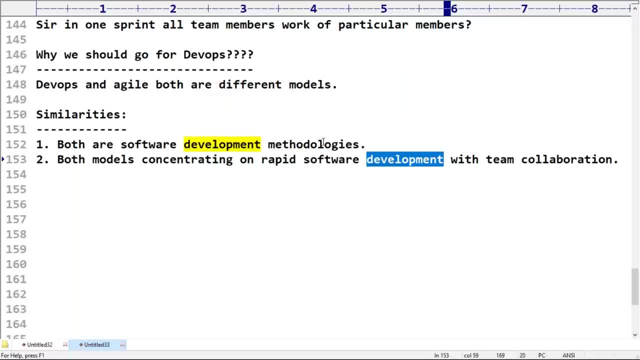 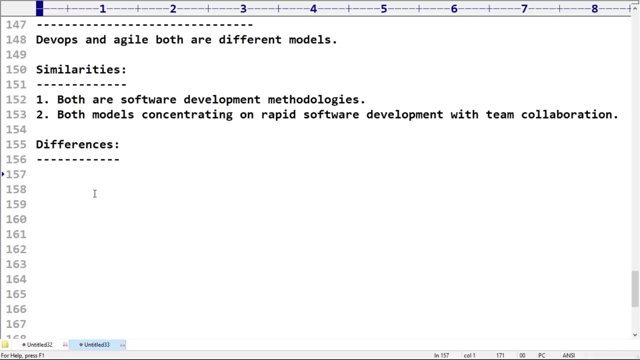 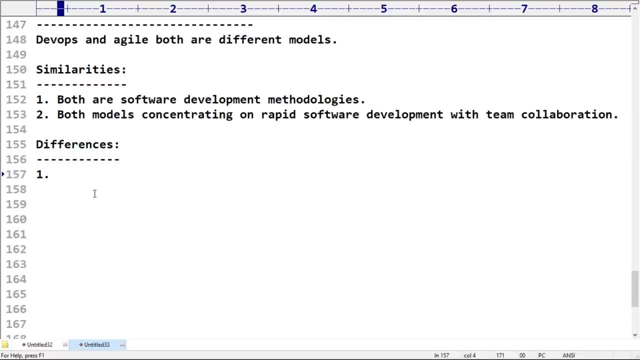 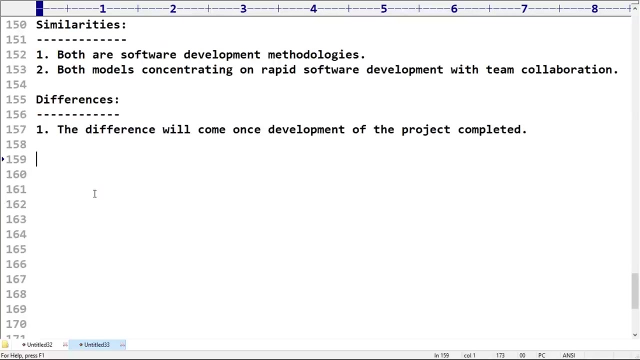 do you know? the difference between these models will start after development of the project. remember, until software development, both models are always the same. okay, the difference will come. will come once, once development of the project completed, project completed. what is the meaning of that, sir? what it means, sir? so do you know? devops talks about the development and the 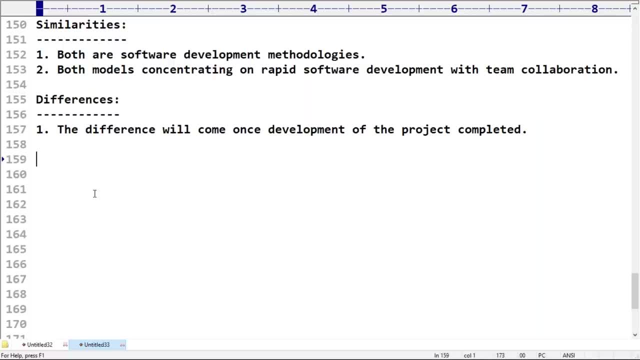 operations, correct or not. they respond: respond: development of the project, even post development, also post development also. my devops is going to talk. devops will talk post development after development. operations part also is going to be covered. but this bloody agile model talks about only development, remember they, it never talks about operations part. okay, agile model talks about: 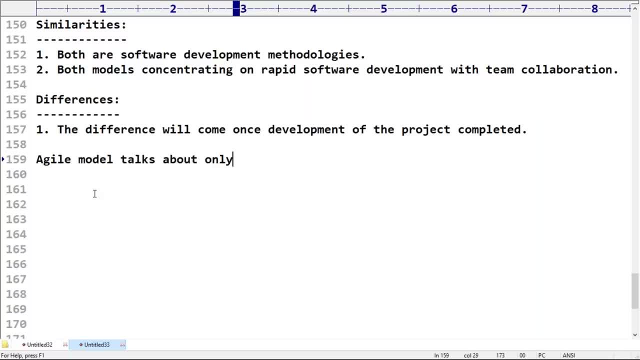 talks about only development, only development, development, but not operations, but not operations, sir, in the operation spot agile model. no, no, no, as l model is applicable only for development. but devops, devops model talks about, about the complete, complete life cycle, complete product life cycle, complete product life cycle, product life cycle life cycle. okay, like, like a development. 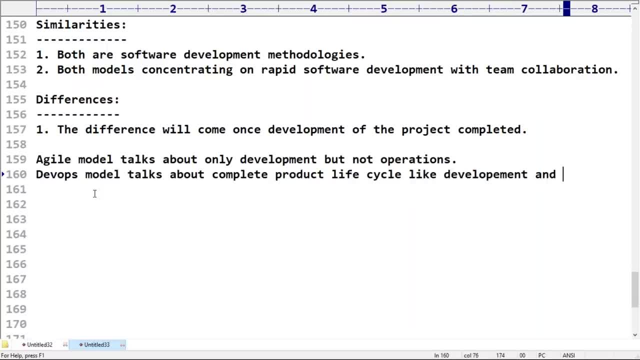 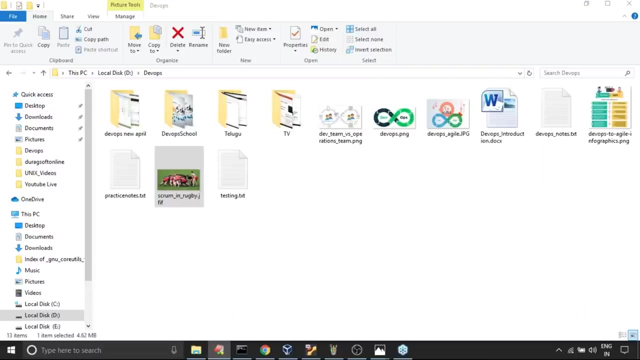 like a development and operations. development and operations. are you in the position to understand key differences are key difference between devops and the agile model is this bible only talks about development but not operations, but devops talks about development as well as operations. okay, there is one small image, is there? sir? these are not my created images, okay. 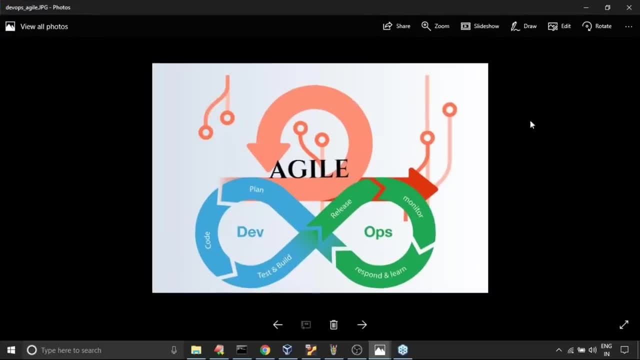 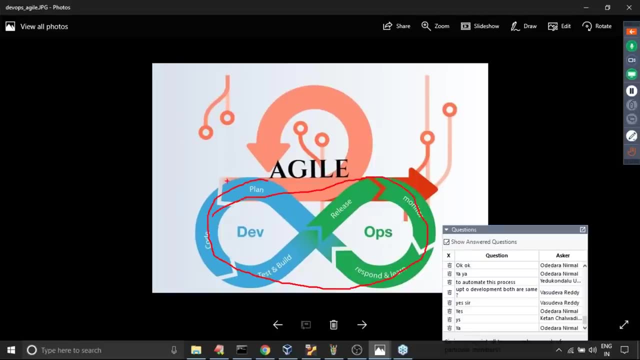 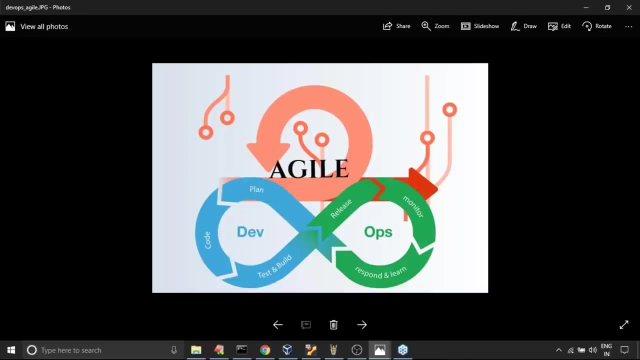 these images already there in the in google, if you want, you can able to observe that carefully. sir, here the web talks about both the things. both the things are, but this agile only talks about development. have you observed? it talks about only first part. it never talks about the second part. 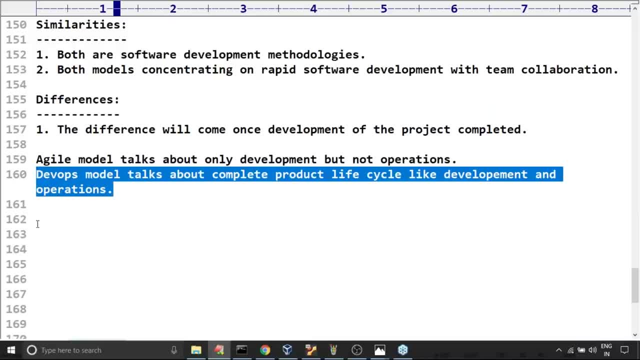 that is the one important difference. okay, like a second difference here is okay, very, very important. second difference is: in agile model, separate people are responsible for developing, testing and deploying the software. correct, right, okay, in isaiah array tester is the different different developer is the different developer. is the different ui engineer either ui ui designer. 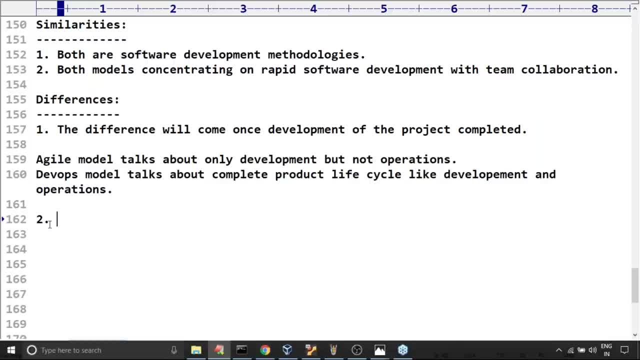 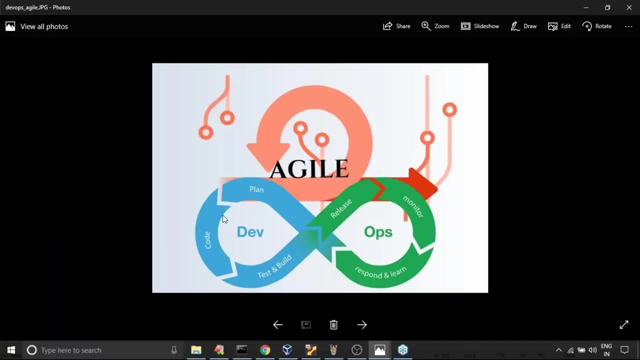 is the different, okay, deployment- deployment person is the different, okay, but in devops model, the beauty of devops is: everyone is all rounder. okay, developer is the operations operations person is the development team- okay, everyone is all rounder. remember that, even though you are specialized in the development area, sir, i'm, i'm the specializer, i'm the specializer in the. 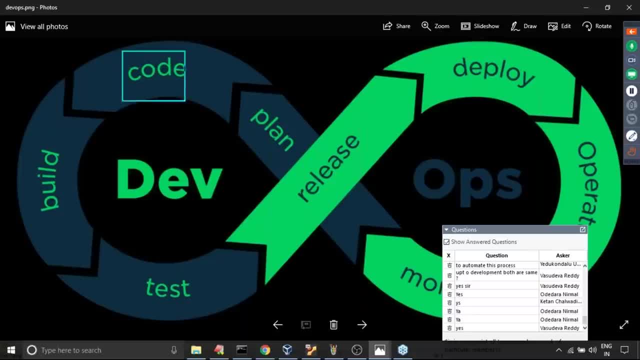 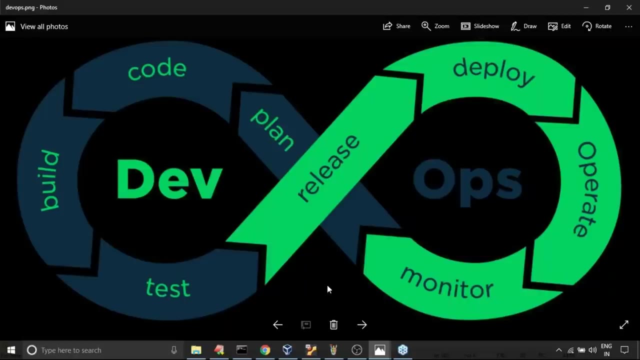 development area. assume that. so even you are specialized in the development area. but you should have- you should have, sir- complete picture on the remaining total thing. okay, total things are so individual dependency won't be there, so that's why. so the devops rule is also known as devops generalist. 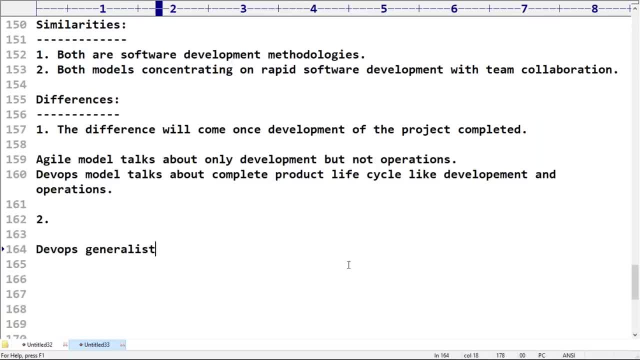 okay, generalist, generalist. what is your qualification? what is your role in the devops world? generalist means a general, in any area i can involve, in any area i can involve. so do you want? means involving software configuration management. yes, no problem at all. do you want to be involved? 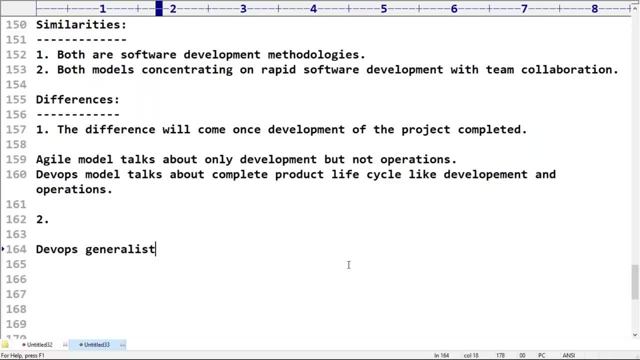 in development, no problem at all. like: so devops engineer? okay is, devops engineer is all rounder. remember a bit carefully. any doubt, friends, are you in the position to understand? okay, yeah, now observe. so the second point is the very, very important. in in as i in agile model separate. 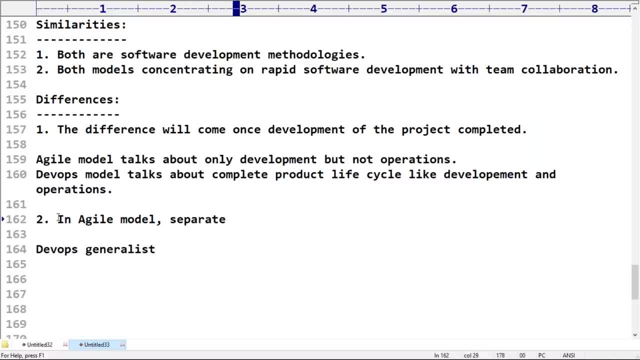 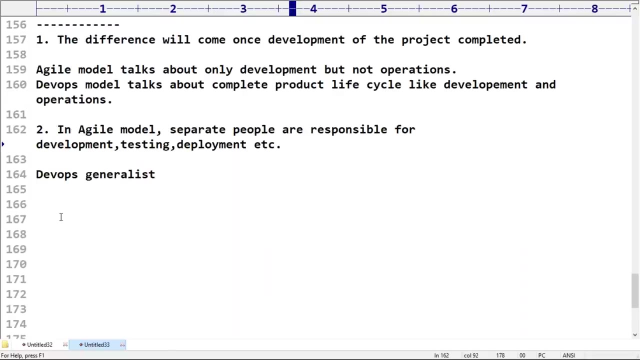 people, okay, separate, separate people. separate people are responsible, separate, separate people. people are responsible are responsible for development, for development, testing, testing, deployment, deployment, etc. okay, for every activity, sir, every person role is. the role is different. but in dev apps, but. but in devapps, but in devapps, okay, devaps. 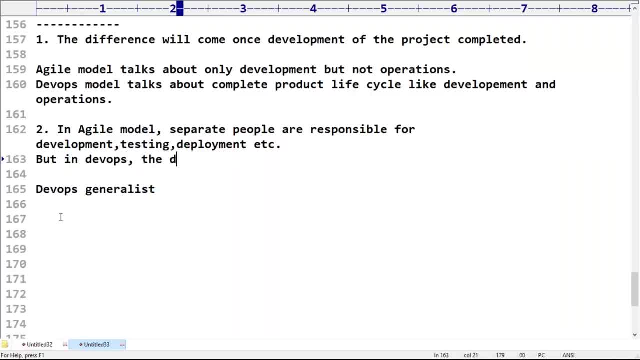 here, just observe that. but devaps, the devaps engineer is responsible. the devaps engineer engineer is responsible, responsible for everything, everything: development to operations, operations to development, everything like a development, development to development to operations, development to operations, operations and operations to development, development. like okay, that's all. so now you people may ask: 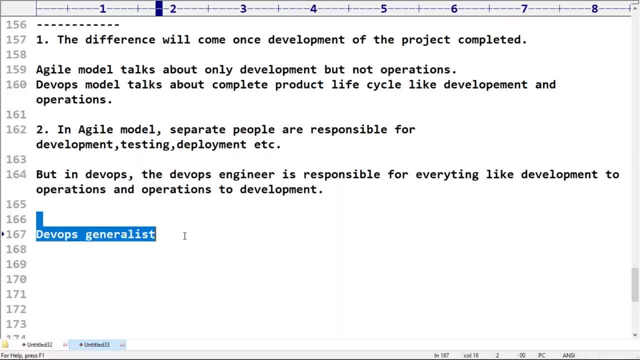 a bigger thing, sir. okay, sir, then we should have a total thing array. you are not required to worry. total, but basic idea, compulsory, you should aware. on complete process: okay, now the developer never going to talk about the release process in the earlier, but, uh, compulsory, compulsory in compulsory. 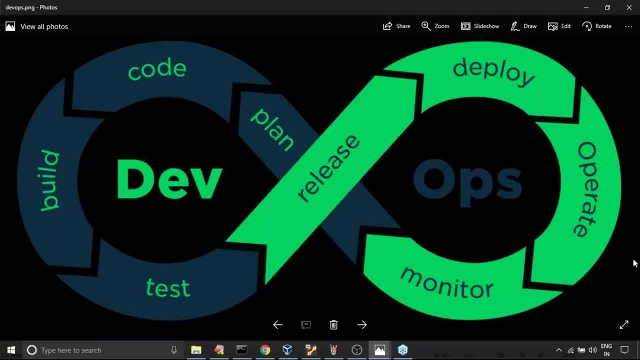 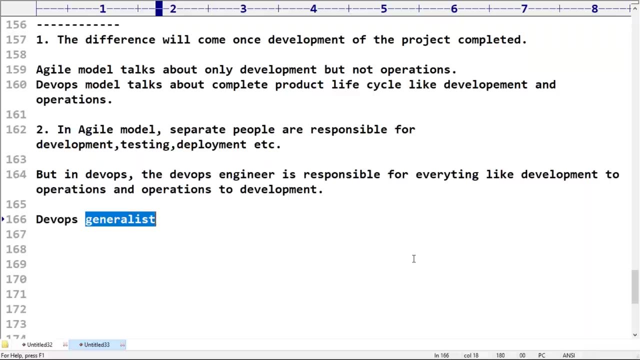 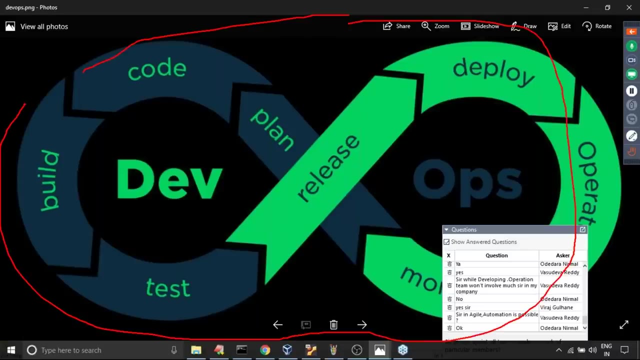 here. everything should be done, everything, everything should be, should, should have clear idea. that's why devap engineer should be the generalist. complete idea should be there on the complete process. remember, the client is always required, the source for the persons who are talking about complete picture, but not the people who are talking about only development or only 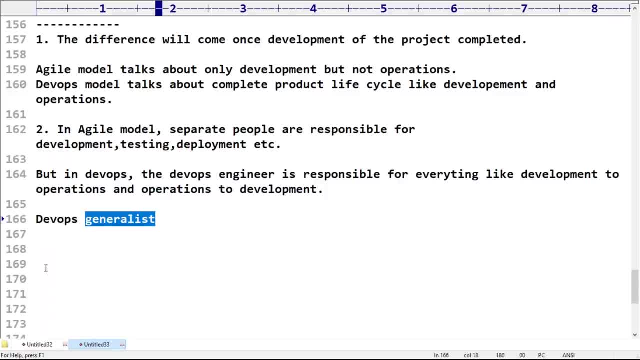 operations. that is also. so one important thing. okay, like sir, up to this, are you feeling? are you feeling comfortable? right, yes, friends, okay, next, uh, agile model. agile model won't force us, won't force us to use automation tools. are getting automation tools? that person is always talks about array, total the job, can you? 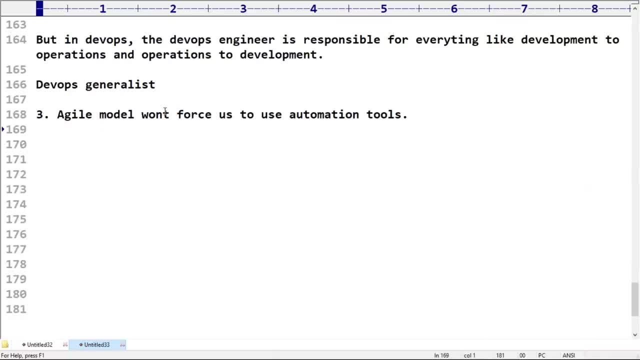 please divide, can you please divide into into small, small activities. better to do small, small activities okay, parallelly, that model is always starts, it never talks, force us to use automation tools, but but devaps, devaps, model, model is completely, is completely based on automation. okay, remember that most of the work 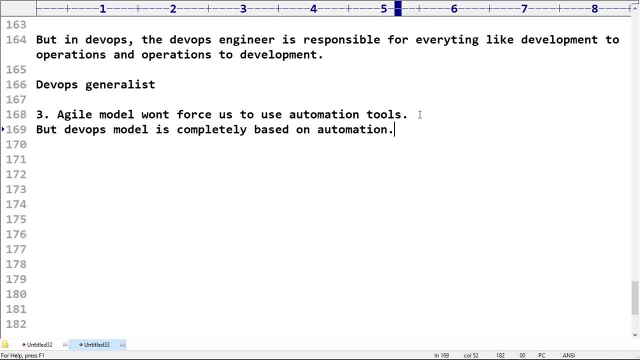 will be done automatically. we are not required to do much activity. most of the work is based on a around automation. we are not required to do much activity because of this automation. also, n number of advantages are there. okay, like so? bug fixing is a very easy. bug fixing is a very easy. 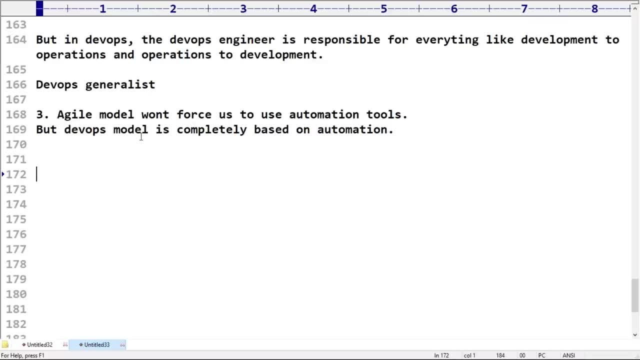 so just you know, monitoring will be there everywhere, automation tools we are going to use. that is the beauties of, that is automation is the biggest important strength on develop s. remember a bit carefully right next, sir. one more, one more. thanks so much, sir. you got it. thank you so much. 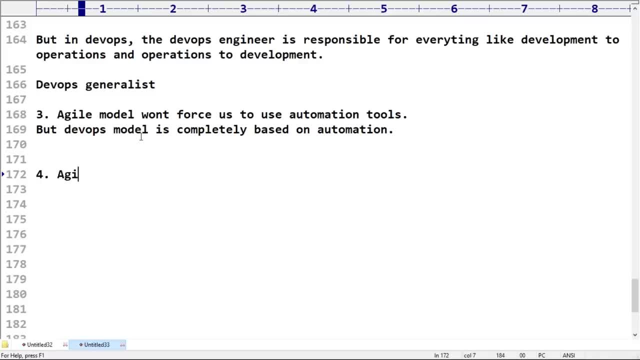 Next, sir, one more, one more difference: Agile, agile is always, always gives the importance, always giving highest priority. Agile, always, always giving highest priority, giving highest, highest priority, priority for, for highest priority for speed, because the name itself indicates: agile, agile. 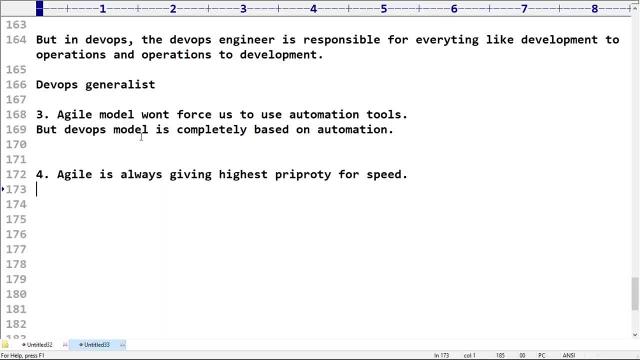 speed, speed development, rapid development, right, But but, sir, DevOps, DevOps, giving the priority, giving, giving the priority, DevOps, giving the priority. priority for both quality, quality and both quality and the speed. Remember this one: 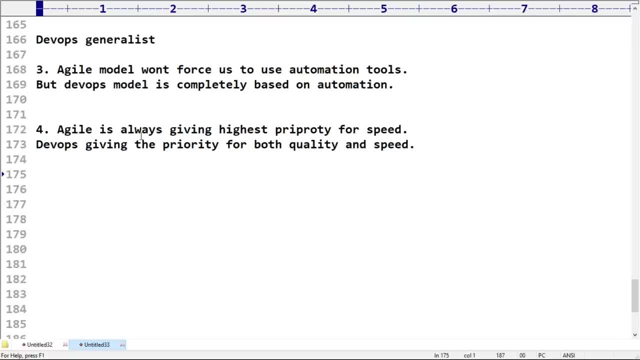 Quality is also important. Quality of the product is also important, sir. okay, Cut into pieces, pieces, and each piece you are going to develop individually may be a problem, may be a may be a problem. okay, like that. 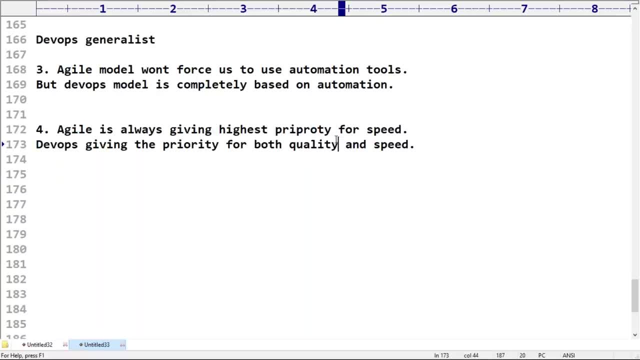 Agile. agile is always giving highest priority, only priority, only for speed, only for speed. Sometimes may compromise with the quality, but here DevOps is always talks about both quality and the speed. okay. Next thing, very, very important thing, sir, okay. 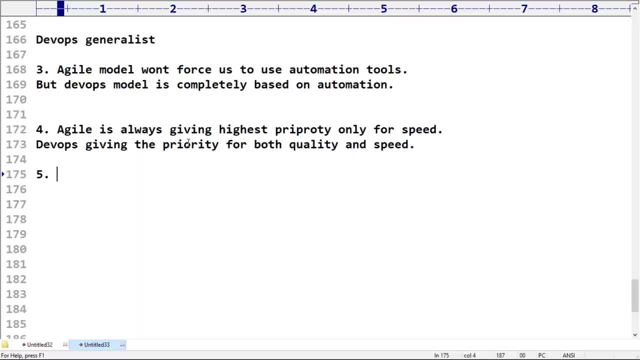 Sir, here just observe: In the agile model, when we will get the feedback from, who is the responsible to give the feedback? Respond: who is the responsible to give the feedback? in the agile model, Client is the responsible, correct? 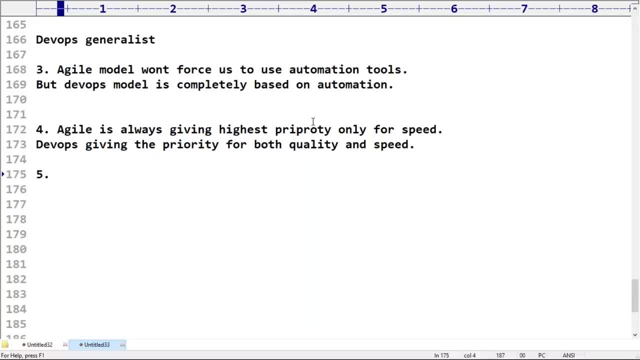 Client is the responsible after seeing the product- okay. In agile, client is the responsible to give the feedback. feedback for the sprint- okay. But but in DevOps, immediate feedback is available. In DevOps, immediate feedback is available because the total activity will be configured, will be monitored. 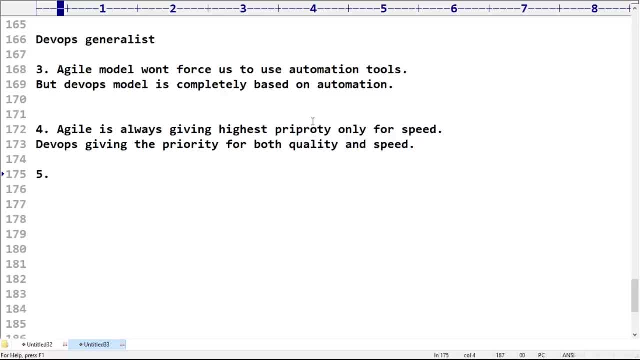 There are some monitoring. self-monitoring tools are available. Self-feedback is there. immediate feedback is there. We are not required to project it to the client and waiting for feedback. no, Immediate feedback from our monitoring tools. Remember, there are several automation tools. 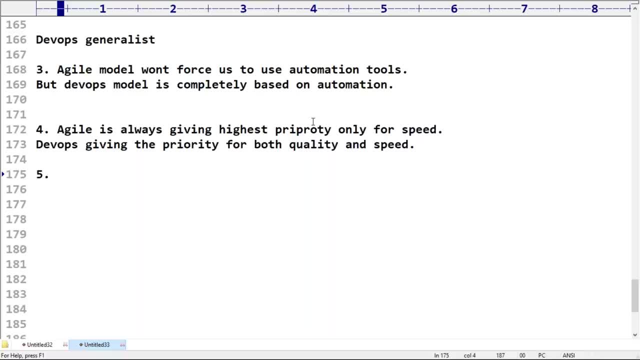 we can configure for monitoring of every stage in our DevOps. Remember that is also one important beauty. So in agile, in agile, agile, client is the responsible, client is the responsible. okay to give, to give the feedback. 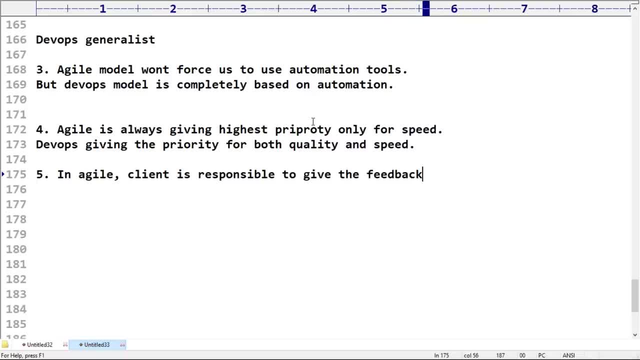 Client is the responsible to give the feedback, feedback, feedback, right. So for the sprint, for the sprint, Sprinter, like client, is the responsible to give the feedback for the Sprinter. but in DevOps, but in DevOps, but in DevOps. 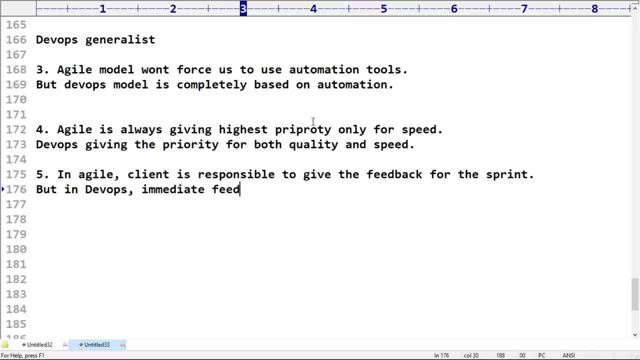 Immediate feedback, immediate feedback, but in DevOps, immediate feedback is available from the monitoring tools. Remember this one, sir- From monitoring tools. okay, Ended Ended monitoring tools. okay, like that's what you should have been. are you in the position to? 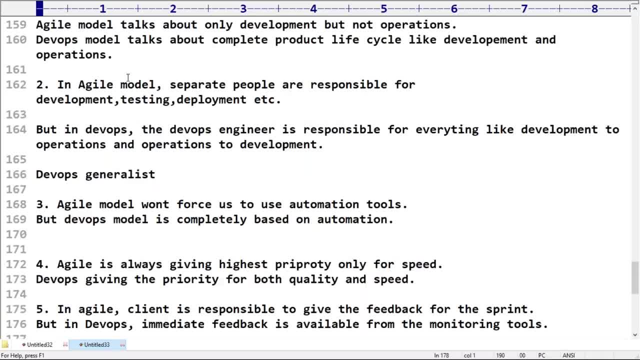 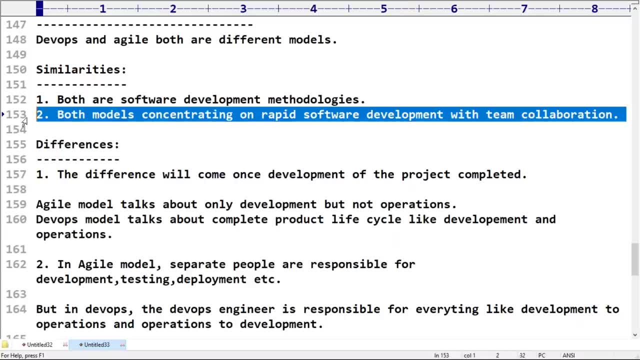 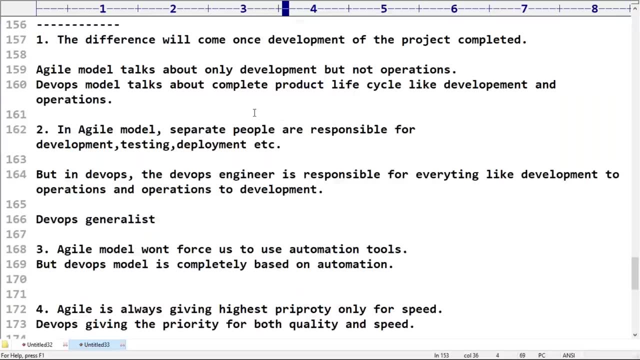 understand now with this, sir. have you observed, right? okay, multiple differences are there, friends? just only collaboration, team collaboration and rapid software development by seeing these two things hurry. devops is the asl based model. no, array. asl based model is the different devops. model is the different. devops is always talks about automation. devops is always talk. 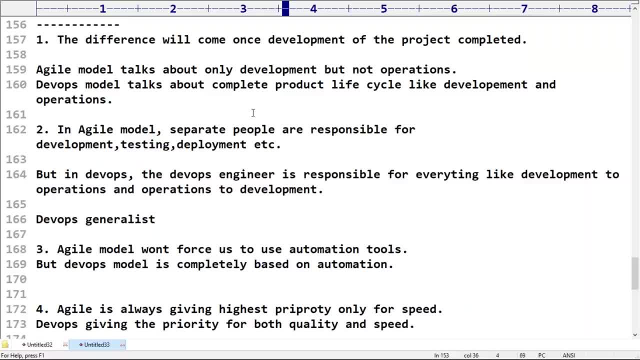 about. okay, like, yes, edu, gondola, sdls, until development. both the things are same, but this one is going to talk about the next level things also next in the sdlc also. okay, sdlc also, there is a. there is a difference these person is always going to impose everywhere. 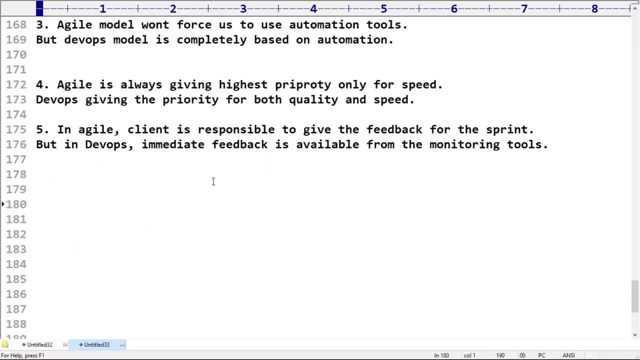 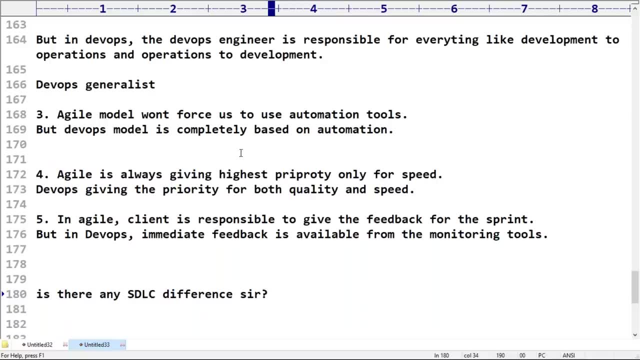 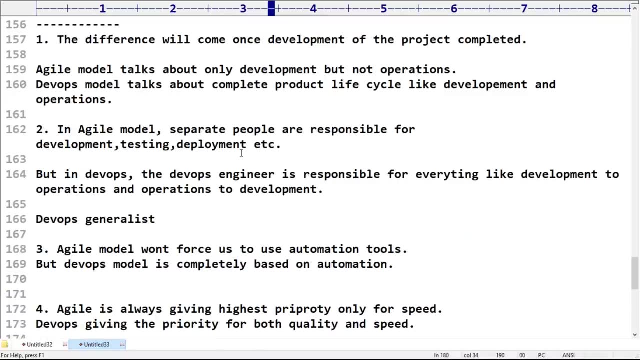 automation tools. yes, edu gondola is asking something in sdlc. is there any difference? yes, this person is always talks about everywhere: automation tool is the mandatory, but their automation tools are not mandatory. technically, any disadvantage automation apart from losing jobs. was there already no chance at all? that is the training we require to do monitoring tools- normal, normal monitoring. 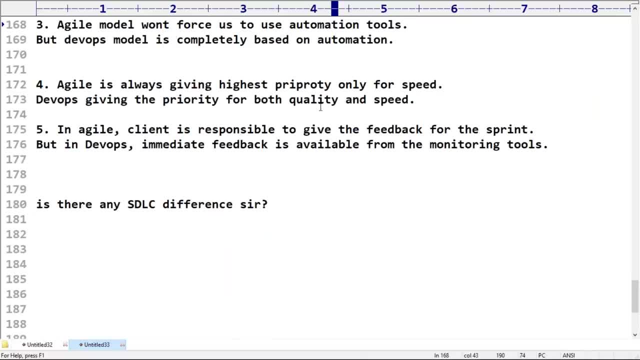 monitoring tools means if your server, my server, is there, my application is running. keep on running, sir, keep on running. provide the service. by mistake, by mistake, my application is down. may be some problem in the server? okay, hey, okay, so i have to check manually whether my application is running or not. instead, 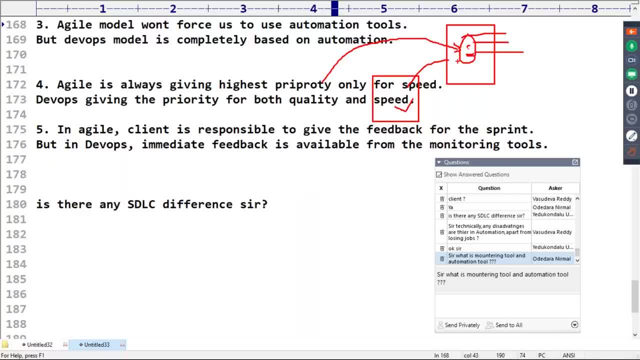 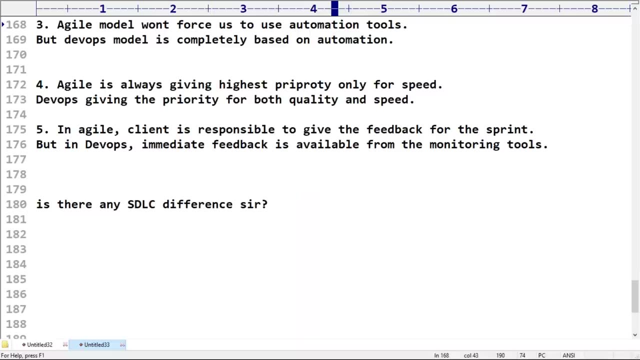 of that, i will configure one automation tool immediately. once this application is down, immediately this monetary tool is going to rise, the alert saying boss, there is so on. so application is not running for the last five minutes onwards. please check, collect immediately. a lot is going to be riser by monitoring tools. okay, we can configure monitoring. 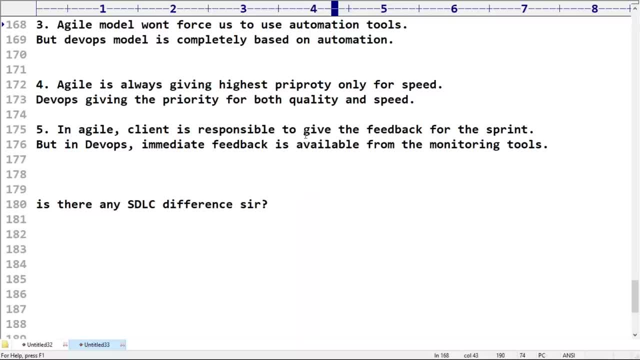 monitoring tools. okay, like next. automation tool means, sir, which is going to be performing automatically? monitoring tool is also automation tool, only we are not required to operate automatically. it's going to do that. okay, clear. so if any person is asking what is the difference between devaps and agile, are you in the position to understand? yes, friends, everyone in the position. 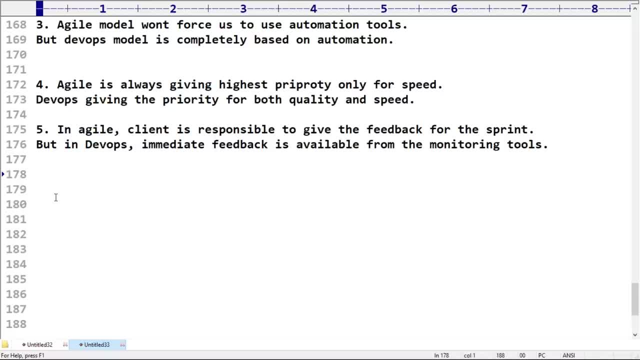 to understand everyone in the position to give left and right to that person. yes, these are various things you should avoid. so in the olden days, one worst model we have waterfall model. next level, the most hot cake model, asl model. okay, now the people are always talks about dev apps. 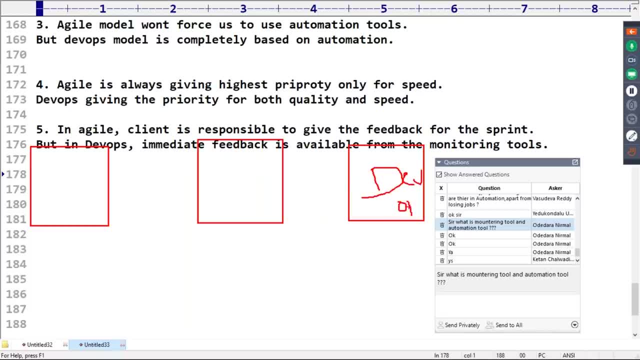 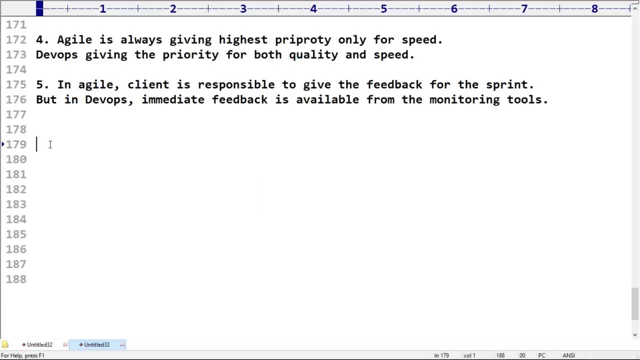 okay, this is the future trend as of now. okay, dev apps, dev apps. the biggest specialty of dev apps is end to end, end to end completing. it's going to talk both development and operations. end to end- complete thing is always going to talk. remember very carefully about that. 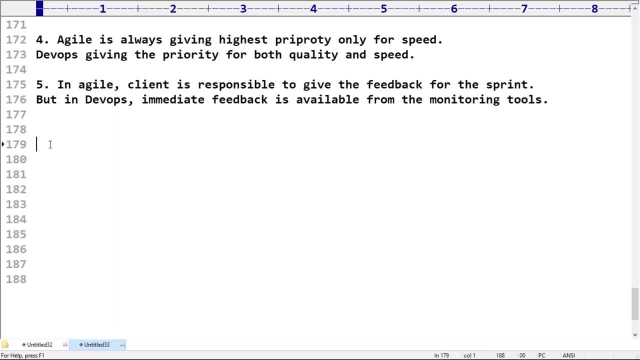 okay. next, the biggest specialty: automation everywhere. automation. we are not required to do anything. automation. automation tools by default will be there. continuous monitoring by default will be there. continuous feedback is their biggest asset to the devops model. right, okay, now can you please from this portal discussion? okay, what is the dev apps? okay, can you please confirm again? 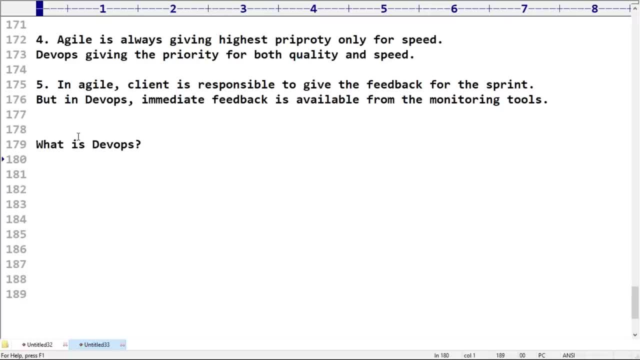 is it a new tool or is it a new technology in the market? i respond: is it a new tool? is it a new technology in the market? no, it is. it is a new. it is a new, a new culture. it is a new culture or process we have. 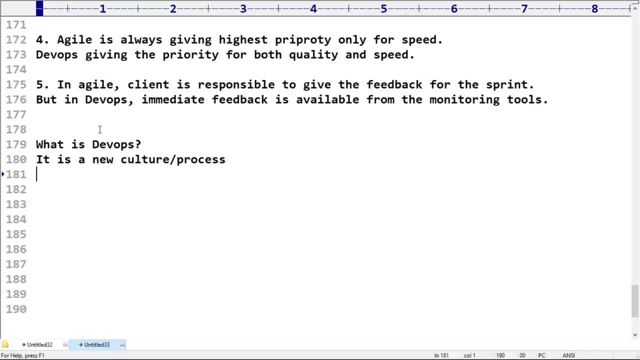 to follow for software development and operations. okay, devops, talks about both the development and operations, is a combination of development and operations. it is the process of, it is the process, process of, process of continuous. it is the. it is the process of continuous development. okay, continuous development, continuous build, continuous, build, build. okay, like we can use the word, it is. 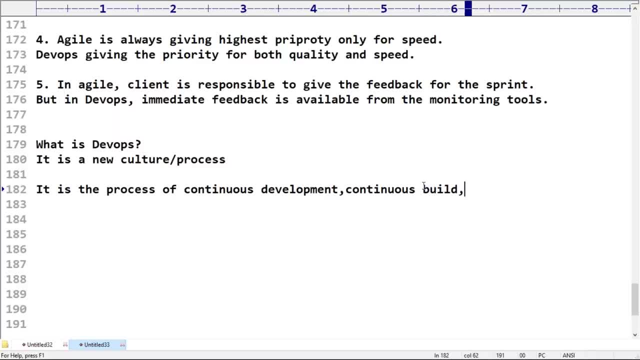 a continuous development. continuous build: okay, it is, it is not going to be stopped, sir. continuous build, it is, it is not going to be stopped, sir. continuous test: okay, continuous test. continuous release, continuous, continuous release. release like a release of the software- okay, continuous. everything is always continuous. it is a culture: okay, what is the meaning of continuous integration? continuous. 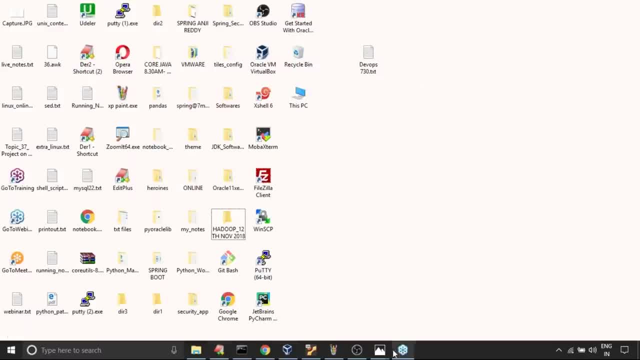 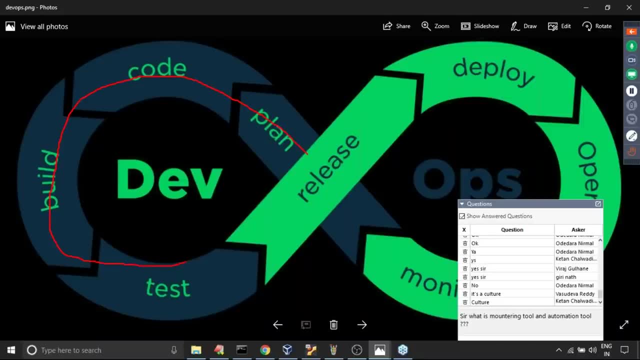 delivery like this part i will discuss. sorry, have you observed? if you observe the logo of the devops, okay, it is, it is a continuous process. have you observed? right, it is the. it is, it is a continuous process. the beauty- have a look. one side with the continuous process. 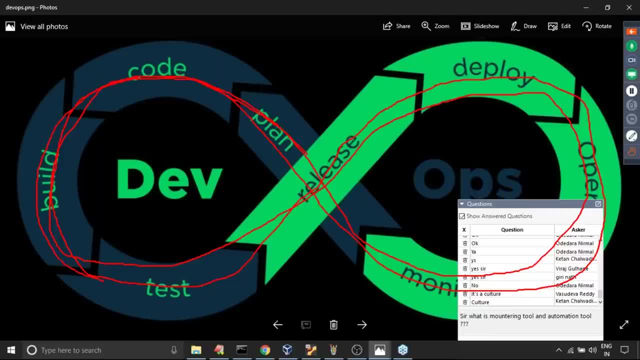 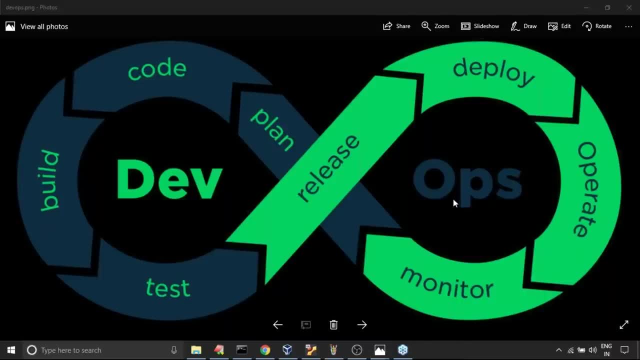 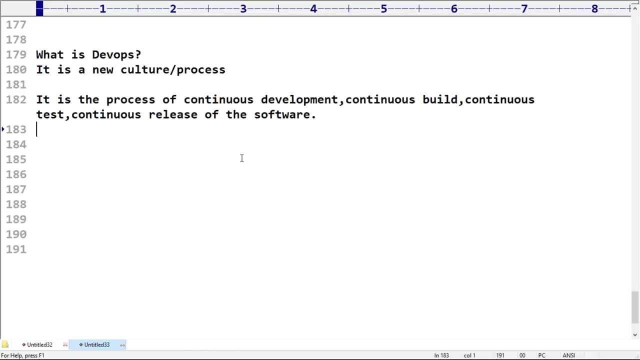 infinity. it is never going to be stopped. okay, for every new chain, if this model, this cycle is going to provide the support, okay, this culture is a highly recommended okay to follow. this is the next level trend in the software industry. clear, are you getting the basic introduction? 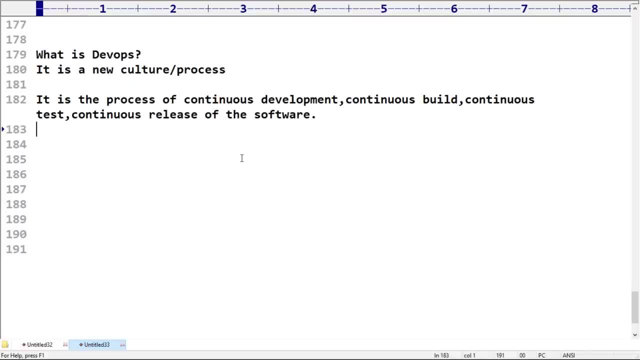 why devops, devops versus agile devops versus waterfall model? okay, what this new culture like, but anyway, technical words i didn't use sir. what is the? what are various automation tools? are there? okay, automation, automation, devops, tools. which tools? which tools are there? i didn't use these. 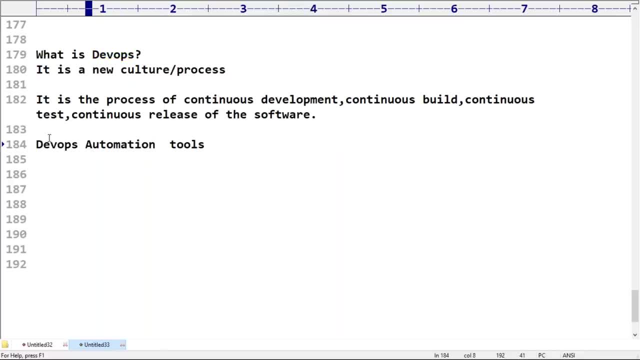 words. maybe in the next session i will talk about which tools we are going to use, for which purpose of these tools, which are very popular tools. okay, like, we will discuss and then. so each tool, one by one, one by one, we have to perform post-mortem. okay with the integration. 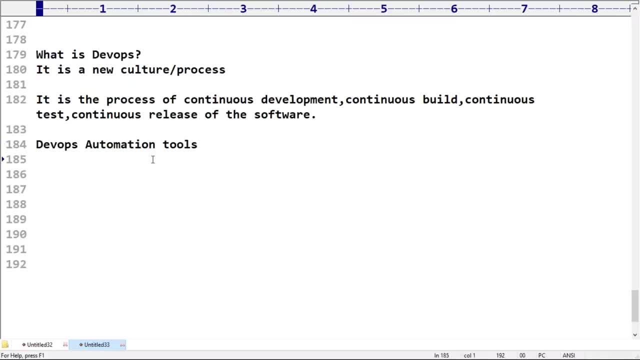 things. that's what you people should aware about the dev apps. yeah, how is defined dev apps, water flow, etc. any organization? yeah, how is defined dev apps, water flow, etc. any organization? what is the meaning? what is the meaning of that? most currently, most of the people are always going to waterfall already gone. 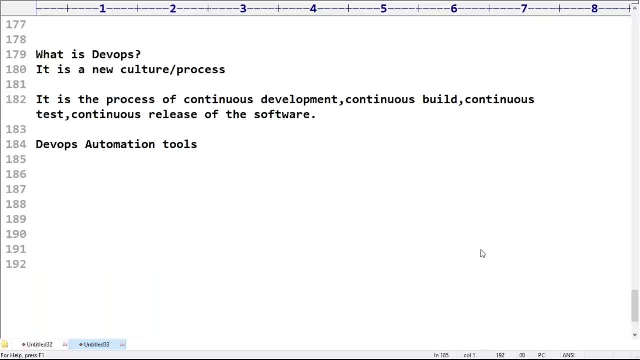 whatever, who is going to? who is going to decide? who is going to decide? so, mostly the client came up with the requirements. software company people are responsible, so to provide guidelines or the client side it team will be there. they are going to impose. can you please implement? based on devap. 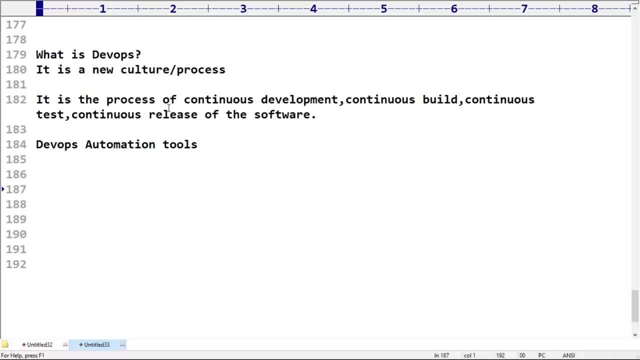 model like: so client side id experts will be there. if the client is the small client client or otherwise, okay, small scale client- then the software company itself is going to tell these are the possibilities, like okay, like yeah, next, uh, uh was already. is asking one small doubt. okay, his doubt is, sir, even after? 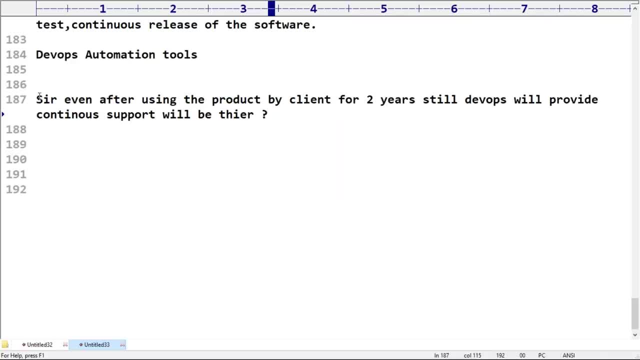 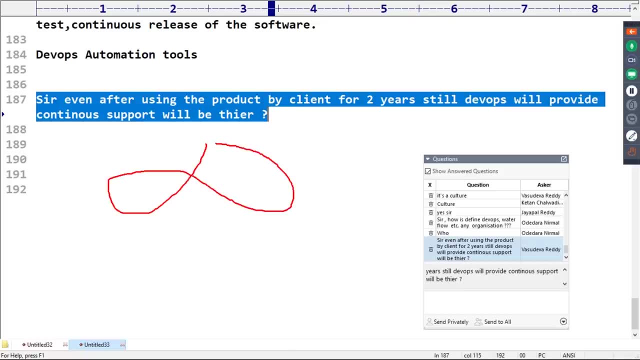 using the product by client for two years still. devops will provide continuous support, will be there. yes, that's what. that is the beauty. my devops cycle, my devops cycle. once my cycle is going to start, where it is going to end, have you observed right, is it going? 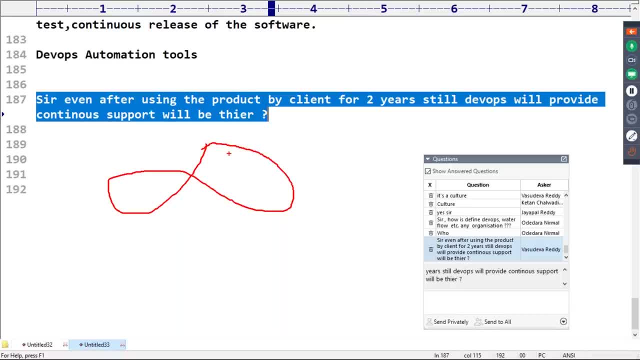 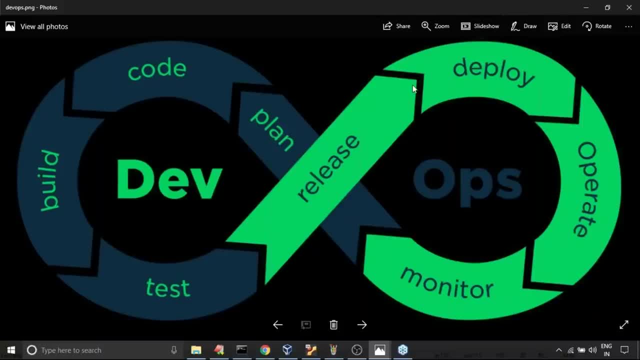 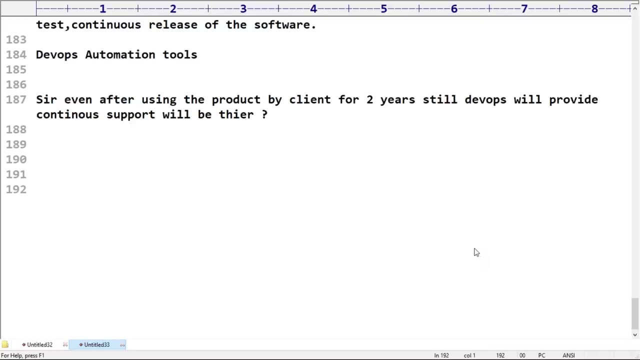 to end anywhere. this is the devops cycle. is it going to end anywhere? are you seeing anywhere end point of my devops? it is infinite, loop, loop, forever. this loop is going to execute. that's why, beautifully, the design logo, okay, good. so what is the difference between astosh, what is the difference between scrum and devaps? 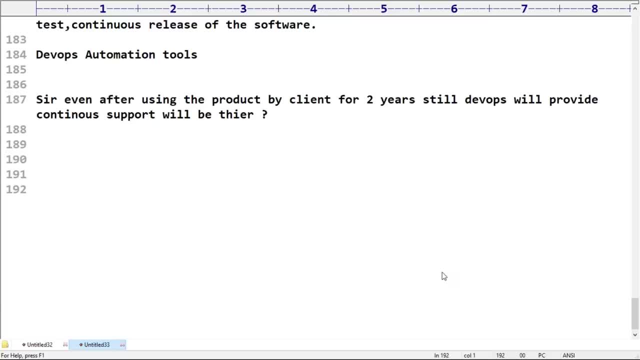 now you should not ask this question, sir. what is the difference between scrum, scrum under devaps? you should not ask this question just because we covered almost multiple, multiple things. just to go through the video. okay, yeah, sir, for devaps, general, generalist role, what development technology that is the generalist? 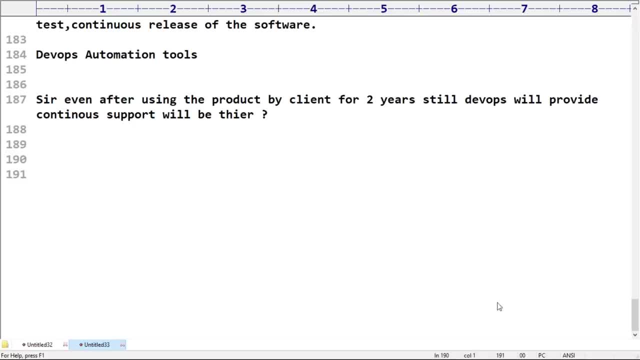 role. yeah, that's what. okay, so here for dev apps, for dev apps, generalist role. what development technology we have to give air? that is our next, the cinema. okay, which technologies you have to, which tools you have to adapt to tell your role is dev apps generalist, so almost.